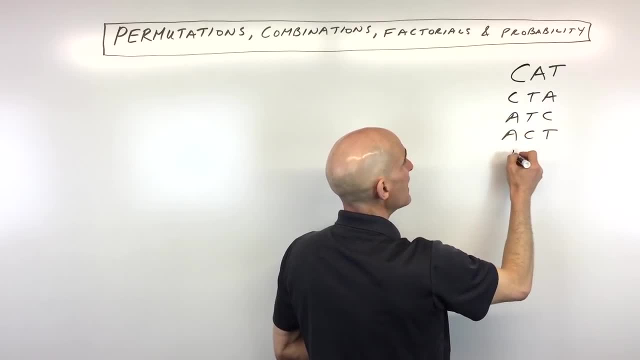 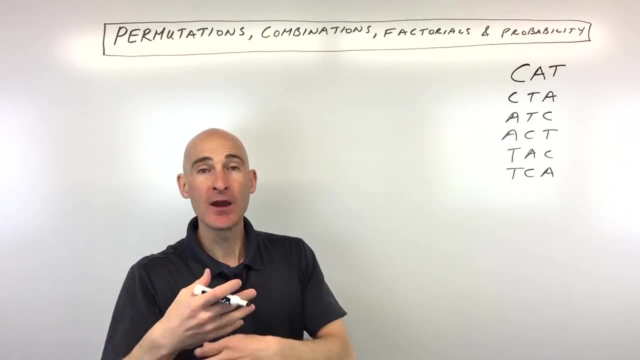 A-T-C, A-C-T, T-A-C and T-C-A. So you can see there's actually six different ways of writing this word, using all three letters in the word cat. So there's six permutations or orderings Now. 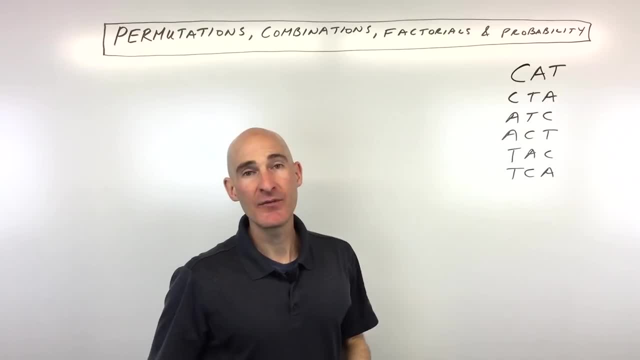 there's another way to do this. When you're taking three items and you're wanting to see how many different ways you can order them, you can use this formula here, which is N- factorial. Now the way the factorial works is: you start at this number here. In this case, we're working. 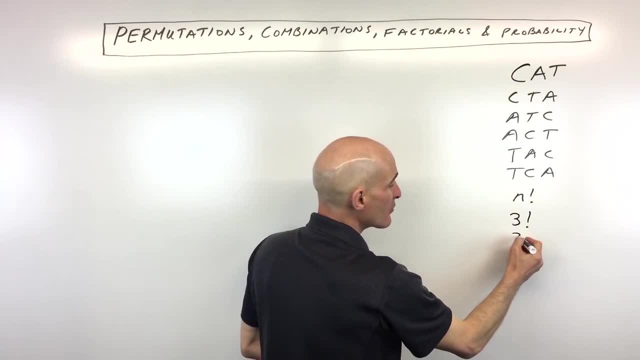 with three letters. That's going to be three factorial, And you take that number three and you multiply down to one. So this is going to be equal to six, three times two times one, And you can see there was six different permutations or orderings. Now, another way to look at this is: 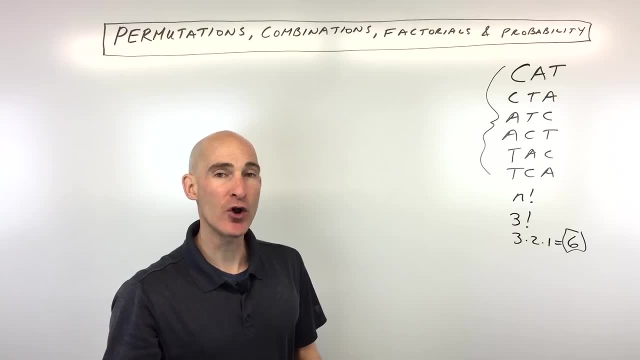 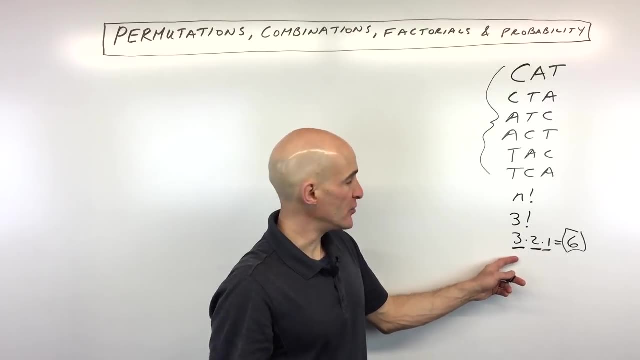 oftentimes this is referred to as the fundamental counting principle or the multiplication counting principle, And basically what you're doing is you're saying: for each category here, each letter, how many choices are there? Well, there's three choices for the first letter in your word. But 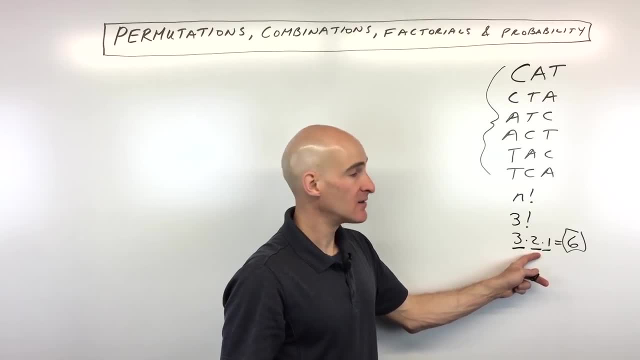 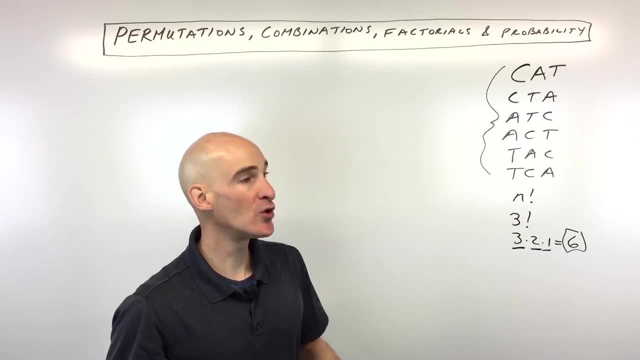 once you use that letter now, there's only going to be two choices for that second letter, And then, once you use up those two, there's only going to be one left for the third. So it's three times, two times one. Sometimes, what your teacher will do to illustrate this is to have you draw a tree. 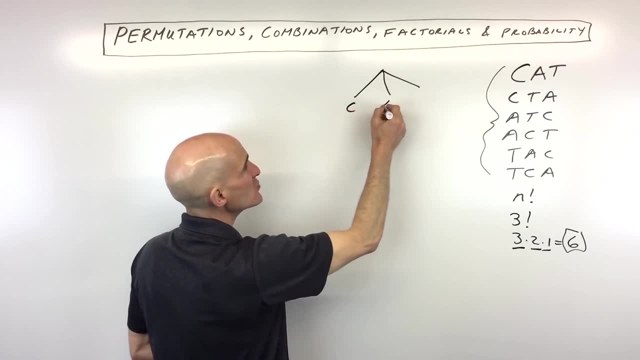 diagram, And so I'll just show you that real quick. So for the first letter, you could choose a C, A or a T. Once you choose C, you've got two choices. You could choose A or T, If you choose. 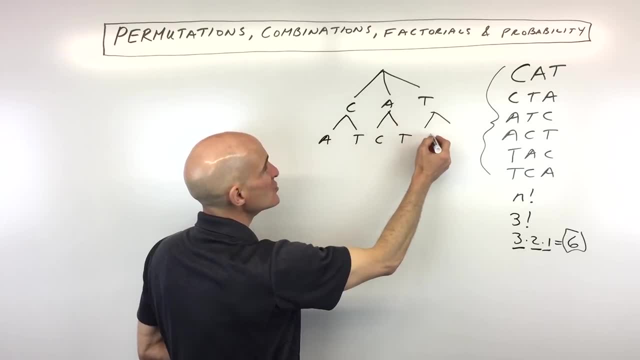 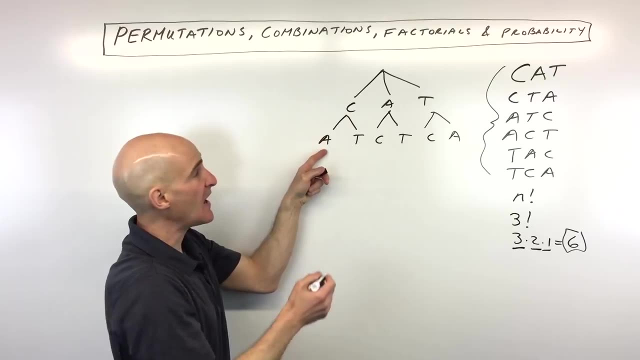 A, you have two choices. That's going to be C Or T. If you choose T, you have two choices: There's going to be C or A. So if you're going down this branch, you can see. if you've chosen C, you've chosen A. the only letter left would be T. 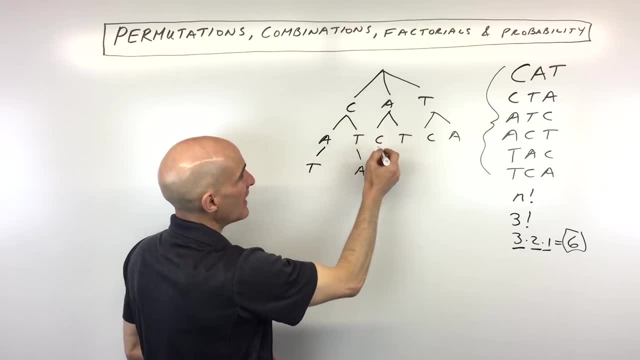 Or here would be C T. The only letter left to choose would be A A, C, T, A, T, C, T, C, A, T, A, C, And again you can see. if you count these roots, so to speak, there's only going to be six outcomes. 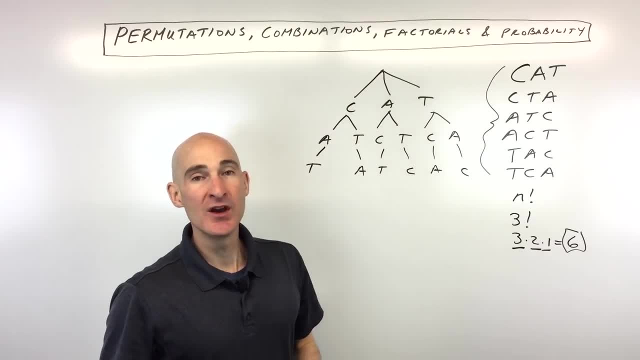 that are possible going down each of these roots. So that's the idea there. Now what happens if you want to take permutations of n objects r at a time. Say, for example, you only wanted to make like a two-letter word using these: 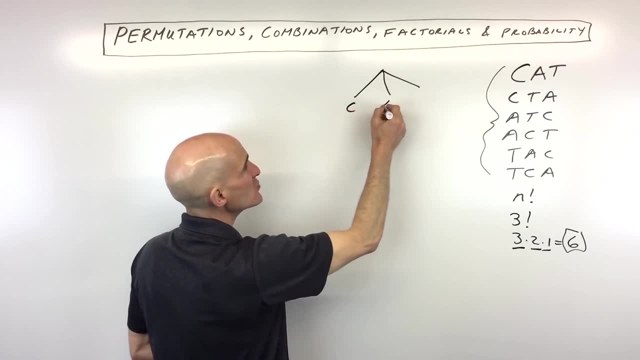 diagram, And so I'll just show you that real quick. So for the first letter, you could choose a C, A or a T. Once you choose C, you've got two choices. You could choose A or T, If you choose. 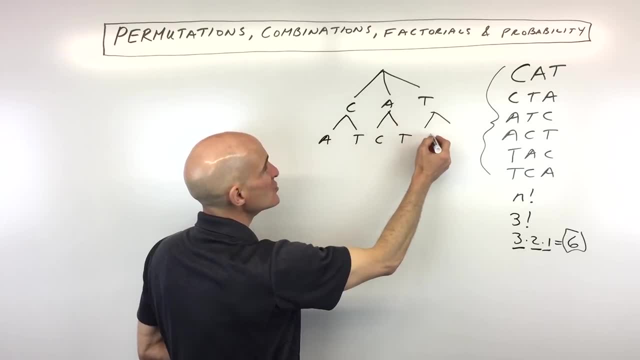 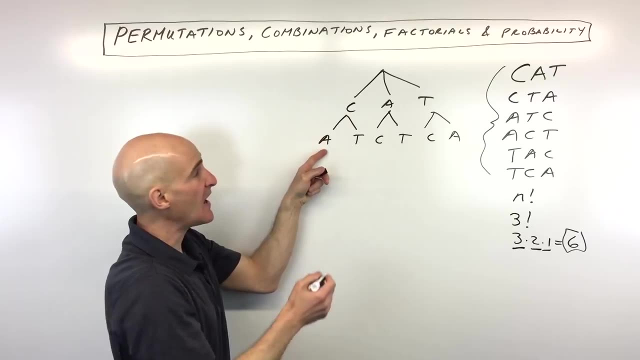 A, you have two choices. That's going to be C Or T. If you choose T, you have two choices: There's going to be C or A. So if you're going down this branch, you can see. if you've chosen C, you've chosen A. the only letter left would be T. 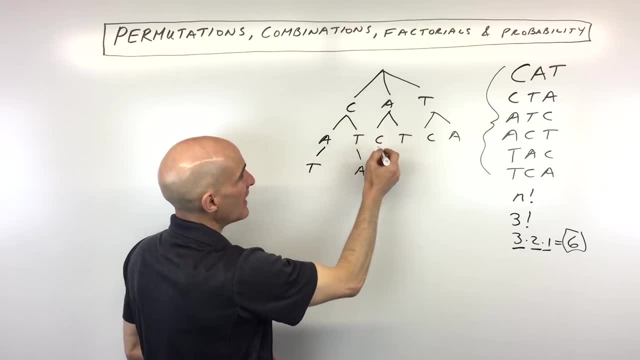 Or here would be C T. The only letter left to choose would be A A, C, T, A, T, C, T, C, A, T, A, C, And again you can see. if you count these roots, so to speak, there's only going to be six outcomes. 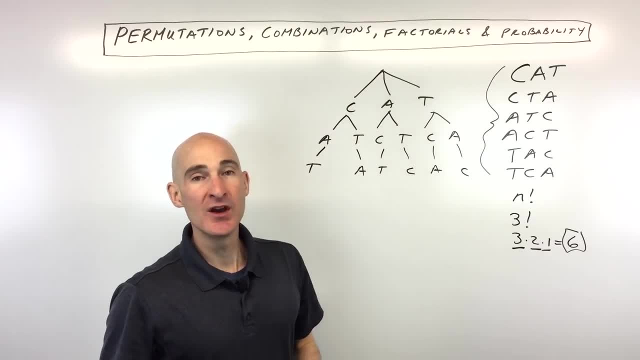 that are possible going down each of these roots. So that's the idea there. Now what happens if you want to take permutations of n objects r at a time. Say, for example, you only wanted to make like a two-letter word using these: 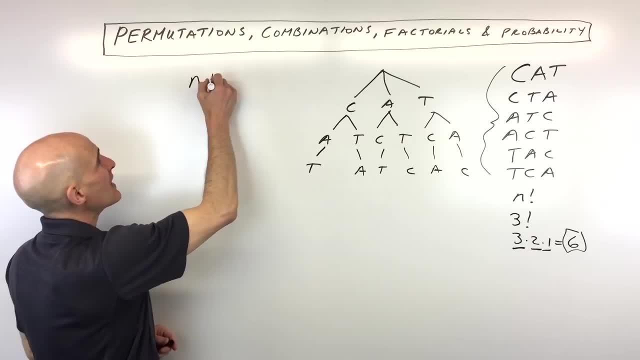 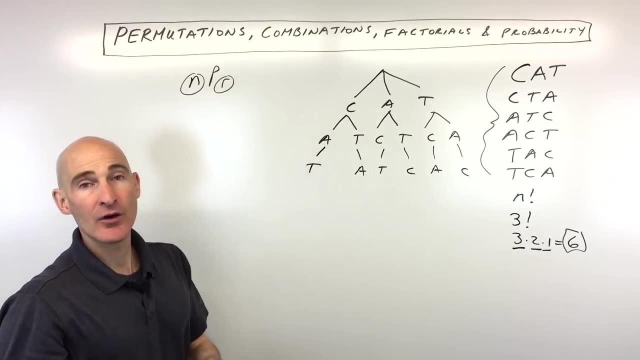 three letters. Well, in walks NPR. So what is NPR? Well, NPR means: out of n objects, how many ways are there to pick r of them? where the order is important? And there's a formula you're going to want to memorize, and we'll talk about this in a minute. It's 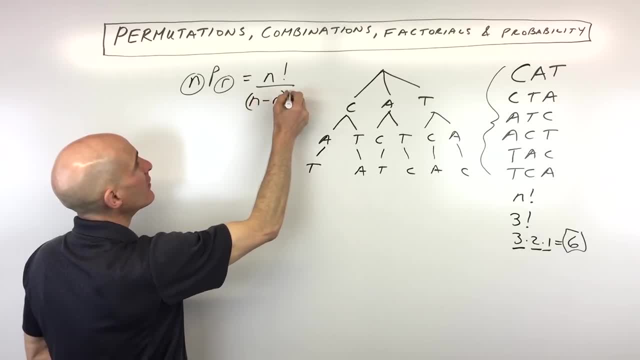 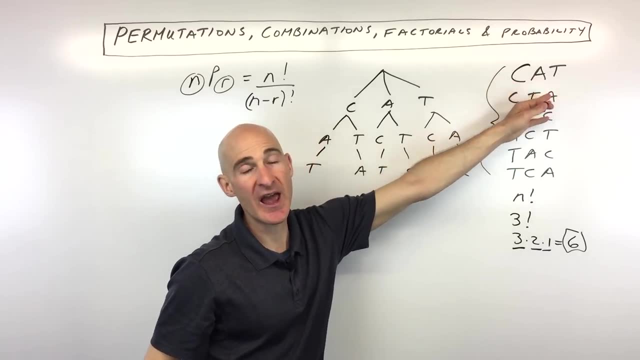 N factorial, over n minus r Factorial. OK, so let's do an example. Say we want to make a two-letter word out of the letters in the word cat. So let's just write them out for a minute, So we could have C-A. 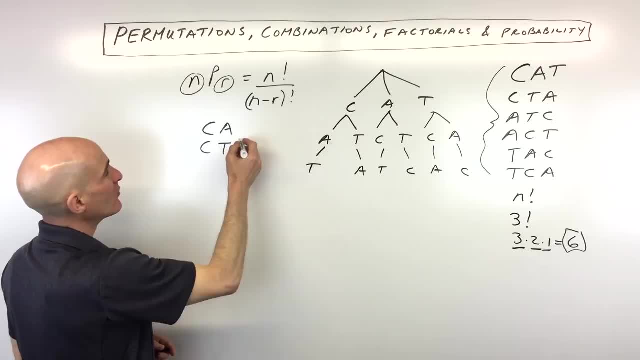 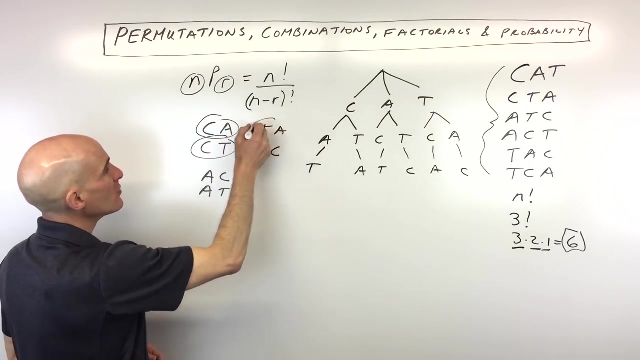 we could have C-T, we could have what else? We could have A-C, we could have A-T, we could have T-A and we could have T-C. So you can see there's a, one, two, three, four, five, six, seven, eight, nine, ten. ten, eleven, twelve, thirteen, fourteen, fifteen, sixteen, seventeen, eighteen, nineteen, twenty, twenty-two, twenty-three, twenty-three, twenty-four, twenty-five, twenty-six possibilities, Six ways of making a two-letter word where the order is important. So C-A is different. 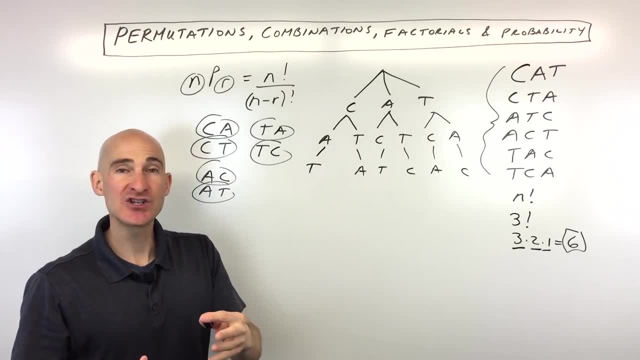 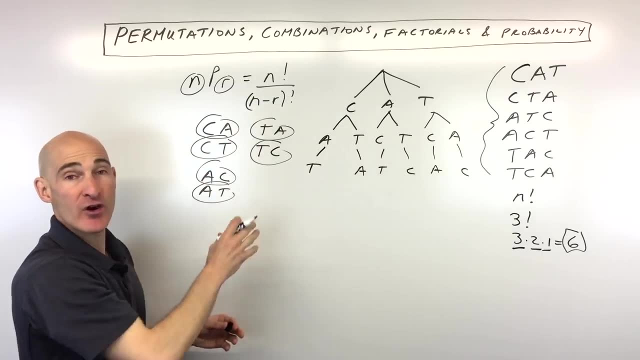 from A-C. Now we're going to talk about, in just a minute, combinations where the order is not important, and we'll talk about that in just a second. But notice, here there's another way to calculate this. instead of writing all these out, We can use the formula We. 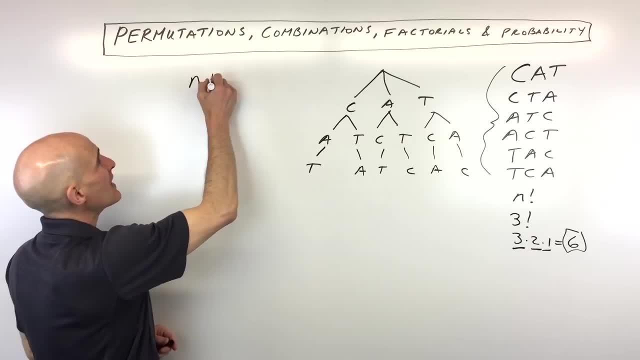 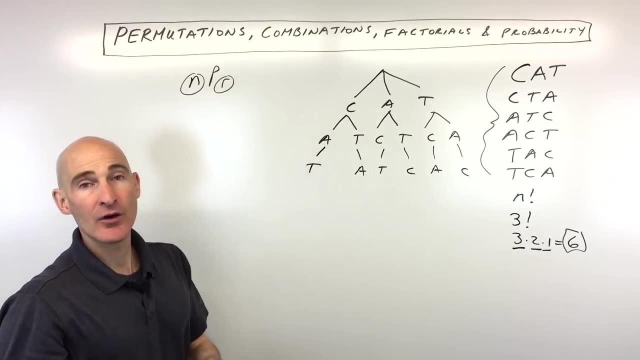 three letters. Well, in walks NPR. So what is NPR? Well, NPR means: out of n objects, how many ways are there to pick r of them? where the order is important? And there's a formula you're going to want to memorize, and we'll talk about this in a minute. It's 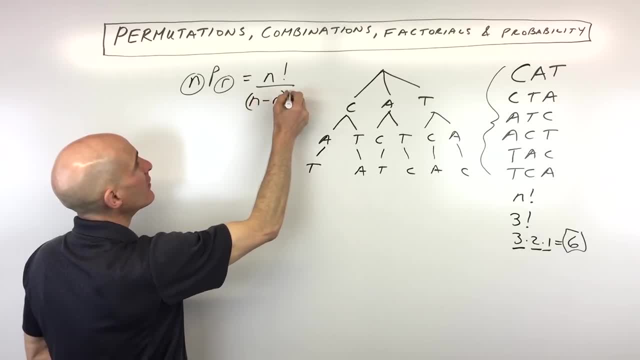 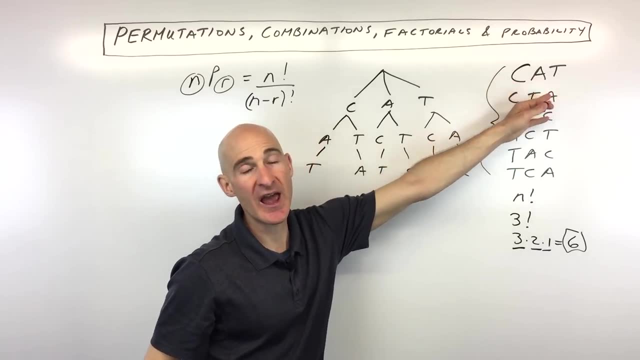 N factorial, over n minus r Factorial. OK, so let's do an example. Say we want to make a two-letter word out of the letters in the word cat. So let's just write them out for a minute, So we could have C-A. 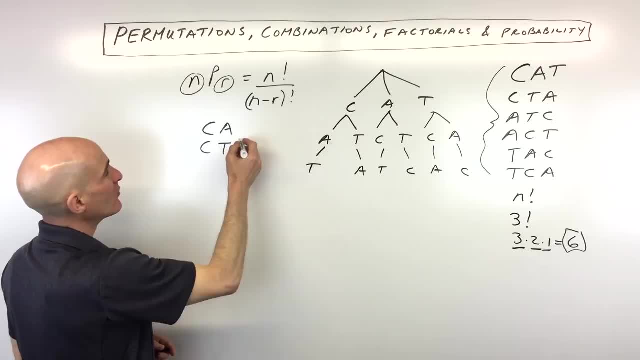 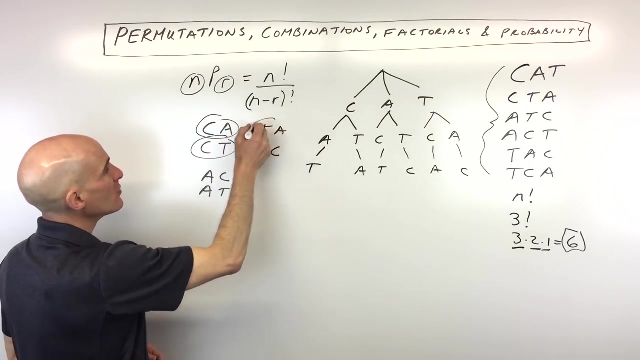 we could have C-T, we could have what else? We could have A-C, we could have A-T, we could have T-A and we could have T-C. So you can see there's a, one, two, three, four, five, six, seven, eight, nine, ten. 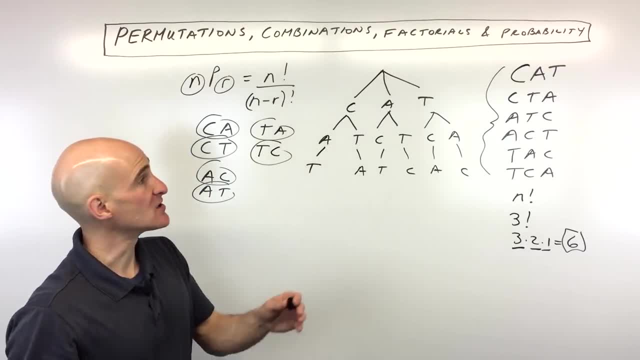 ten, eleven, twelve, thirteen, fourteen, fifteen, sixteen, seventeen, eighteen, nineteen, twenty, twenty-one, twenty-two, twenty-three, twenty-three, twenty-four, twenty-five, twenty-six possibilities, six ways of making a two-letter word, where the order is important. So C-A. 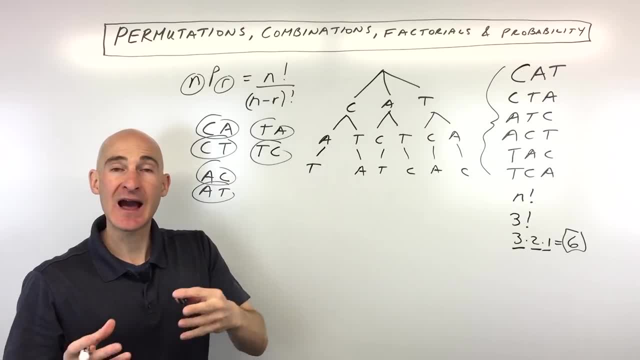 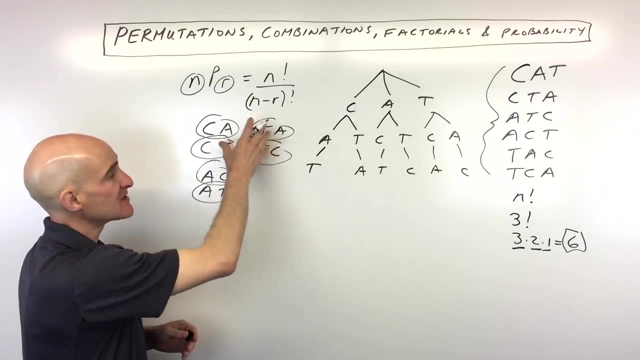 is different from A-C. Now we're going to talk about in just a minute combinations where the order is not important, and we'll talk about that in just a second. But notice, here there's another way to calculate this. instead of writing all these out, We can use the formula. 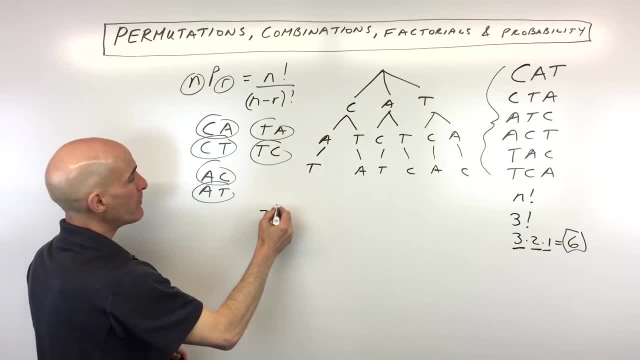 We can say: out of three letters- see C-A and T- we're going to pick two. OK, now I'm just using the word pick just as a way of thinking about this. So let's say: we're going to pick two. OK, now I'm just using the word pick just as a way of thinking about this. So let's: 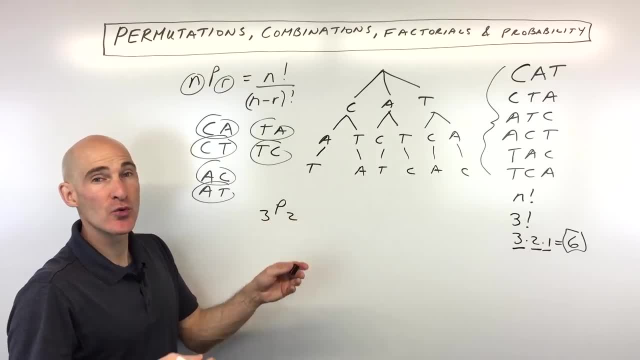 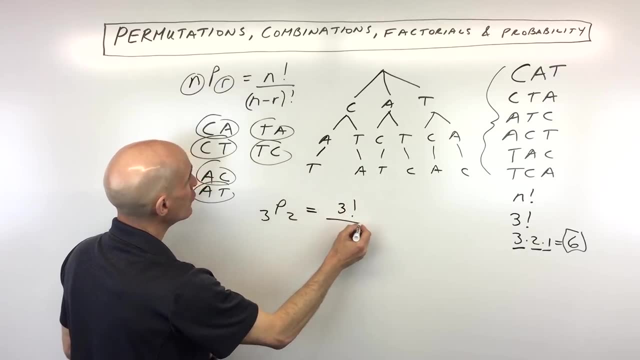 out of three items, we want to say how many ways are there to pick two where the order is important. So, using our formula, you can see that N equals three, R is equal to two. so this is going to be three factorial over three minus two factorial. Now remember the. 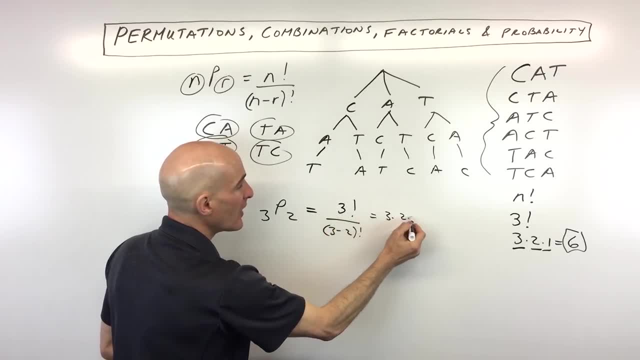 way the factorials work. You start at this number and you multiply down to one. Three minus two is one factorial. One factorial is just going to be one. so you would get three times two times one, which is six over one, which equals six different ways you're. 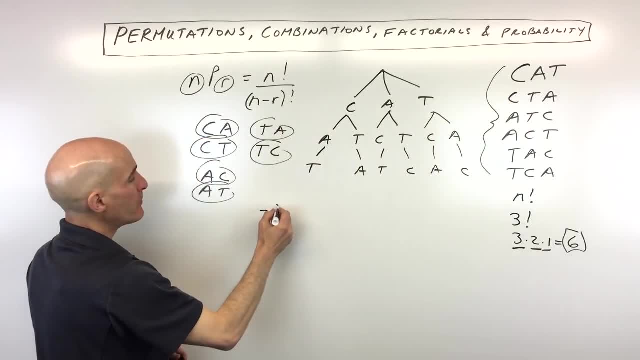 can say: out of three letters- C-A and T- we're going to pick two. OK, now I'm just using the word pick just as a way of thinking about this, But we're going to pick two. So we're going to say: out of three items you want to say, how many ways are there to pick two? 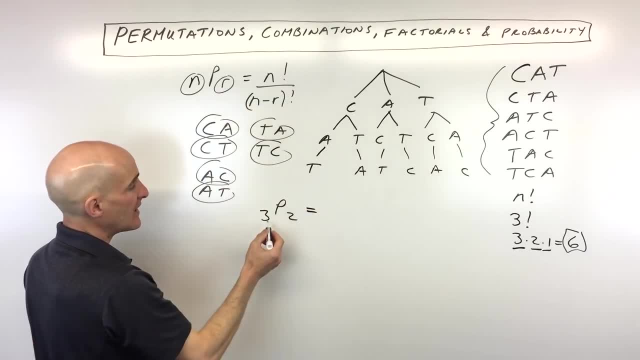 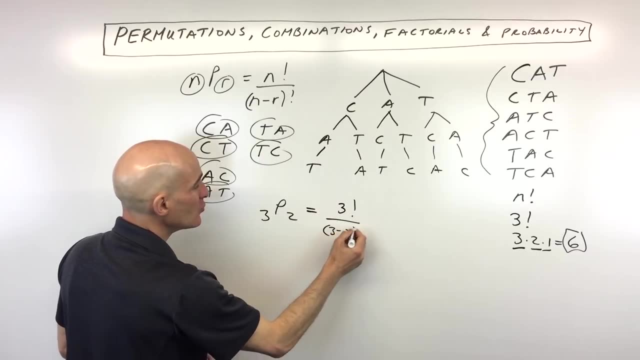 where the order is important. So using our formula, you can see that N equals three, R is equal to two. So this is going to be three factorial over three minus two factorial. Now remember the way the factorials work. You start at this number and you multiply. 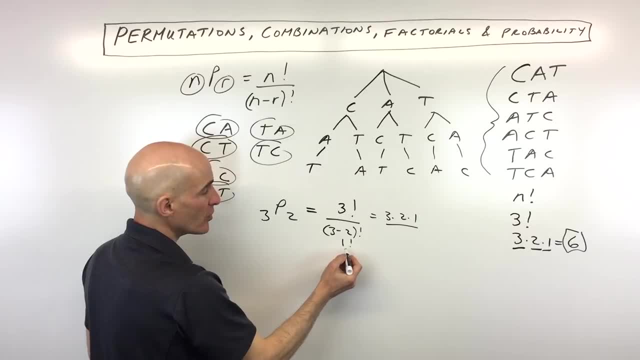 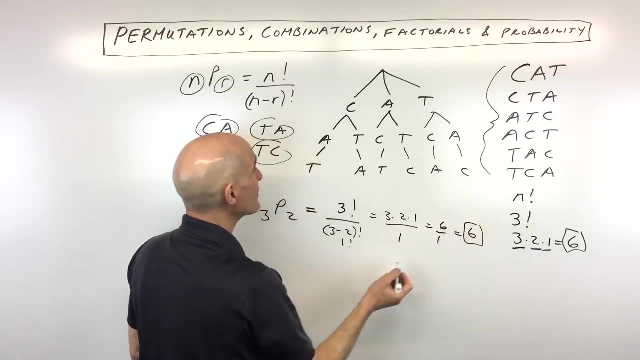 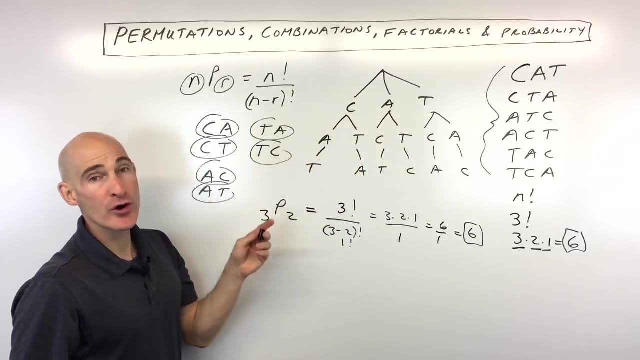 down to one. Three minus two is one factorial. One factorial is just going to be one. So you would get three times two times one, which is six over one, which equals six different ways of picking two letters out of the three letters that we started with to make a word. 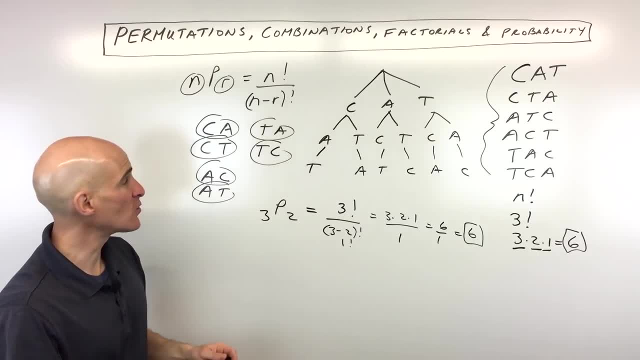 where the order is important. Now say, for example, the order is not important, So this is when we're going to be talking about combinations And combinations. you can see that A-C and C-A- these are actually the same two letters. So, for example, if you were going to pick, 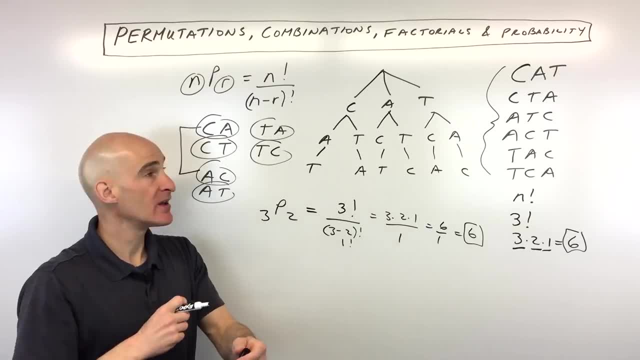 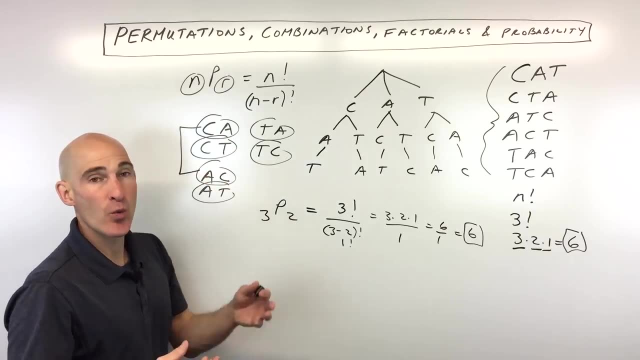 two items out of a bag of three items. it doesn't matter if you pick C first and then C or A first and then C, because you're going to end up with those two items anyways. So we would only count this as one result or one combination. Same thing here We've. 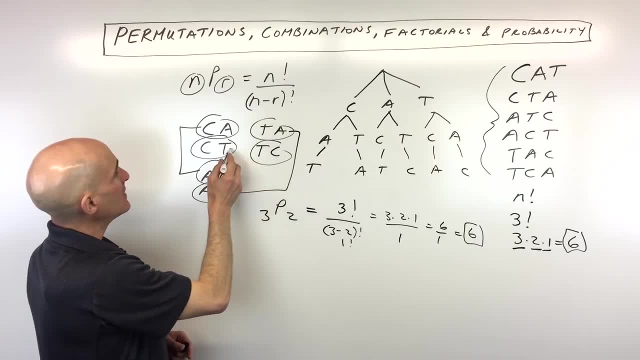 got T-A and A-T and then we have C-T and T-C. So you can see we've grouped those together. So there's really only three unique outcomes here, three distinct outcomes. And the way we would do this is we would use our combination formula, that's N-C-R. And the way this works. 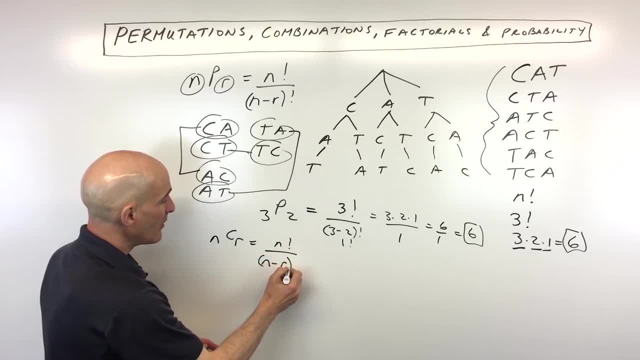 is it's N factorial over N minus R, R factorial, R factorial. Now notice how this formula and this formula- they're almost exactly the same, right? The only difference is that we're dividing by this R factorial, And what this means is that we're dividing out the duplicates. We don't want to count A and C. 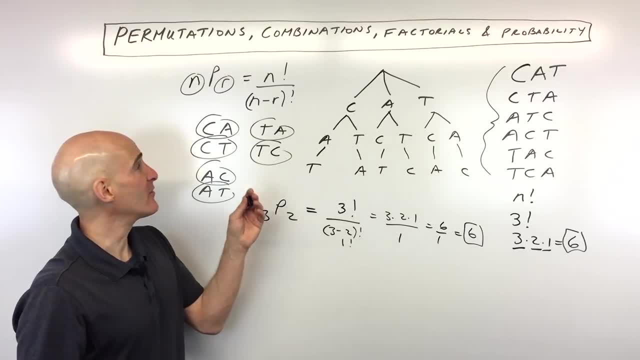 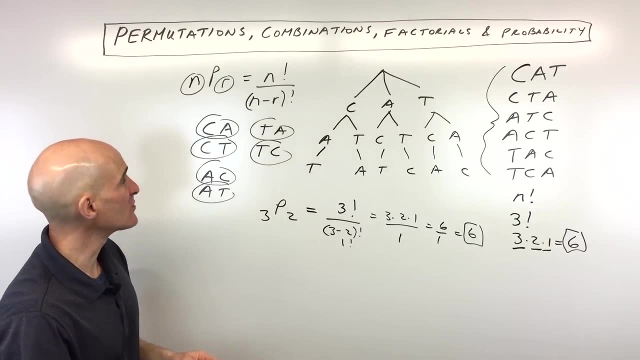 of picking two letters- okay- out of the three letters that we started with, to make a word where the order is important. now say, for example, the order is not important, so this is when we're going to be talking about combinations and combinations. you can see that AC- okay, and CA. 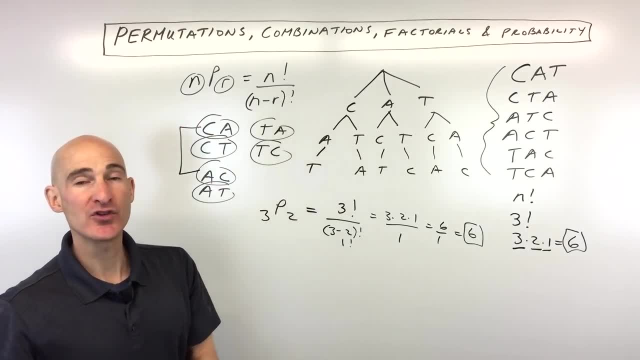 these are actually the same two letters. so, for example, if you were going to pick, you know, two items out of a bag of three items, it doesn't matter, you know, if you pick C first and then, or A first and then C, because you're going to end up with those two items anyways. okay, so we 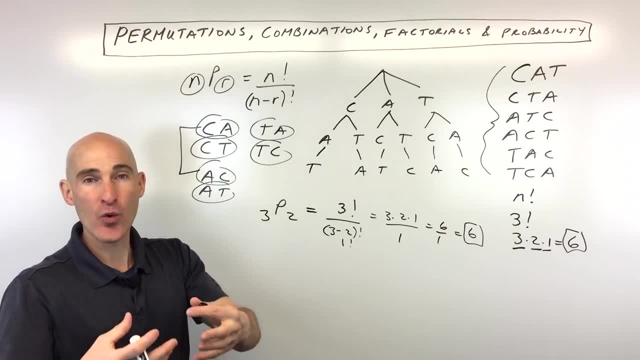 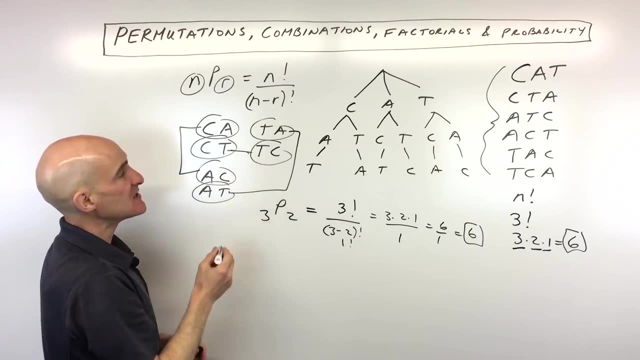 would only count this as one result. okay, or one combination. same thing. here. we've got TA and AT, and then we have CT and TC. so you can see we've grouped those together. so there's really only three unique outcomes here, three distinct outcomes, and the way we would do this is we would use our 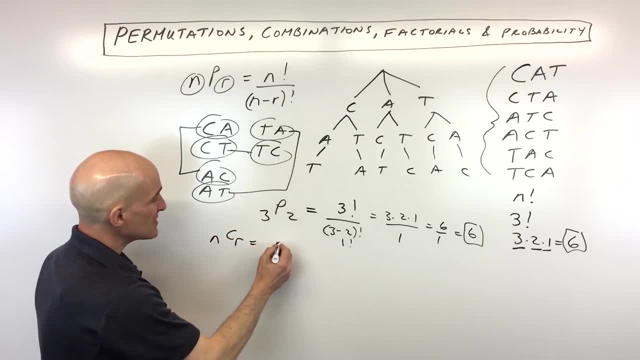 combination formula. it's NCR and the way this works is it's n factorial over n, minus N sub n, and we consider it always as a matrix and this is why you have to use n over n over n changes R factorial, R factorial. Now notice how this formula and this formula- they're almost exactly. 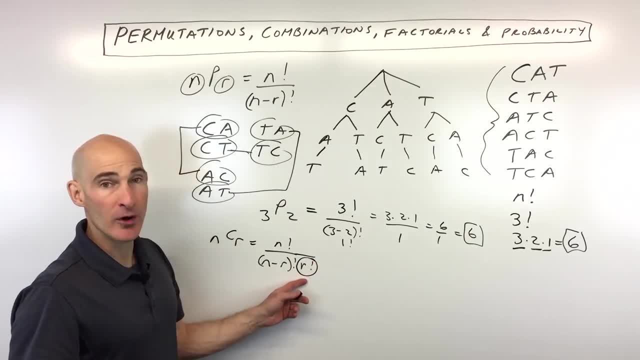 the same right. The only difference is that we're dividing by this R factorial, And what this means is that we're dividing out the duplicates. We don't want to count A and C and C and A as the same. So what we're doing is we're, you know, as different? I should say they're the same, So we. 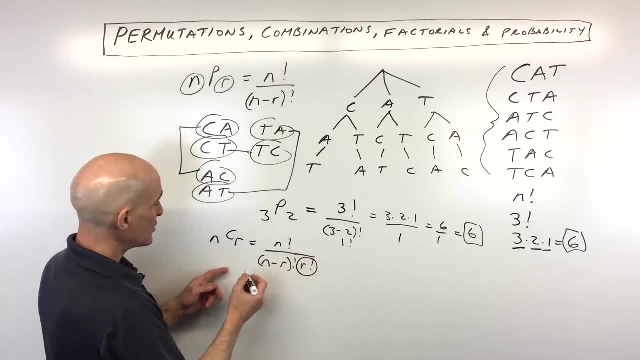 want to double count those, We want to divide out those multiplicities. So in this particular example, we had three letters. okay, C-A-T, We're choosing two. okay, That's just one way to think about it. You know, out of three, we're choosing two. The order is not important, We just want to. 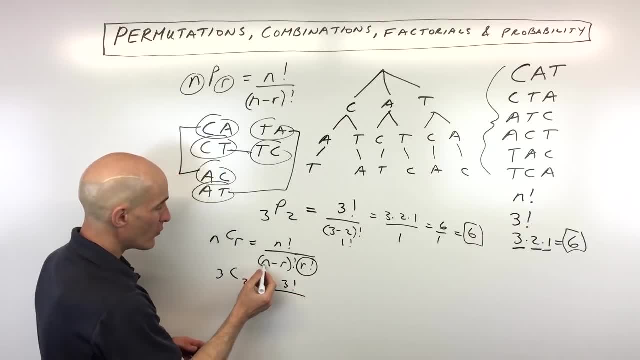 find out how many different outcomes there are. So that's going to be three factorial over three minus two, which is one factorial times two factorial. If we expand this out, we get three times two times one over one factorial, which is one. Two factorial is two times one. Notice the 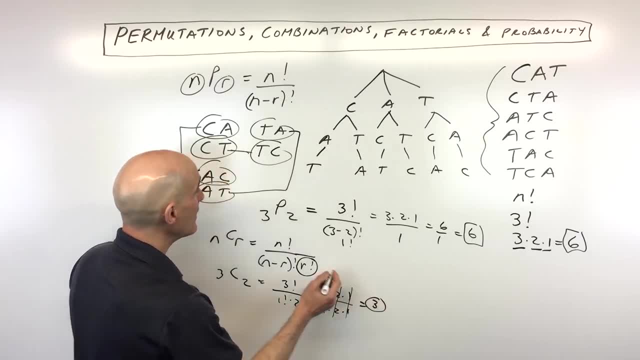 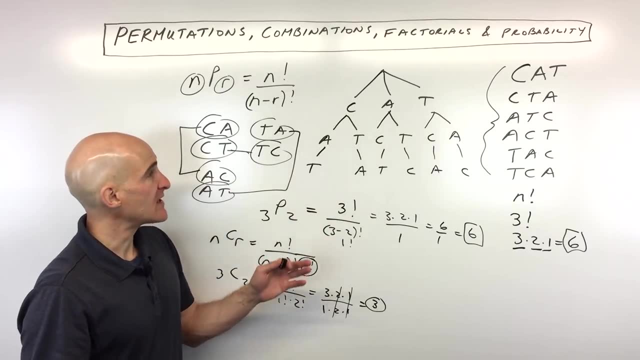 two and the one they cancel. Three divided by one is equal to three, And that's what we're finding out here, that there was actually three groups of those two letters. right, So that's the idea between permutations, combinations. But quickly, I just wanted to go back here for a 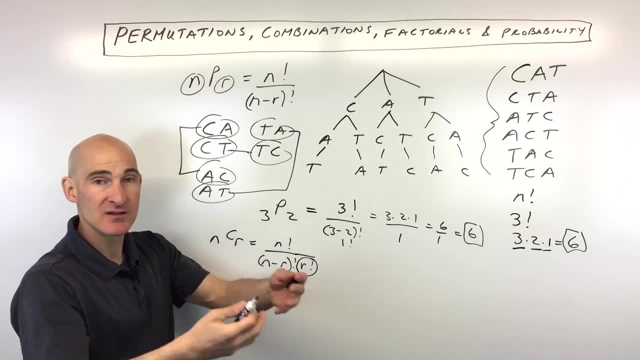 and C and A as the same. So what we're doing is we're, you know, as different. I should say they're the same. So we want to double count those, we want to divide out those multiplicities. So in this particular example, we had three letters. okay, C-A-T. We're changing them. 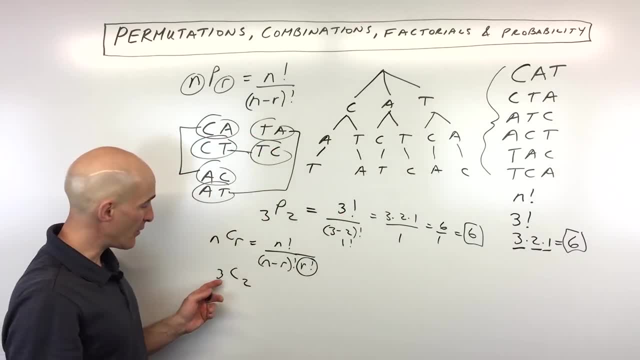 We're choosing two. Okay, that's just one way to think about it. You know, out of three we're choosing two. The order is not important, We just want to find out how many different outcomes there are. So that's going to be three factorial over three minus two, which. 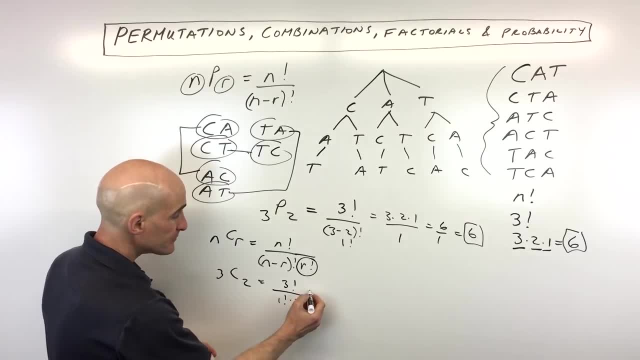 is one factorial times two factorial. If we expand this out, we get three times two times one over one factorial, which is one. Two factorial is two times one. Notice the two and the one they cancel. Three divided by one is equal to three, And that's what we 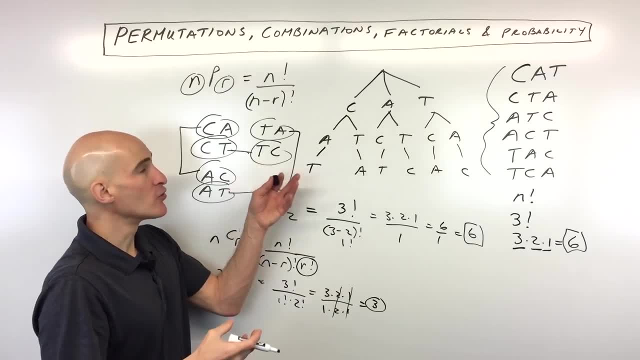 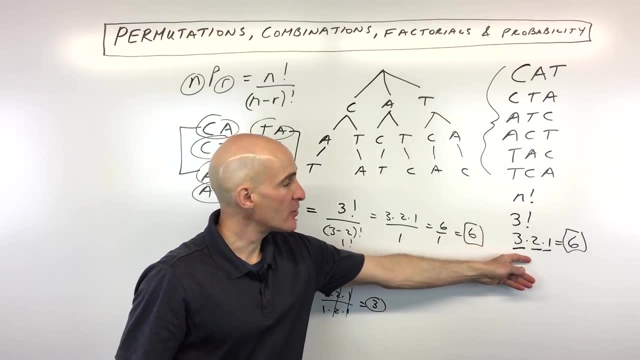 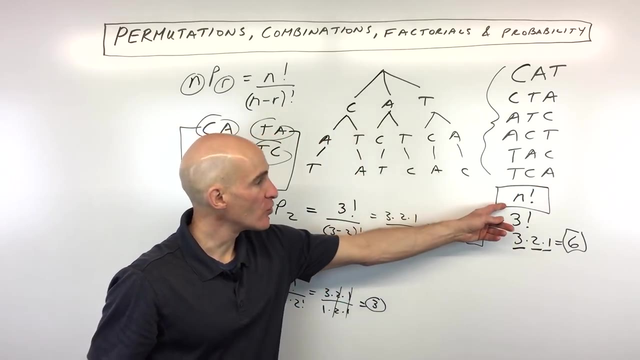 found out here that there was actually three Groups of those two letters, right. So that's the idea between permutations, combinations. But quickly, I just wanted to go back here for a moment. We were talking about this formula, n factorial. So the n factorial represents you know how many ways to arrange all n items. 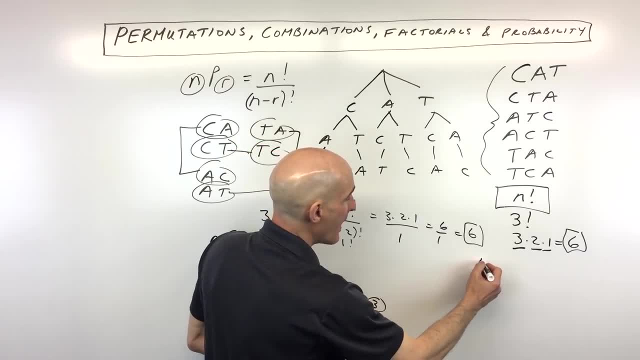 So, for example, if we had like a word, say, for example, like math, right, M-A-T-H, And we say, well, how many ways can we rearrange all of the letters? You can see there's four letters, So we would say that this is four factorial. 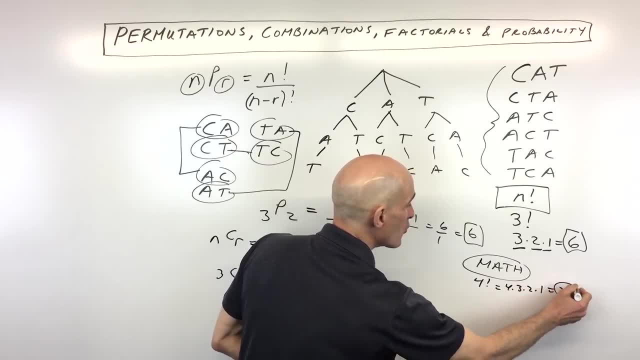 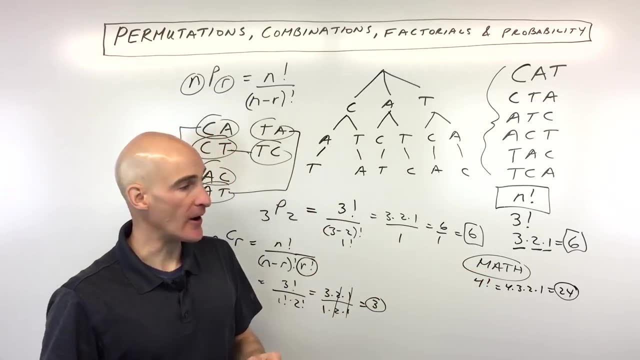 That's going to be four times, three times, two times one, which means there's 24 different ways to use all four letters and rearrange those and make you know a different so-called word. right, It might not actually be a word, but it'll look like you know, like a four. 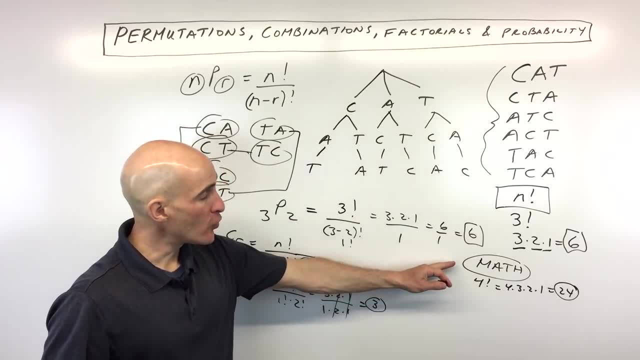 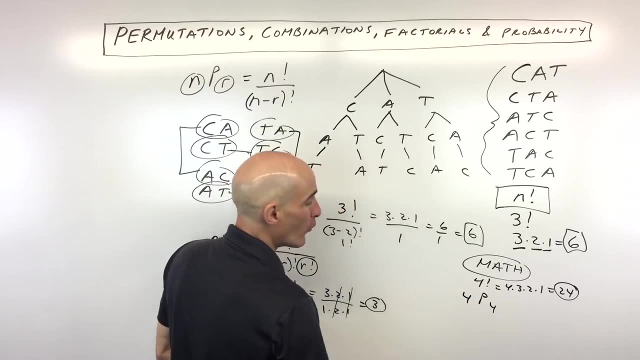 letters right In a different order. Now, another way to do this problem is to use the permutations formula, the NPR. The only difference is we would be saying 4P4.. So we'd say, out of four letters we're going to pick four, So basically all of them. And if we're going 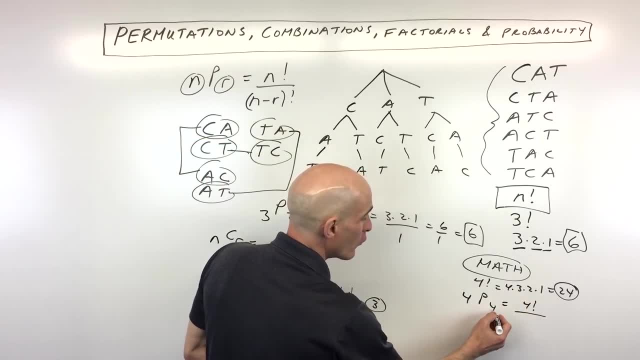 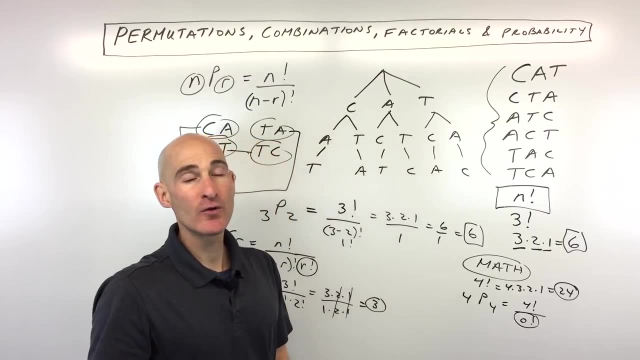 to use our formula, you can see this is going to be four factorial over four minus four, zero factorial. So I'm just doing n minus r, But zero factorial. this is one that you're going to want to memorize. Zero factorial is equal to one. Okay, so you weren't going. 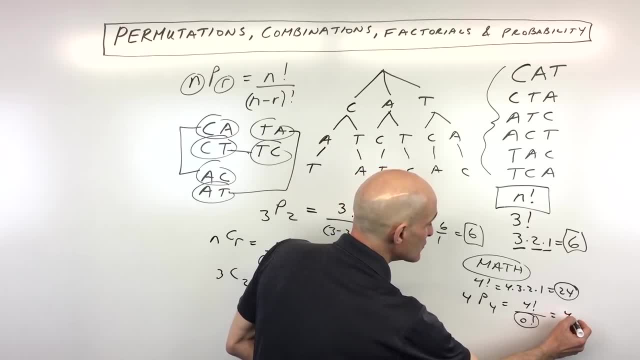 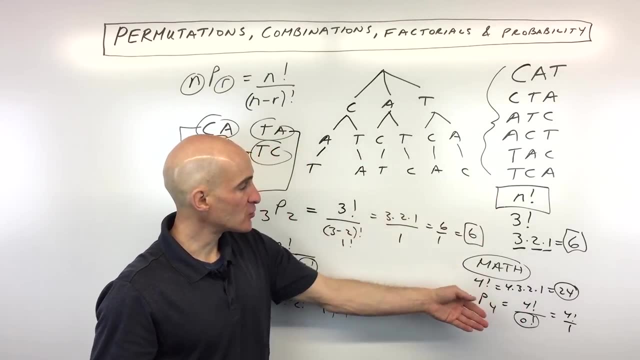 to memorize that. So you can see, zero factorial is one. So we end up just with four factorial, like we had up here, which is 24.. So two different ways to do it. You can either use the formula n factorial or you could use the NPR formula. Now, if you take a word like algebra and you 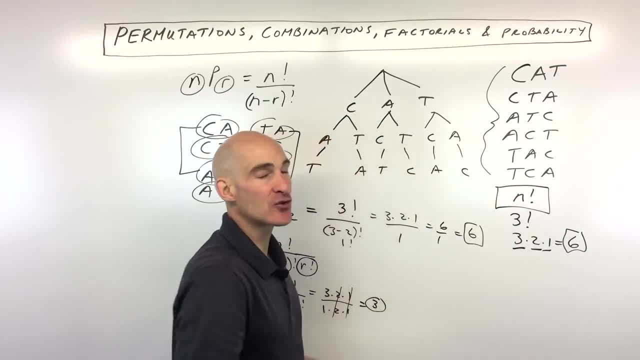 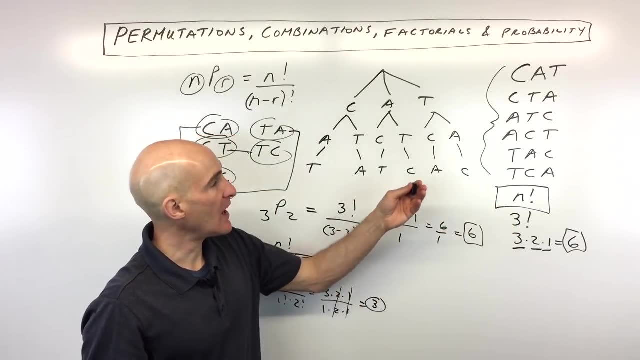 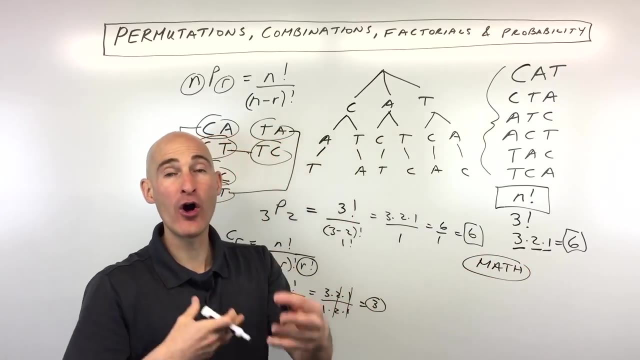 moment We were talking about this formula, N factorial. So the N factorial represents, you know, how many ways are to arrange all N items. So, for example, if we had like a word say, for example, like math right, M-A-T-H, And we say, well, how many ways could we rearrange all of the 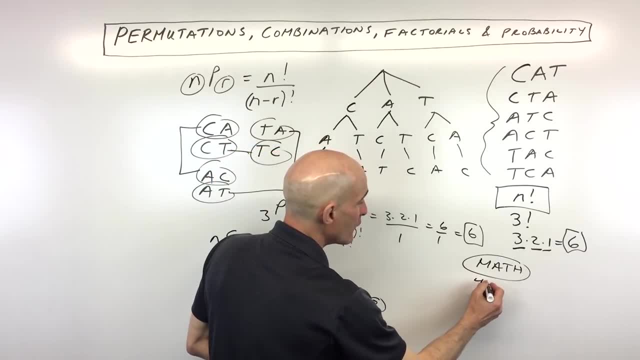 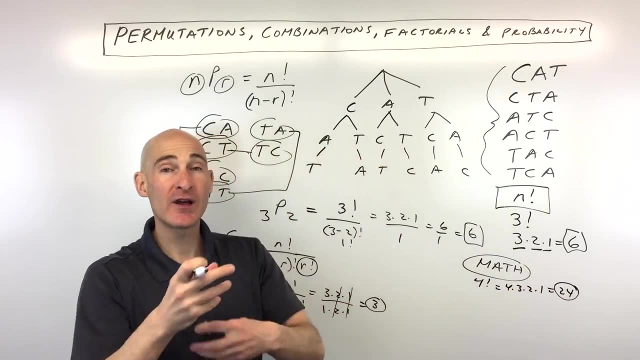 letters. We can see there's four letters, So we would say that this is four. factorial. That's going to be four times, three times, two times one, which means there's 24 different ways to use all four letters and rearrange those and make you know a different so-called word. right, It might not. 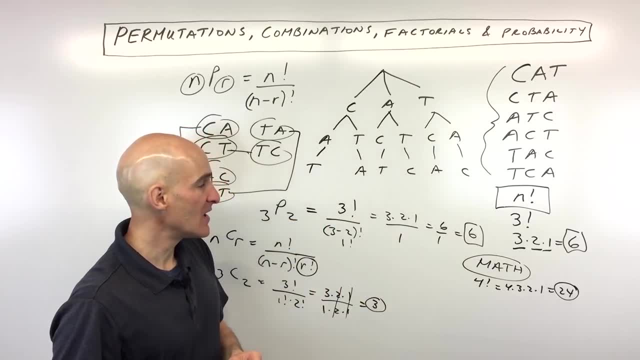 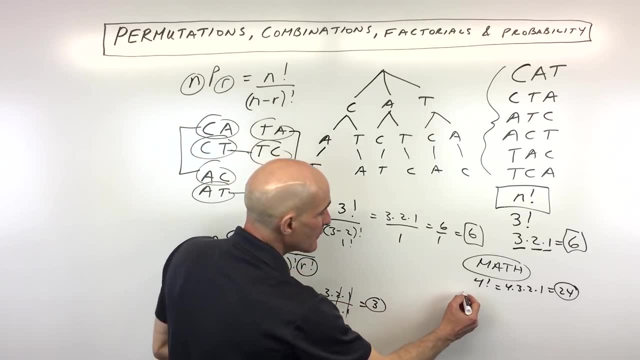 actually be a word, but it'll look like, you know, like a four letters right In a different order. Now, another way to do this problem is to use the permutations formula, the NPR. The only difference is we would be saying four P, four. 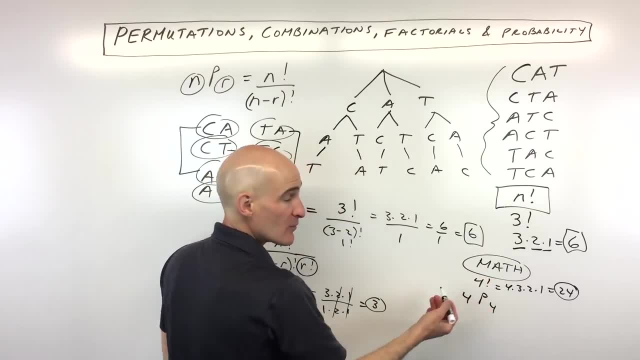 So we'd say, out of four letters, we would be saying four, P four. So we'd say out of four letters we're going to pick four. so basically all of them. And if we use our formula you can see this is: 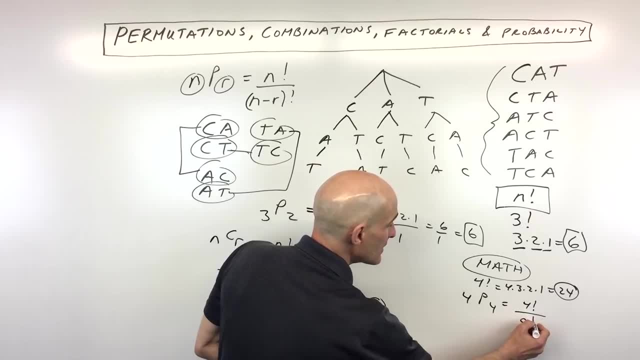 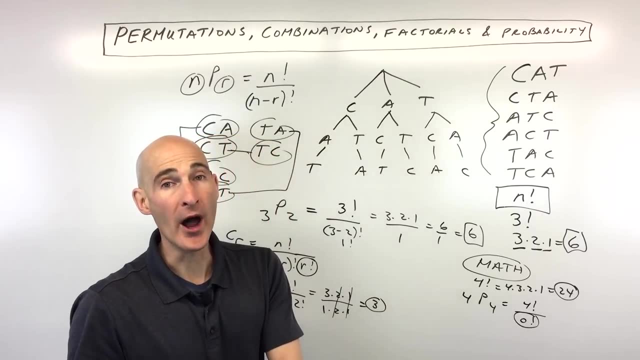 going to be four factorial. over four minus four is zero factorial. So I'm just doing N minus R, but zero factorial. this is one that you're going to want to memorize. Zero factorial is equal to one. Okay, so you weren't going to memorize that. So you can see zero factorial is one. So we end up just 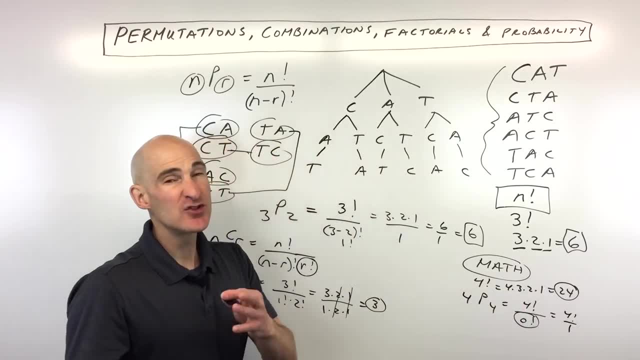 with four factorial, like we had up here, which is 24.. So two different ways to do it. You can either use the formula N factorial or you could use the NPR four. So we're going to pick four, so basically all of them, And if we use our formula you can see this is going to be four factorial over. 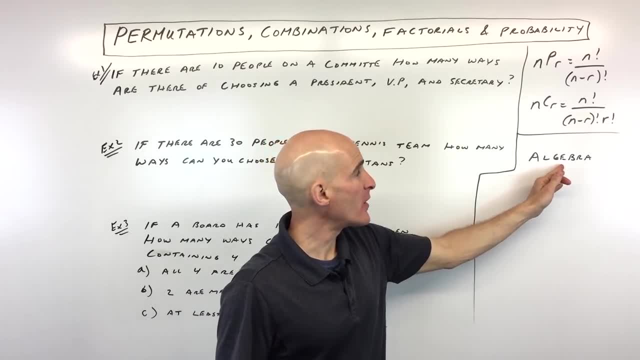 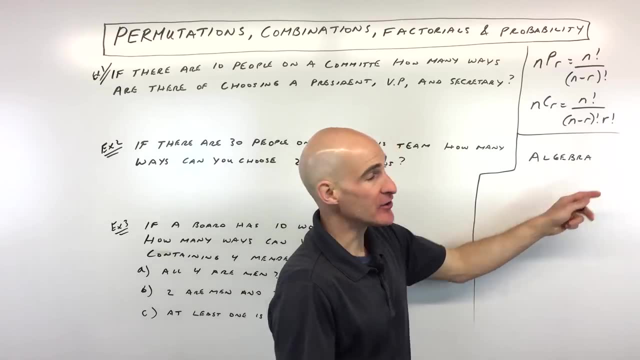 formula. Now, if you take a word like algebra and you want to find out the number of permutations of all the letters in the word algebra, you can see that there's one, two, three, four, five, six, seven letters. So there's going to be seven factorial ways of you know rearranging all. 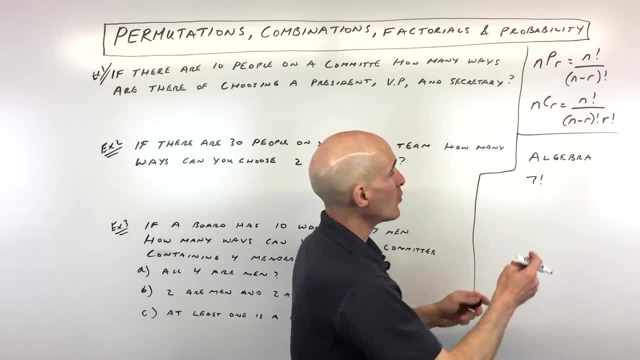 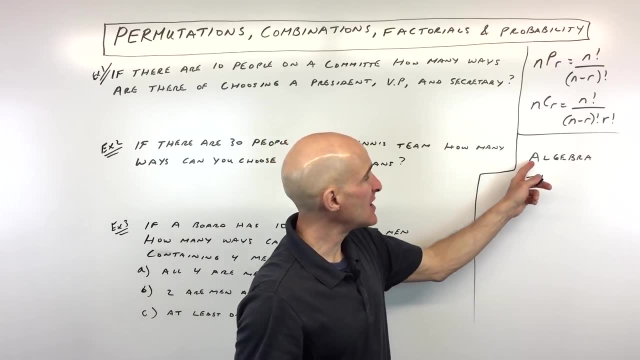 seven of those letters. But notice how that there's two A's. So when there's multiple letters, you know there's repetitions. what you want to do is you want to divide out those multiplicities. So in this case, because there was two A's, we're dividing by two factorial. two factorial is just. 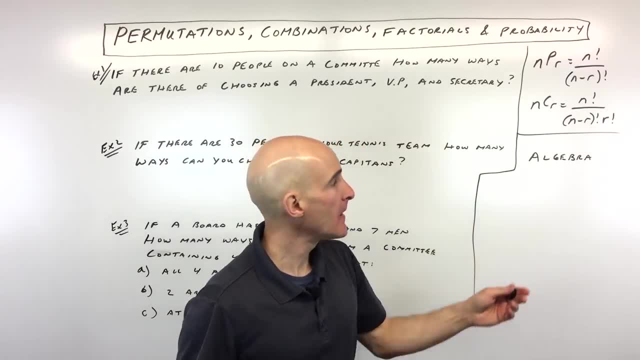 want to find out what the formula is. you're going to want to find out what the formula is about the number of permutations of all the letters in the word algebra. You can see that there's one, two, three, four, five, six, seven letters, So there's going to be. 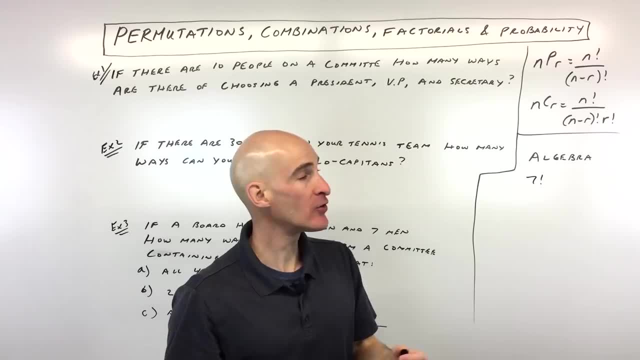 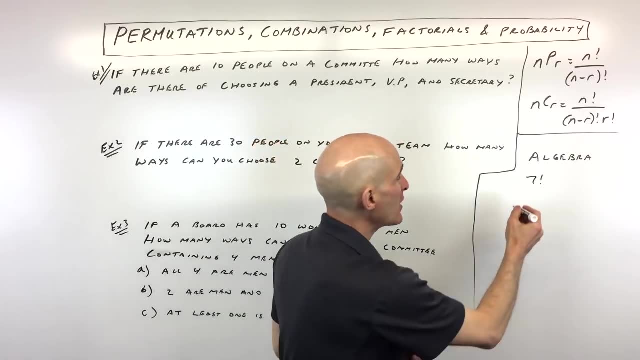 seven factorial ways of rearranging all seven of those letters. But notice how that there's two a's. So when there's multiple letters, there's repetitions, what you want to do is you want to divide out those multiplicities. So in this case, because there was two a's, 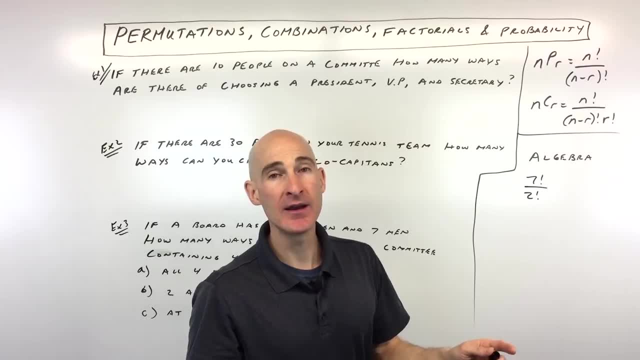 we're dividing by two factorial. Two factorial is just two times one, which is two, And you can see that if I was to put this a here and this a there, it would be two factorial And this a here. it would still look like the word algebra. So we don't want to double count. 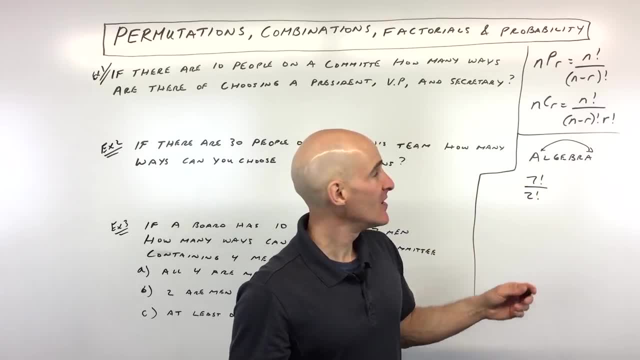 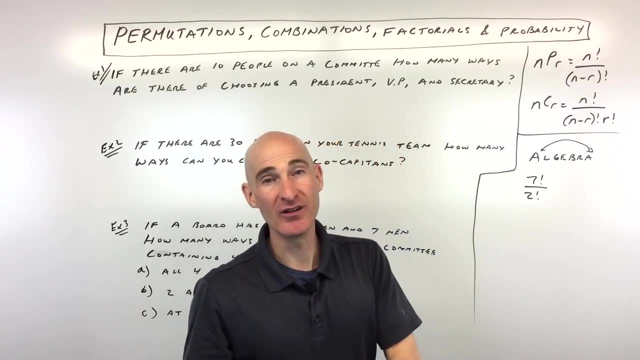 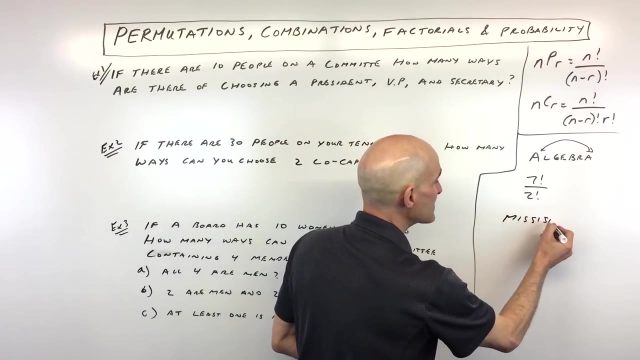 that as the same. We want to count it as a separate permutation. We don't want to basically treat that as a different word. It's going to look like the same words. We want to divide out those multiples. Take another example, like Mississippi, M-I-S-S-I-S-S-I-P-P-I, This one has 11 letters. So there's going. 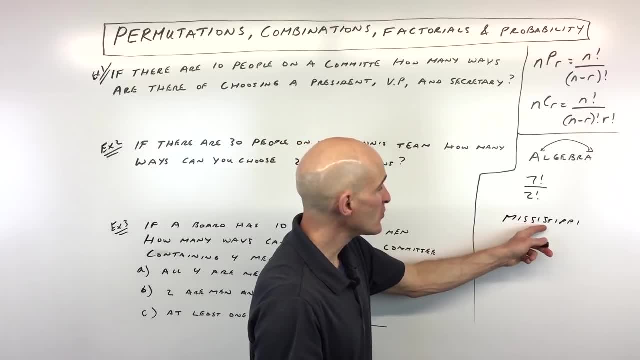 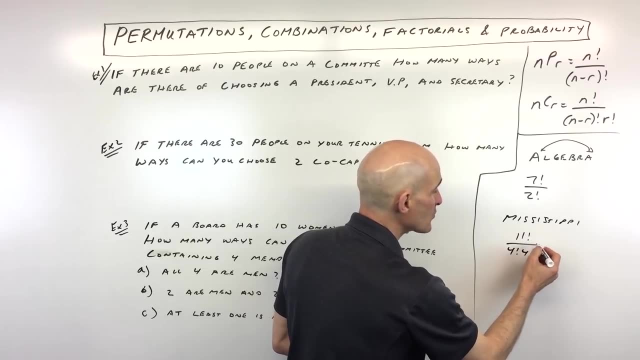 to be 11 factorial ways of rearranging those 11 letters. But notice, we've got four s's, So we're going to divide by four factorial. We've got four i's, We divide by four factorial. And we've got two p's. We're going to divide by two factorial. And again, all this is doing. 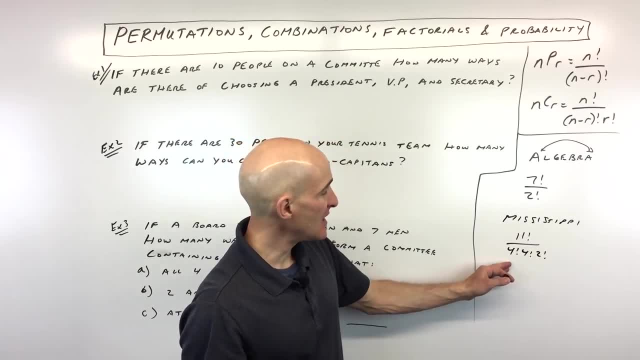 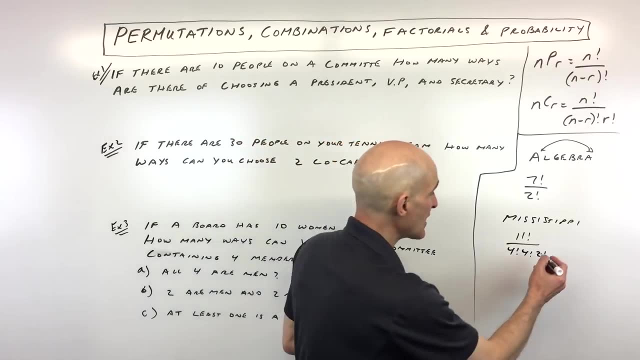 is, it's dividing out those multiples. Now you don't want to make the mistake of saying four times four. This is 16 factorial. That's not correct. You have to do these individually. So four factorial. expand this out four times, three times, two times one, Again another. 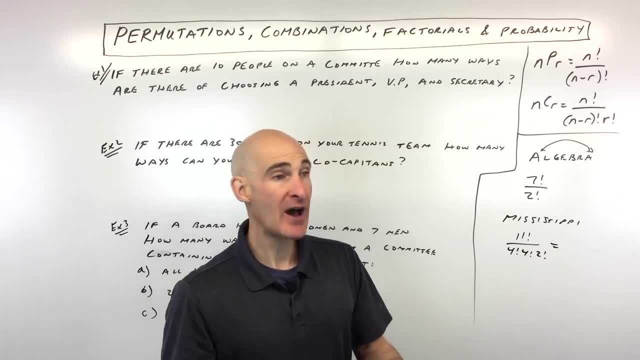 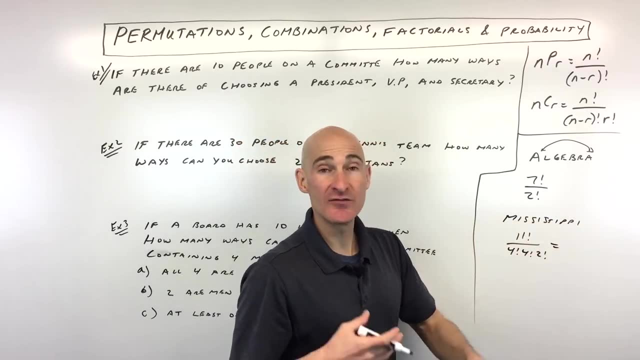 four times, three times, two times one times two times one, And just simplify them and then you can divide And that's going to be the number of distinct or different or unique. however, you want to say that permutations of all the letters in the word Mississippi. 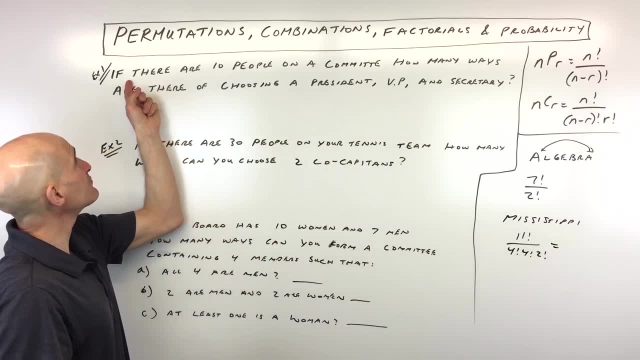 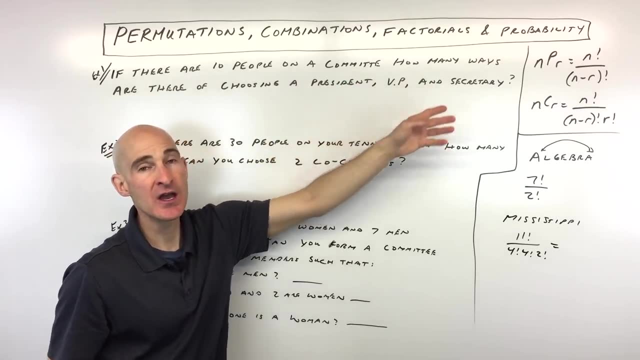 Let's go into some word problems. See if you can do these along with me here. It says: if there are 10 people on a committee, how many ways are there of choosing a president and vice president and secretary? Now, at this point we're just talking about the number. 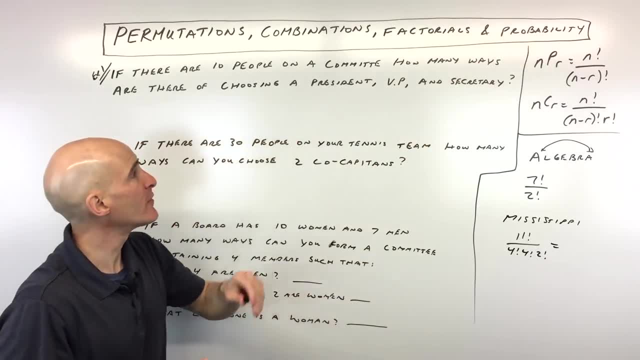 of outcomes. We're going to get into the probability in just a little bit here, But first we want to find out how many different ways there are of choosing a president, vice president, secretary, out of the 10 people on a committee. 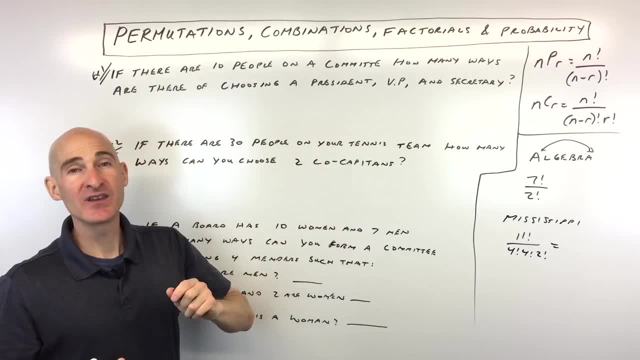 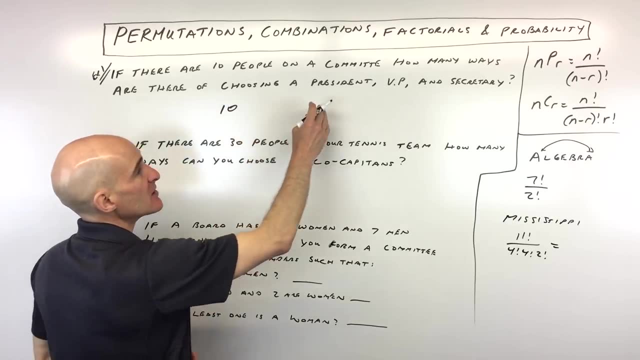 So what we're going to focus on is: is the order important or is the order not important? Well, if you were to take 10 people and you're going to basically pick three of them, right, If you change the order of those people, they're going to have a different job or a different. 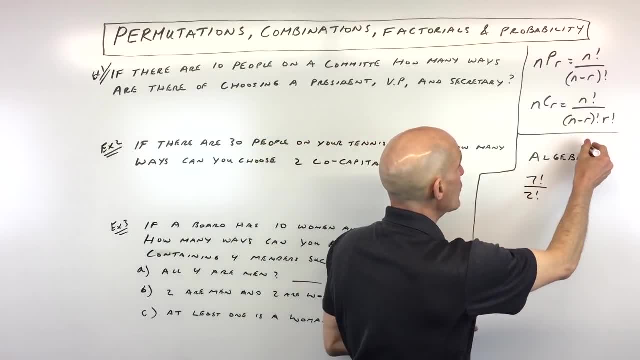 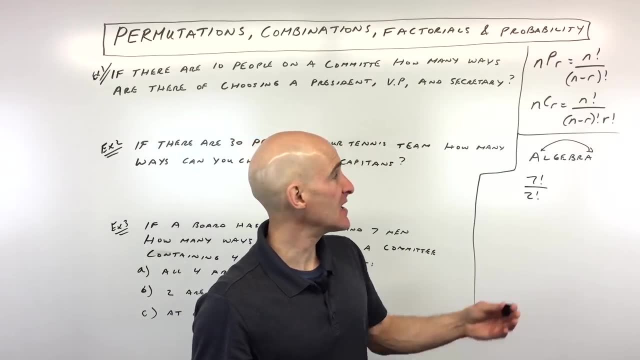 two times one, which is two, And you can see that if I was, to you know, put this A here and this A here, it would still look like the word algebra. So we don't want to double count that as a distinct, as you know the same. you want to count it as a separate permutation, right? We don't want. 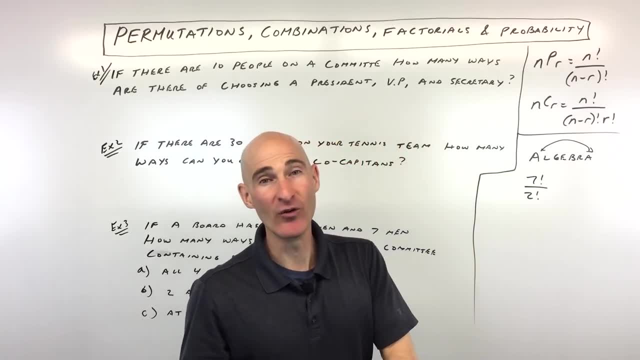 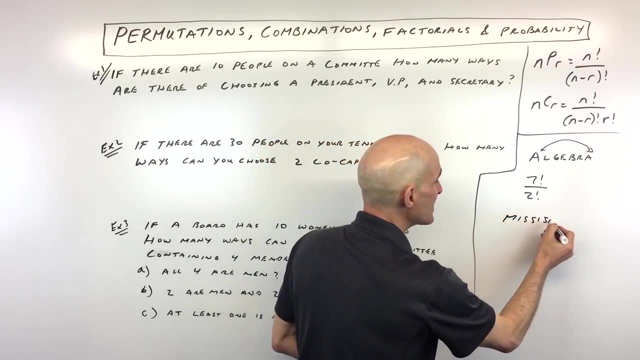 to. you know, basically treat that as a different word. it's going to look like the same words. we want to divide out those multiples, right? Take another example like Mississippi: M-I-S-S-I-S-S-I-P-P-I. 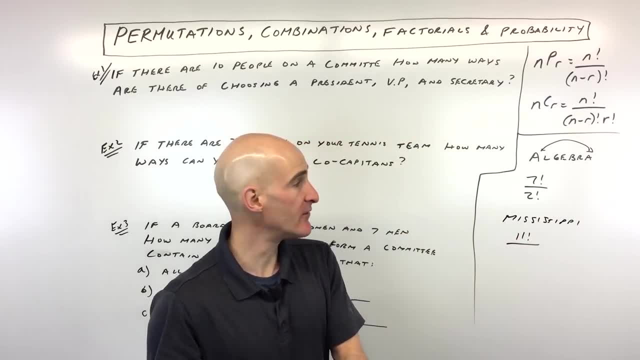 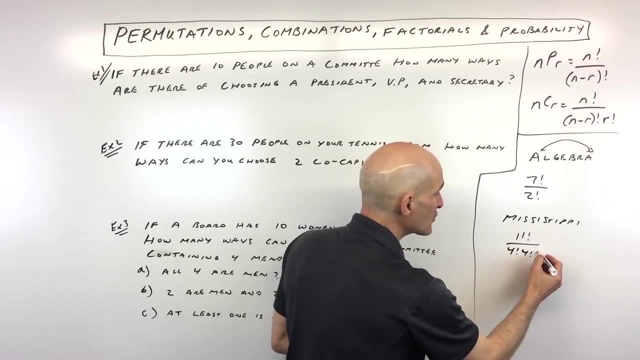 this one has 11 letters, so there's going to be 11. Factorial ways of rearranging those 11 letters. But notice, we've got four S's, so we're going to divide by four factorial. we've got four I's. we divide by four factorial. and we've got two P's. 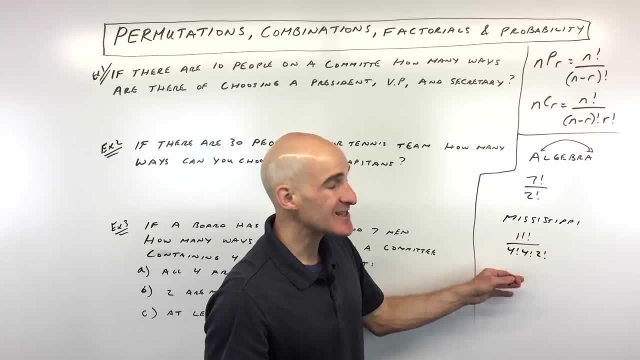 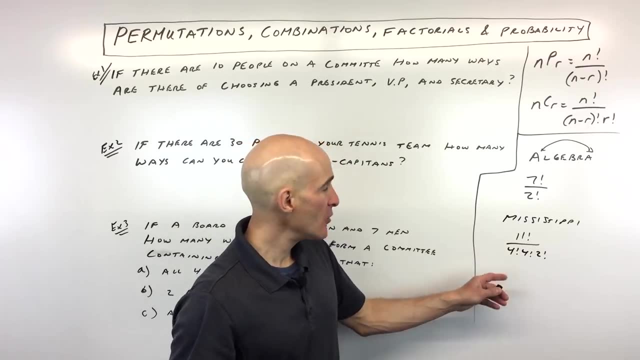 we're going to divide by two factorial And again all this is doing is it's dividing out those multiples. Now you don't want to make the mistake of saying four times four, this is 16 factorial. that's not correct. You have to do these individually. So four factorial: expand this out. 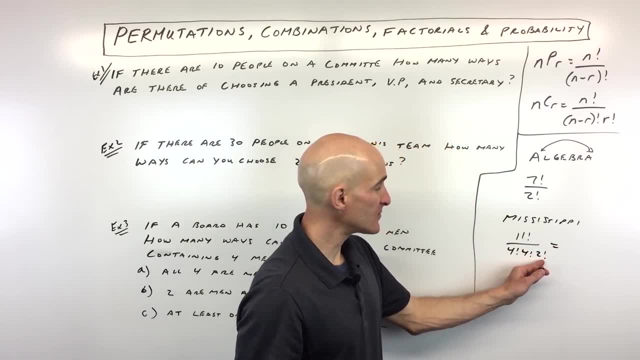 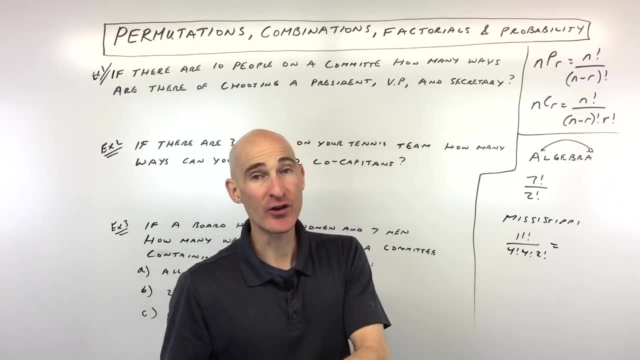 four times three times two times one, again another four times three times two times one times two times one, And just simplify them and then you can divide And that's going to be the number of distinct or different or unique. however you want to say that permutations of all the letters in the word Mississippi, Let's 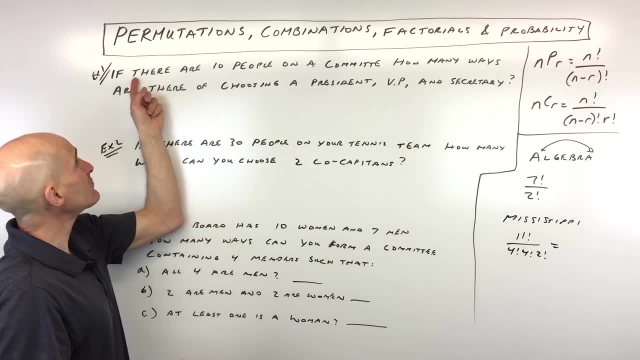 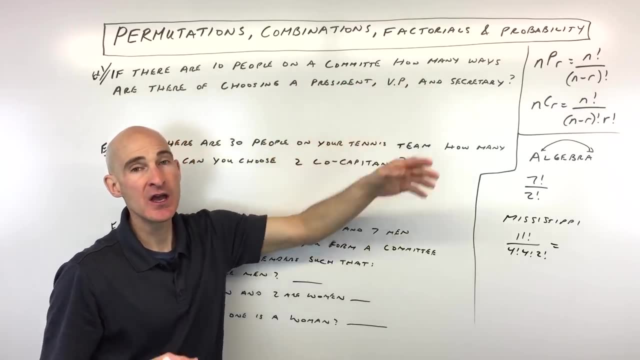 go into some word problems. see if you can do these along with me here. It says: if there are 10 people on a committee, how many ways are there of choosing a president and vice president and secretary? Now, at this point we're just talking about the number of outcomes we're gonna get into. 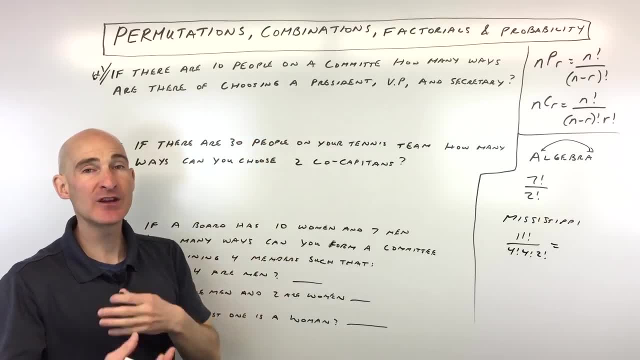 probability in just a little bit here, But first we want to find out how many different ways there are of choosing a president, vice president, secretary, out of the 10 people on a committee. Now the question that you want to really focus on is: is the? 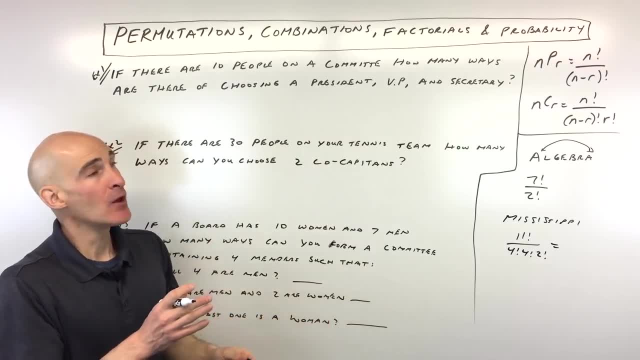 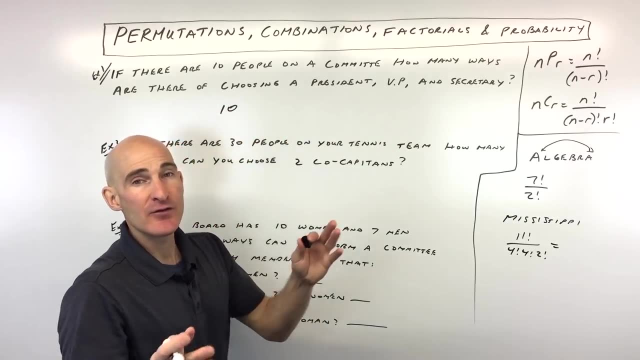 order important Or is the order not important? Well, if you were to take 10 people and you're going to basically pick three of them, right? If you change the order of those people, they're going to have a different job or a different. 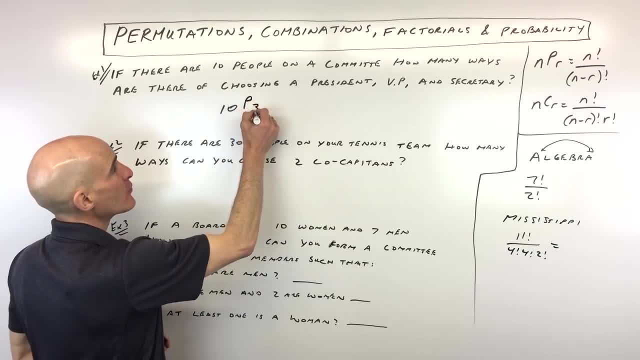 position. So the order is important. So this is going to be 10 permutation three, or 10 p three, or sometimes what I say is out of 10, you're picking three where the order matters. Now, if we use our formula here for permutations, you can see this is going to be 10 factorial over 10 minus three, which is seven. 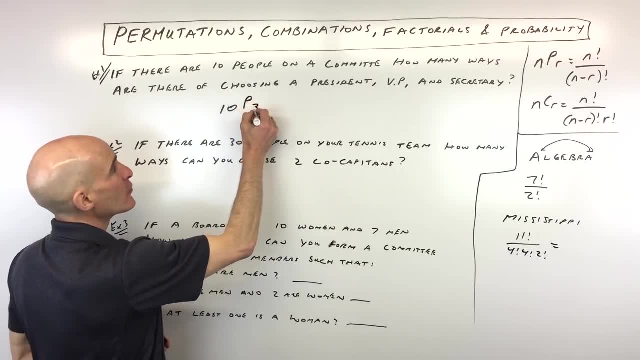 position. So the order is important. So this is going to be 10 permutation 3 or 10 P3, or sometimes what I say is out of 10, you're picking three where the order matters. Now, if we use our formula here for permutations, you can see this is going to be 10 factorial. 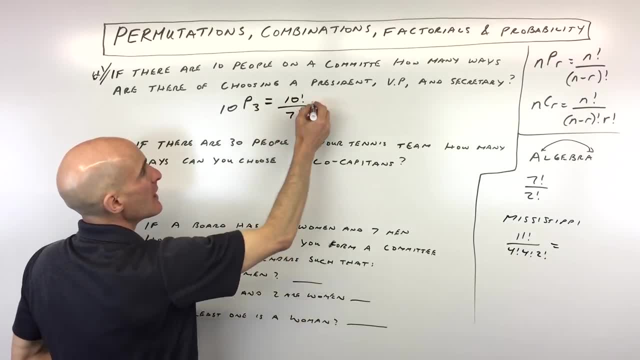 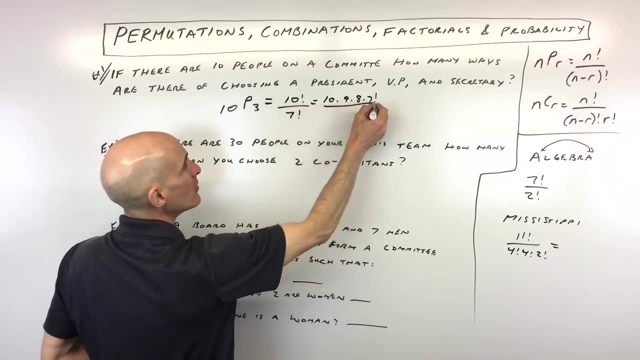 Over 10 minus three, which is seven factorial, And if we expand this out it's going to be 10 times nine times eight times seven, six, five, four, three, two, one. Or you could just write that seven factorial over seven factorial. You can see those are canceling. 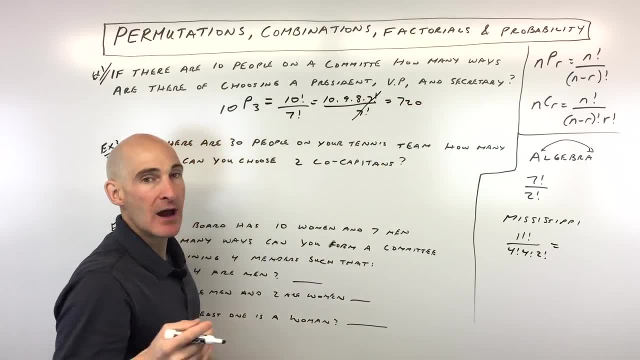 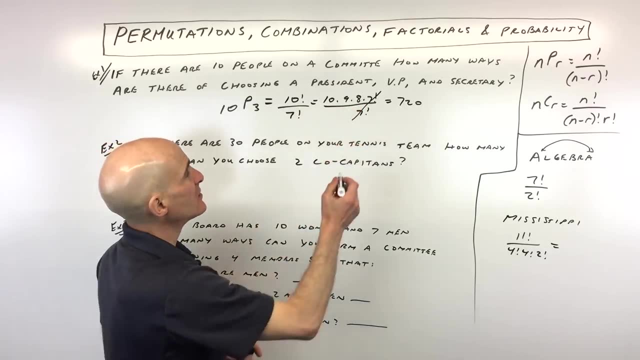 So it's really just going to be 720 different ways. Now, another way to do this is to use the multiplication counting principle or the fundamental counting principle, And you can see that there's just going to be 10 ways of choosing a president. right? But once you? 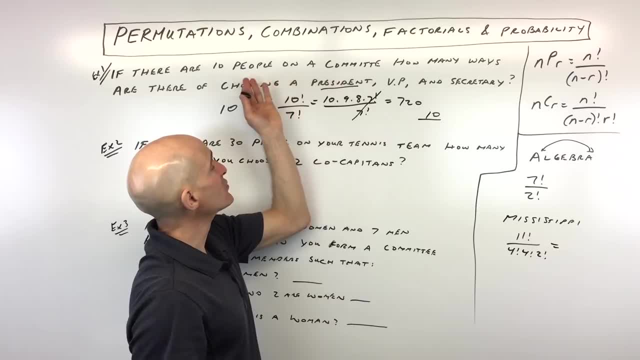 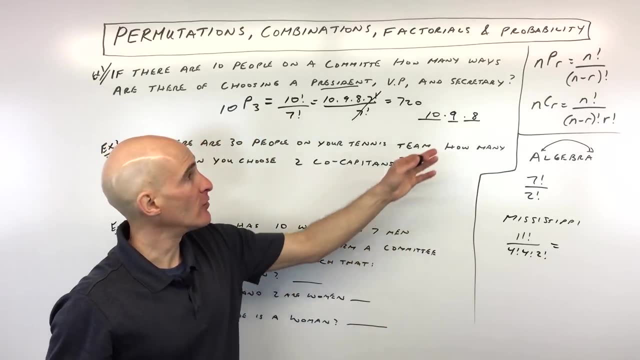 choose that president, there's only nine people left, You know, in this group, to choose the vice president, And then, once you choose those two people, there's only eight people remaining left to choose the final position, the secretary, And you can then use that multiplication counting principle or that fundamental counting principle. 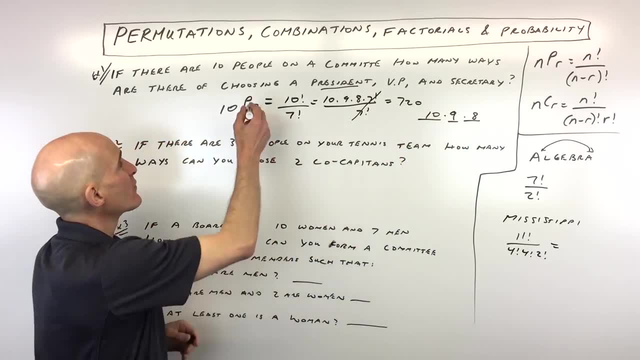 and multiply those together, You're going to get the same result. A lot of students prefer this method because it's just a kind of an easy way to think about it. You say, out of 10, you're picking three where the order matters, But for others this is a little. 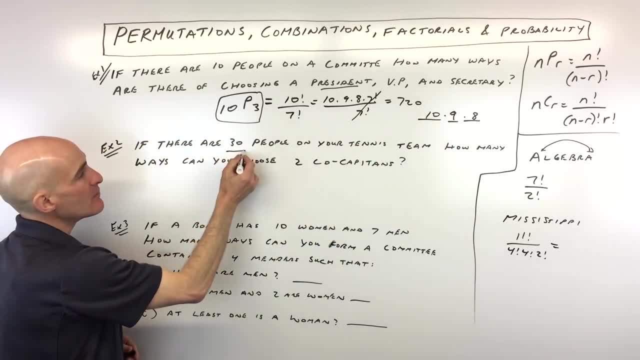 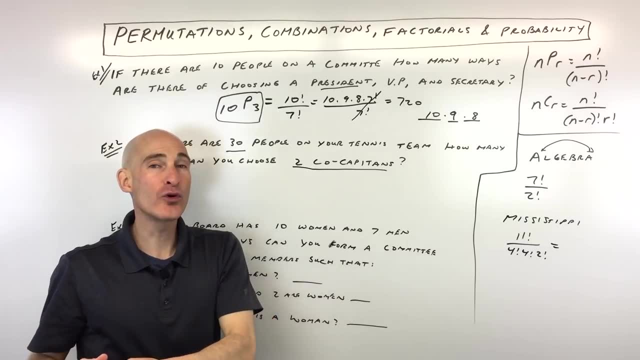 bit easier. So let's look at number two Now. it says: if there are 30 people on your tennis team, How many ways can you choose two co-captains? So my question is: do you think that the order is important or do you think the order is not important? Well, in this case, the order. 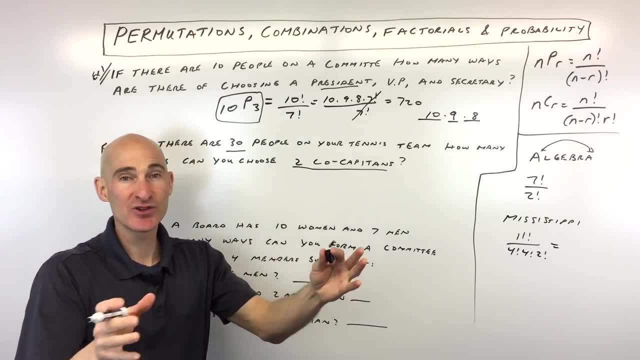 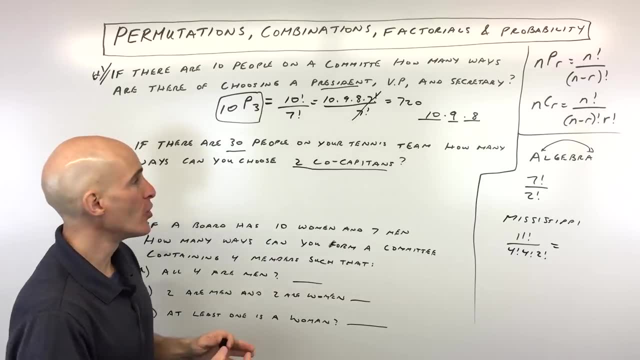 that doesn't matter, because if you take, you know this person and this person and you switch them, they're still going to be the same co-captains. It's not like they're going to have a different position, like one's the president, one's the vice president. No, they're. 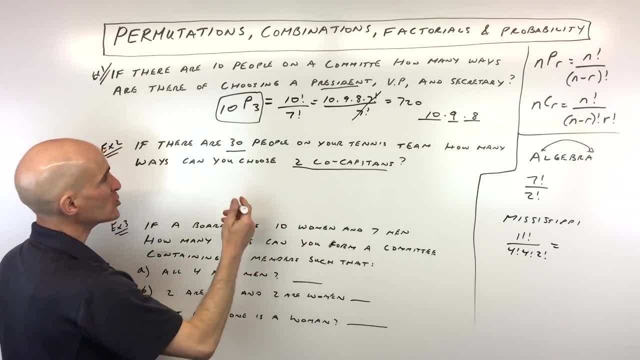 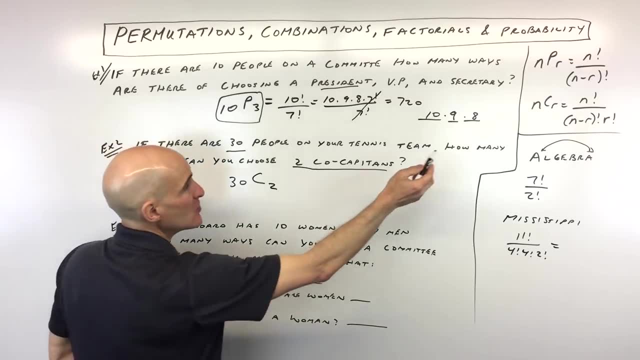 basically they're the same position, So it doesn't matter. you know in what order we choose them. So we're going to use combinations. So 30 combination two, or you could say out of 30, we're choosing two. I'm going to use the combination formula up here, which is: 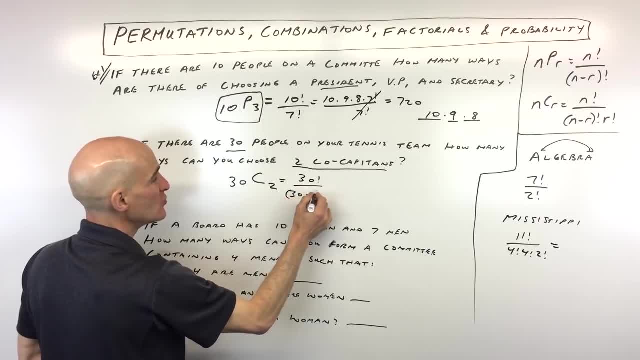 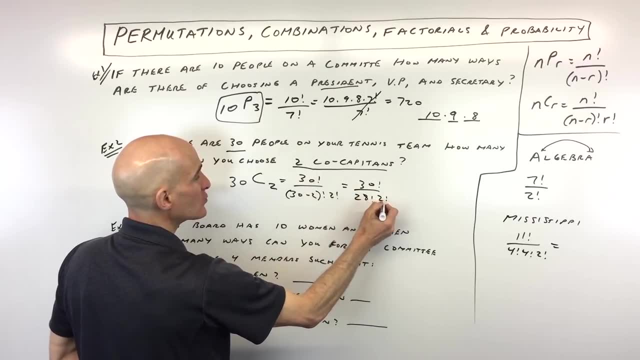 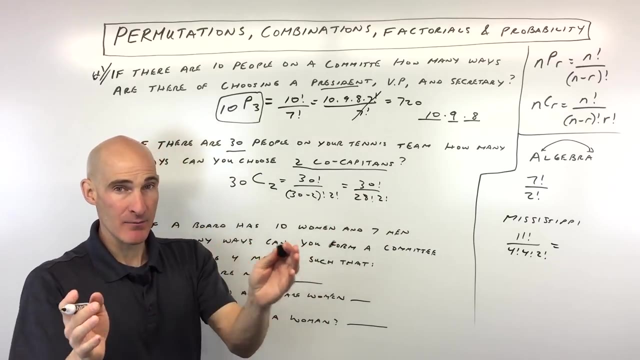 30 factorial over 30, minus two factorial, two factorial. So this is going to be a 30 factorial over 28 factorial, two factorial And again notice this, two factorial. what this is doing is it's dividing out those multiplicities like A and B, B and A. Those are the same. 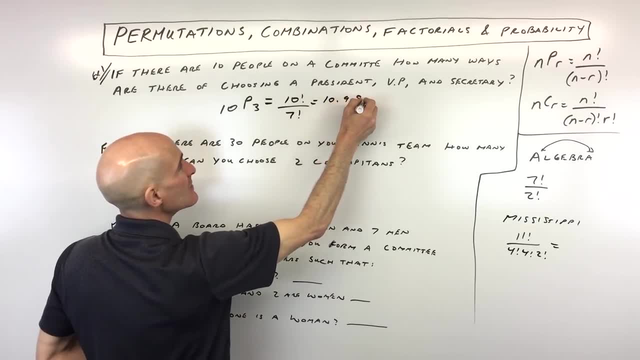 factorial And if we expand this out it's going to be 10 times nine times, eight times seven, six, five, four, three, two, one, or you could just write that seven factorial over seven factorial you can see those are canceling. So it's really just going to be 720. 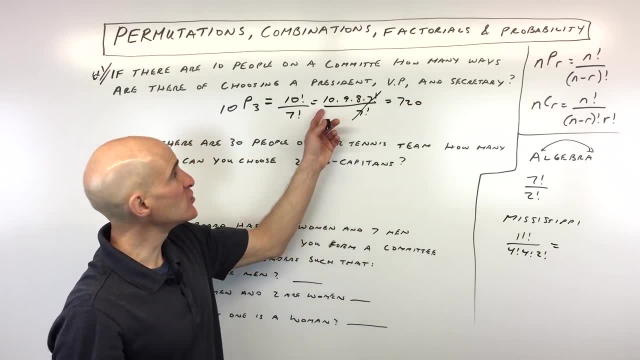 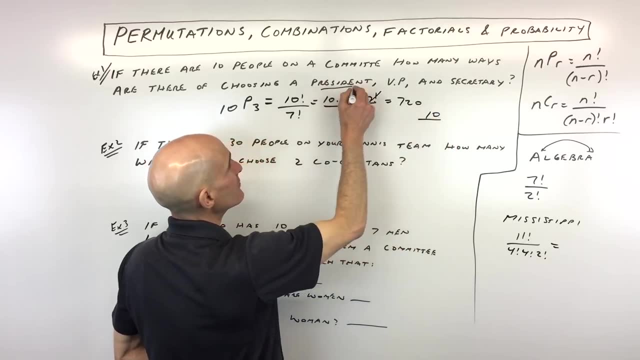 different ways. Now, another way to do this is to use the multiplication counting principle or the fundamental counting principle, And you can see that there's just going to be two people left in the group, and you can see that there's only nine people left in the group to choose the vice president. 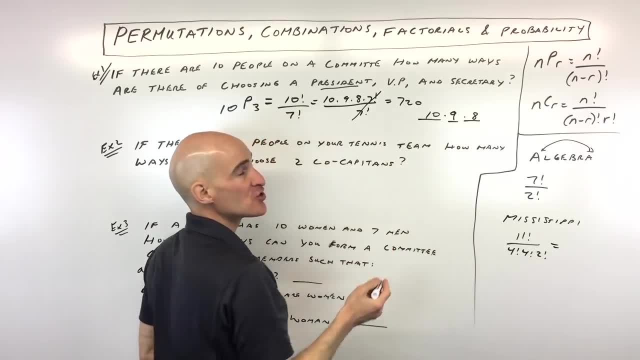 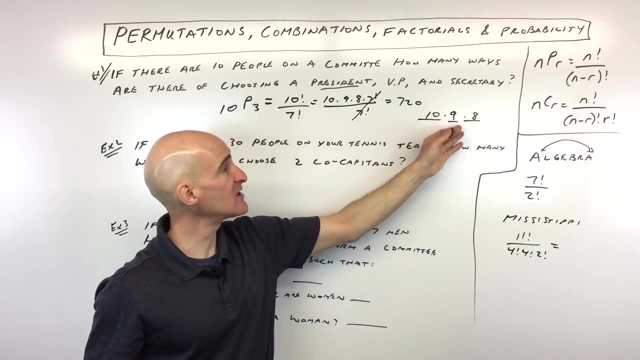 And then, once you choose those two people, there's only eight people remaining left to choose the final position, the secretary, and you can then use that multiplication counting principle or that fundamental counting principle and multiply those together. you're going to get the same. 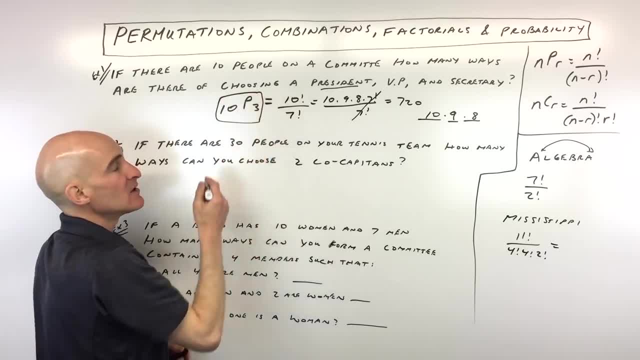 result. A lot of students prefer this method because it's just a kind of an easy way to think about it. you say, out of 10, you're picking three where the order matters, But for others this is a little bit easier. 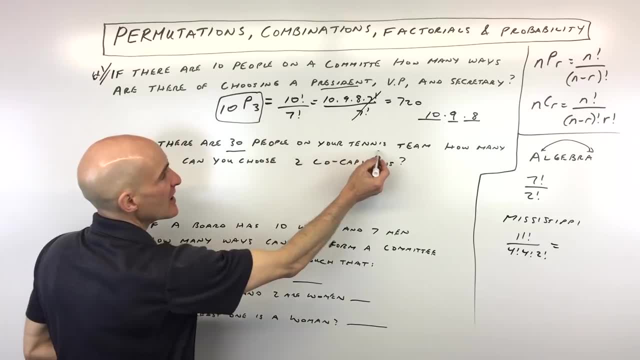 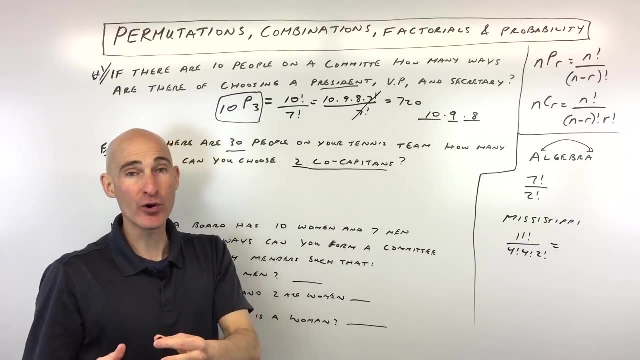 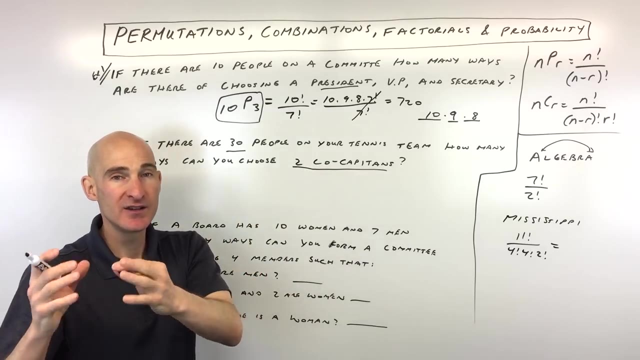 So let's look at number two. It says: if there are 30 people on your tennis team, how many ways can you choose two co captains? So my question is: do you think that the order is important Or do you think the order is not important? Well, in this case, the order it doesn't matter, Because if you take, you know this person and this. 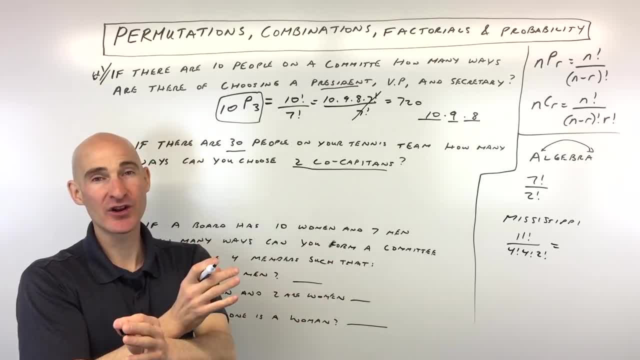 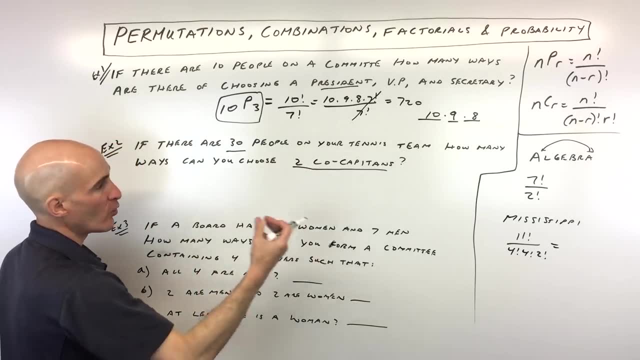 person and you switch them, they're still going to be the same co captains. it's not like they're going to have a different position, like one's the president, one's the vice president. No, they're basically they're the same position, So it doesn't matter. you know in what order we choose them, So we're. 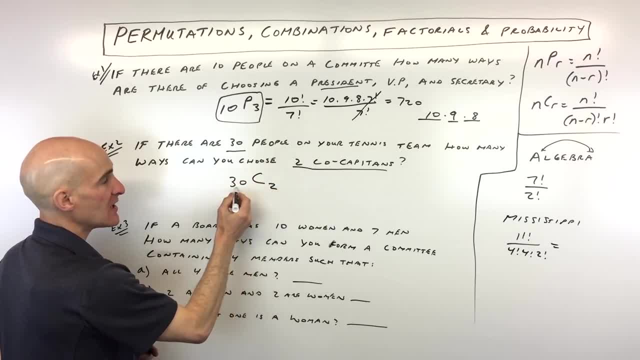 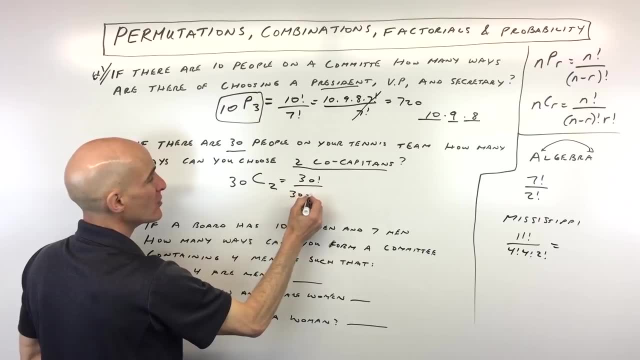 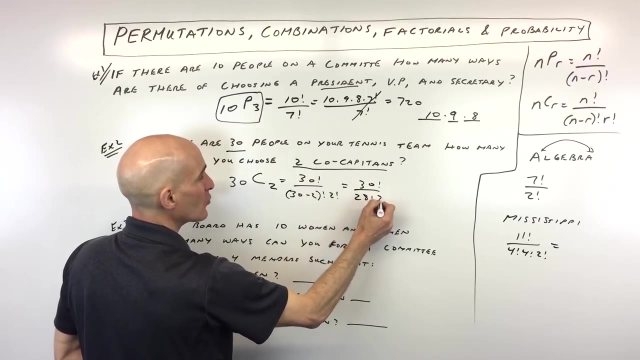 going to use combinations, So 30 combination two, or you could say out of 30, we're choosing two. I'm going to use the combination formula up here, which is 30 factorial over 30, minus two factorial, two factorial. So this is going to be 30 factorial over 28 factorial, two factorial And- again notice this- two. 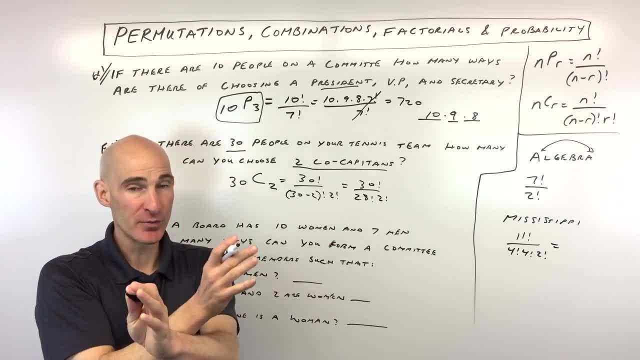 factorial. what this is doing is it's dividing out those multiplicities like A and B, B and A. those are the same two people that are the co captains. you don't want to double count those, So that's why we're dividing them. 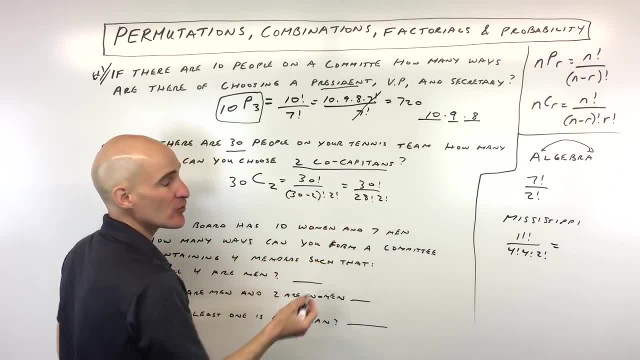 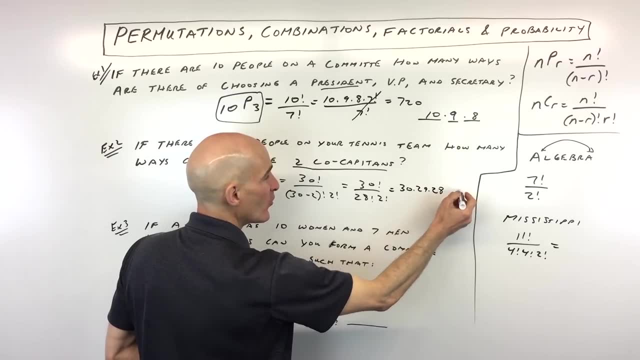 two people that are the co-captains. You don't want to double count those, So that's why we're dividing those out. So you can see, this is going to be 30.. Times 29,, times 28,, 27,, all the way down to one right. So 28 factorial, And here we've. 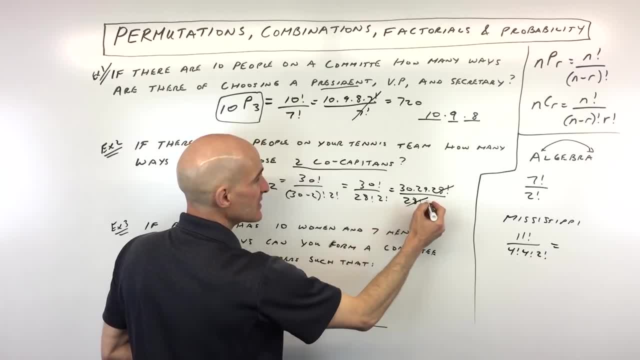 got 28 factorial. Notice that those are the same. Those are canceling over two times one And you can see two goes into 30, 15 times. So we really just have 15 times 29.. And that's going to be the number of ways that you could choose those two co-captains. 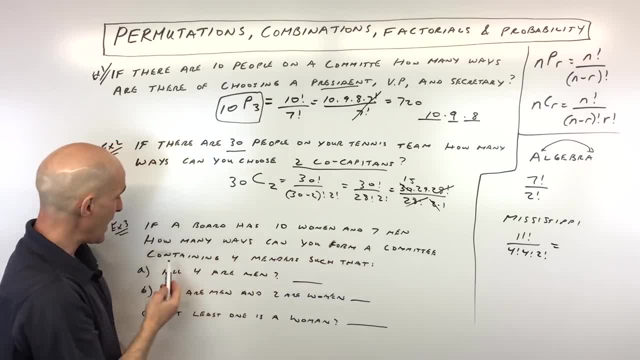 So let's look at number three. It says: if a board has 10 women and seven men, how many ways can you form a committee that contains four members? Okay, so this is important. Four members such that all four are men. Okay, so what do you think on that one? So all four men. I, So all four are men, all. 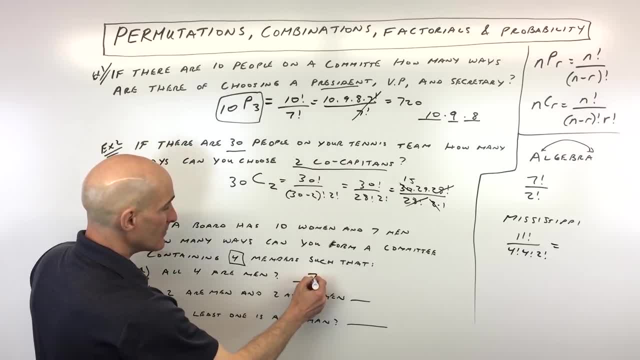 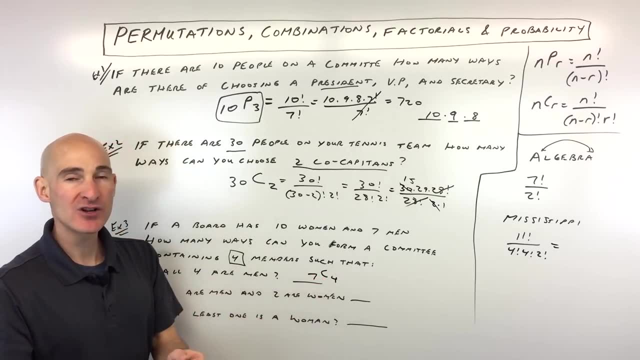 women. Well, you can see there's seven men. So out of seven, we're going to be choosing four, and I'm using the combination seven, combination four, because the order doesn't really matter. It's just a committee, It's not like they have a, you know, president, vice. 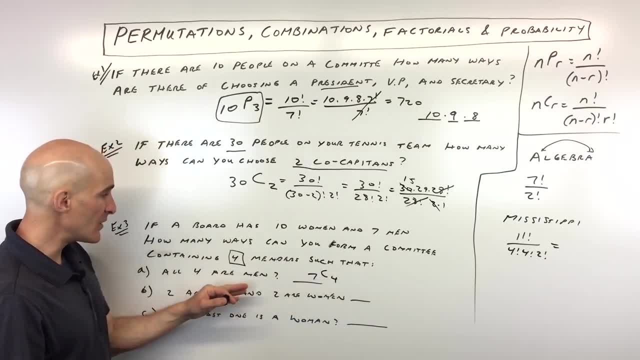 president, or first place, second place, third place, Order's not important, And you can simplify that by using the combination formula hereENE colocar. Did you see是 are men and two are women. Well, again, what you do is: you take how many there are in that group. 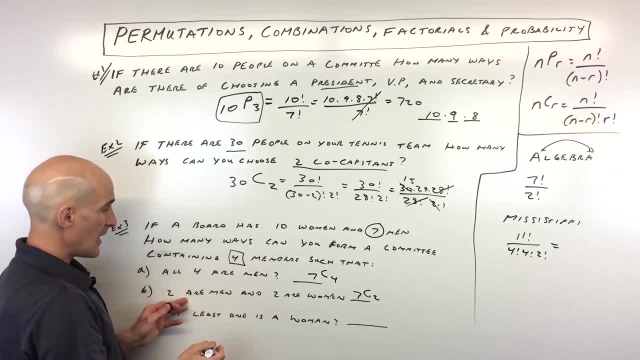 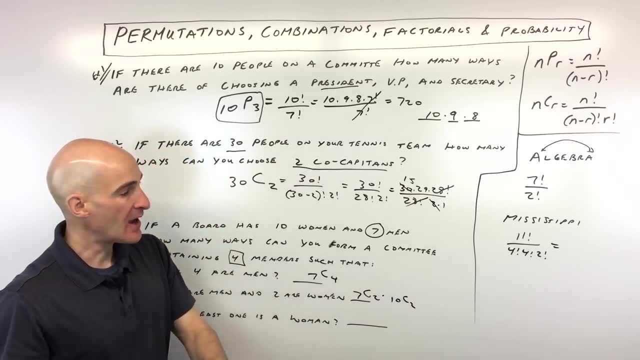 There's seven men but we're choosing two and there's two that are women. So out of the 10 women, we're choosing two and we're going to multiply those together. So we're using that fundamental counting principle. We're basically saying: you know how many outcomes there are in. 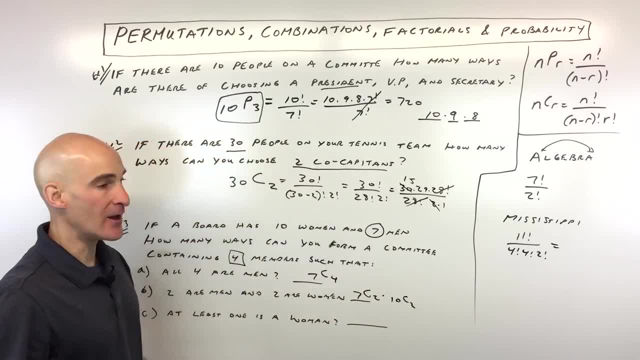 this group times how many outcomes there are in this group and we're multiplying them together. Okay, the last one, this one's a little bit more challenging. It says: at least one is a woman, So at least one. So at least means one could be a woman, two could be, you know, women. three: 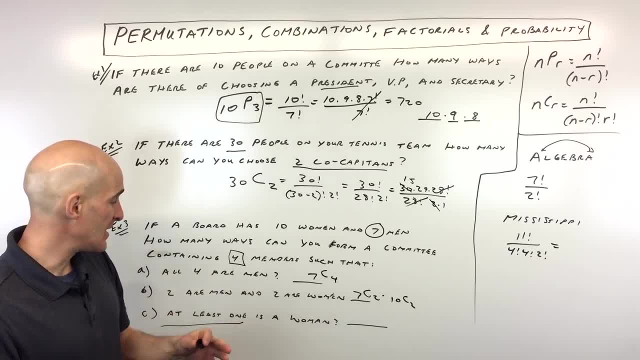 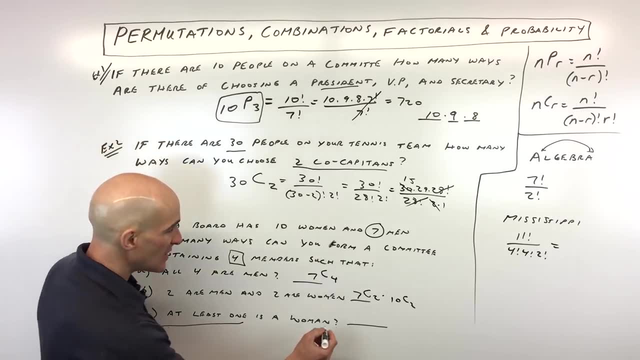 or all four. Now we could do it, you know, by individually and add them all up. But another way to do this: when you see this phrase at least one, you might want to take notes on this one, at least one. what you do is you take the total minus none. Okay, what does that mean? It sounds. 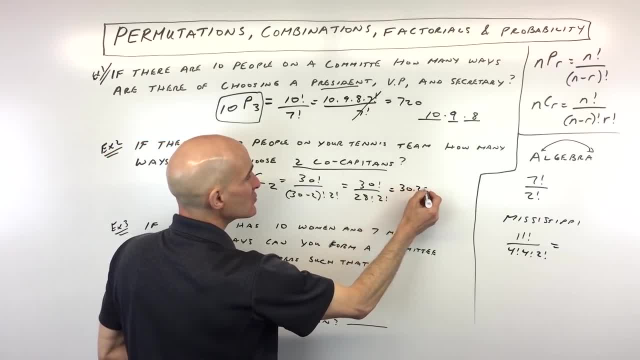 those out. So you can see this is going to be 30 times 29 times 2827, all the way down to one right. so the 28 factorial- And here we've got 28 factorial, notice that those are the same. those are canceling over two times one And you can see two goes into 3015 times. so we really just have 15 times. 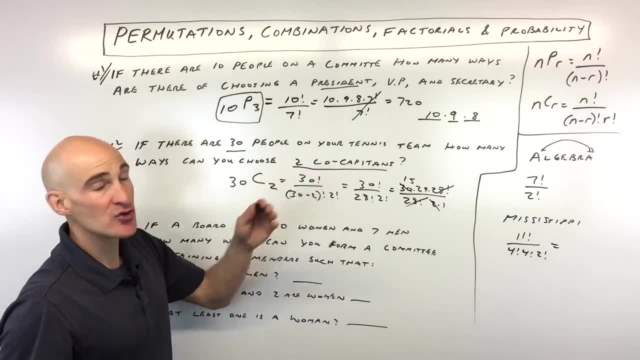 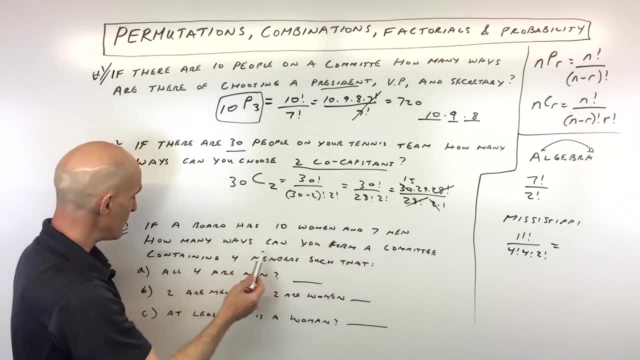 29.. And that's going to be the number of ways that you could choose those two co captains. So let's look at number three. it says: if a board has 10 women and seven men, how many ways can you form a committee that contains four members? okay, so this is important. four members such that all four are men. Okay, so what do you think on that one? So all four are men. 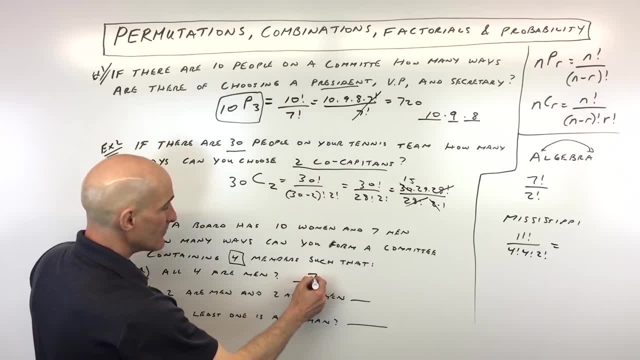 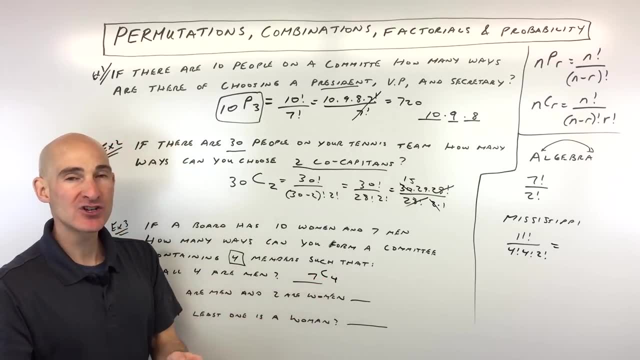 Well, you can see there's seven men. So out of seven we're going to be choosing four, and I'm using the combination seven, combination four, because the order doesn't really matter. It's just a committee. It's not like they have a, you know, president, vice president, or first place, second place, third place, the order is not important And you can simplify that using the combination formula here. 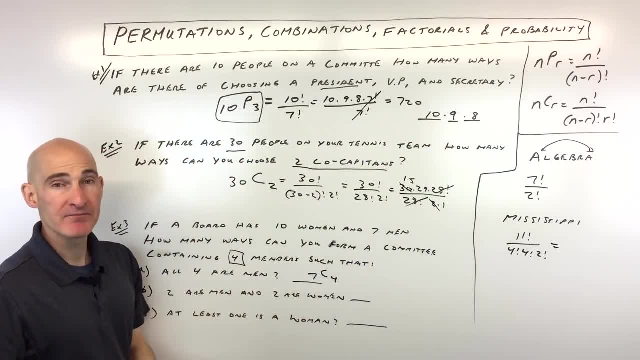 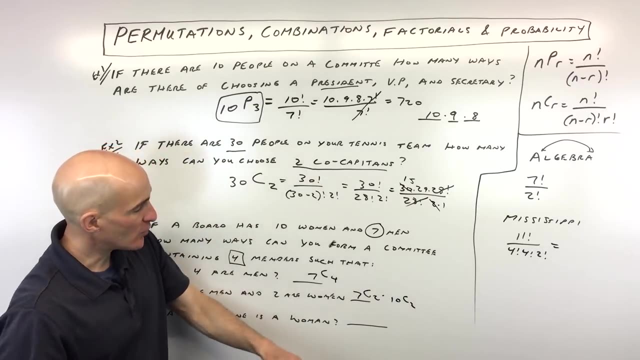 Now letter B. it says two are men and two are women. Well, again, what you do is you take how many there are in that group. there's seven men, but we're choosing two And there's two that are women. So out of the 10 women, we're choosing two and we're going to multiply those together. So we're using that fundamental counting principle. We're basically saying: you know how many outcomes there are in this group, times how many outcomes there are in this group and we're multiplying them together. Okay, the last one. this is a little bit more challenging. It says at least one is a woman. So at least one. So at least means 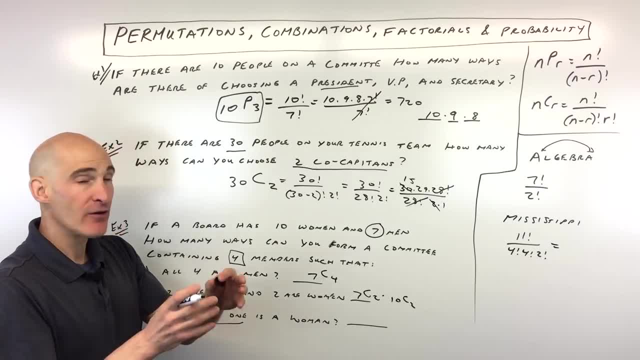 one could be a woman, two could be, you know, women, three or all four. Now we could do it, you know, by individually and add them all up. But another way to do this: when you see this phrase at least one, you might want to take notes on this one, at least one. what you do is you take. 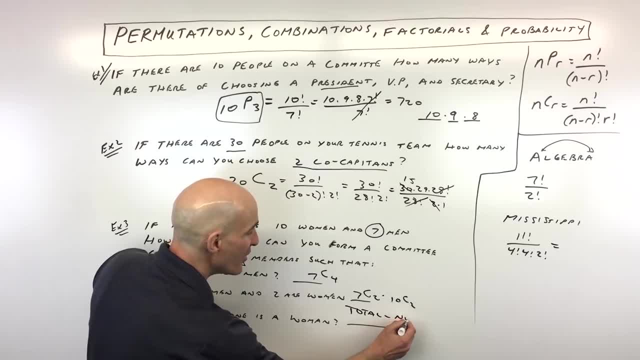 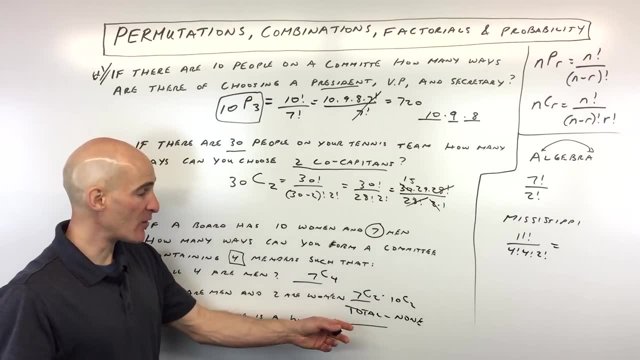 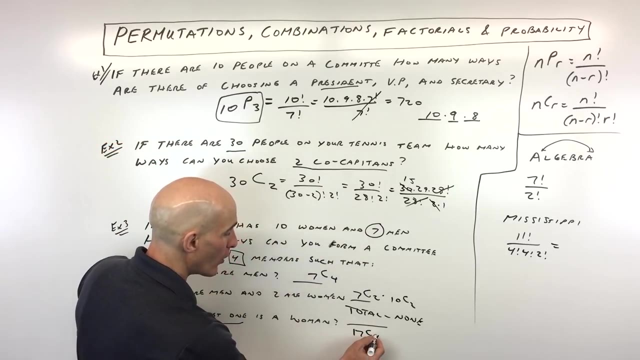 the total minus none. Okay, what does that mean? It sounds a little cryptic, right? Well, the total means: how many ways can you find, you know, how many ways can you make a committee of four people out of 17 people? Well, that's going to be 17. choose four minus the committees that have no. 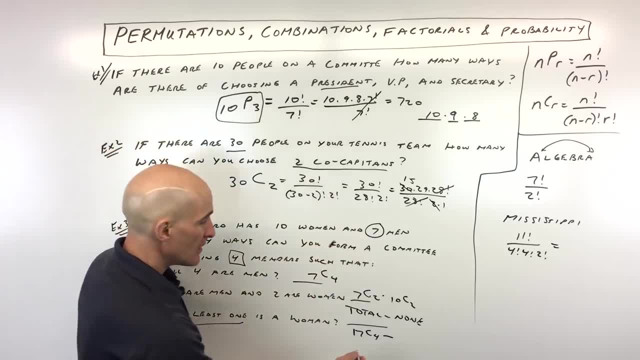 women on them. Well, the committees that have no women on them would be seven: choose four. That would be out of the seven men, you're choosing four. Now, another way that students like to do this too is you could say: well, out of the seven men, you're choosing four times out of the 10. 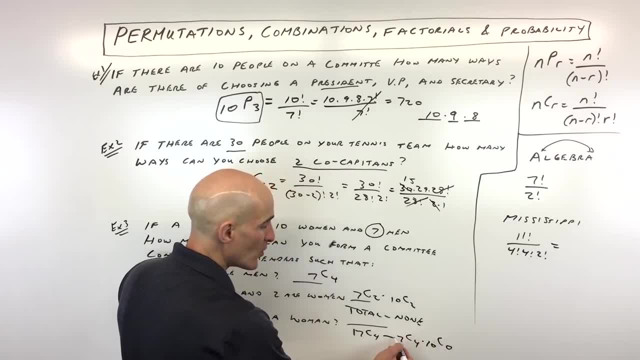 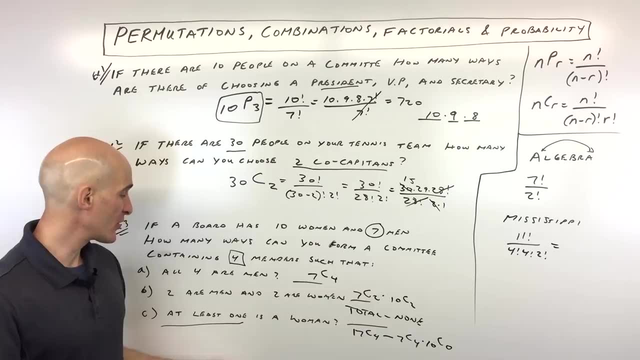 women, you're choosing zero, But 10 choose zero, just one. So one times anything is itself, But this is kind of like a little quicker way of doing it. Okay, so let's look at some examples of how we're doing this problem. Do the total minus no women. 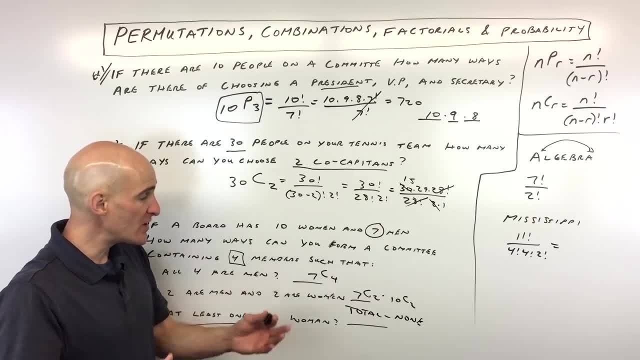 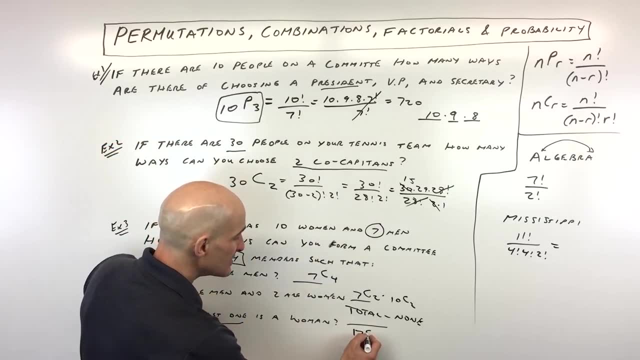 a little cryptic, right. Well, the total means: how many ways can you find, you know, how many ways can you make a committee of four people out of 17?? Well, that's going to be 17. choose four minus the committees that have no women on them. Well, 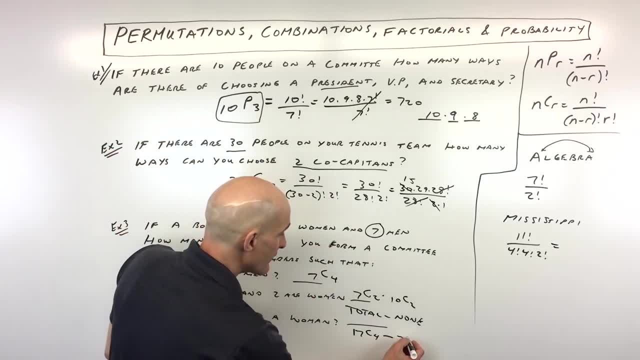 the committees that have no women on them would be seven, choose four. That would be out of the seven men, you're choosing four. Now, another way that students like to do this too is you could say: well, out of the seven men you're choosing four times, out of the 10 women you're choosing, 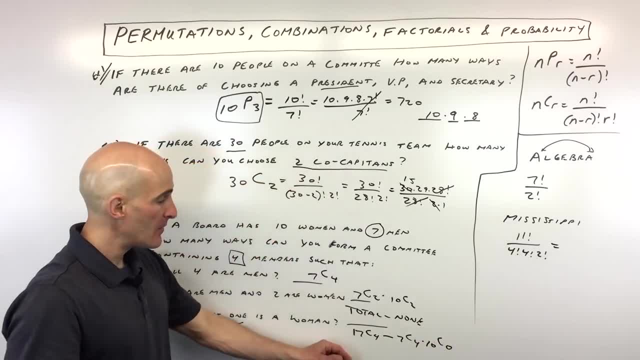 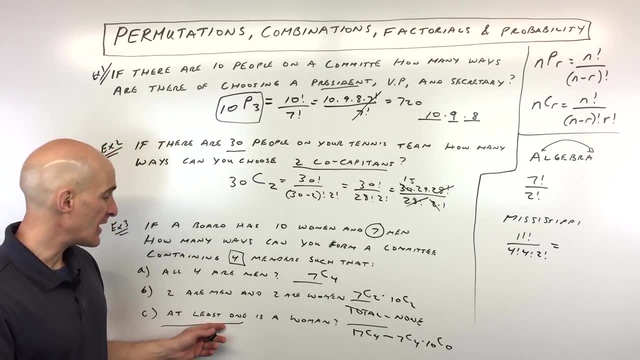 zero, but 10 choose zero, just one. So one times anything is itself. But this is kind of like a little quicker way of doing this problem. Do the total minus no women. it would be all the committees that had at least one or two or three, or all four. 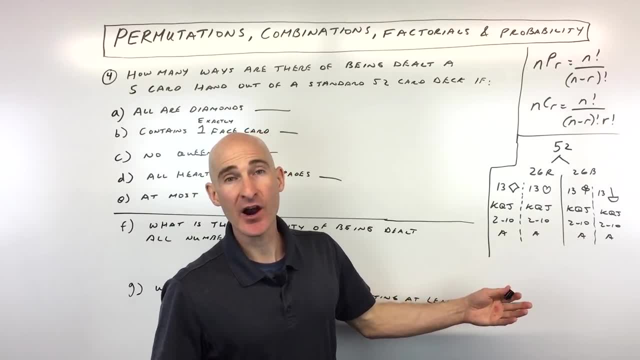 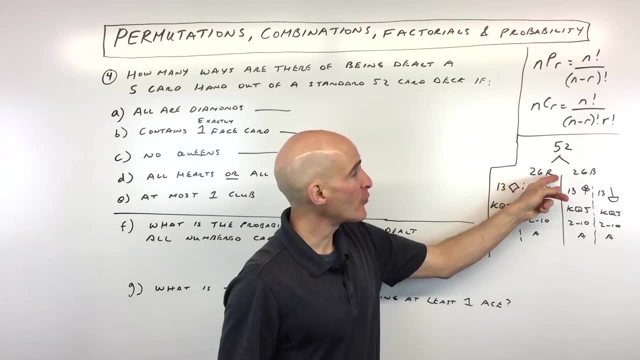 on them. Okay, now some examples with cards, playing cards, a standard 52 card deck. If you're not familiar, it's pretty easy to understand. There's 52 cards in the deck. half are red and half are black. So 26 red, 26 black. and then it's broken down into what they call suits, four suits: 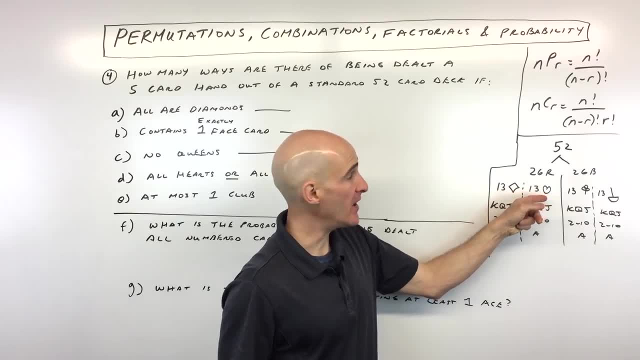 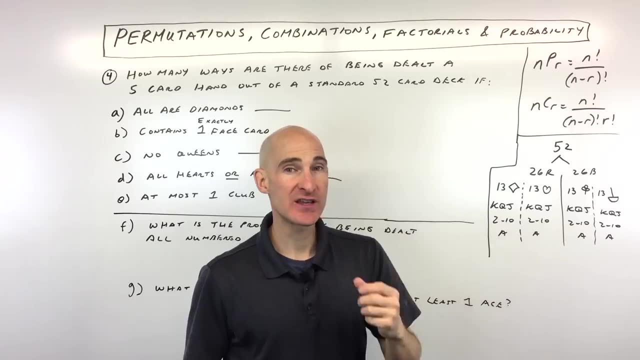 There's 13 diamonds and 13 hearts- These are red. and there's 13 clubs and 13 spades. These are four suits. There's a king, a queen and a jack. They call these face cards because they have a. 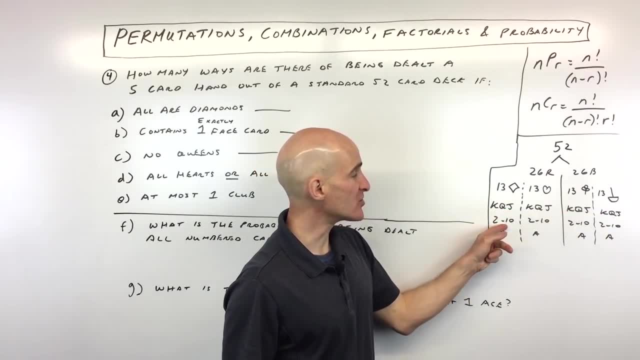 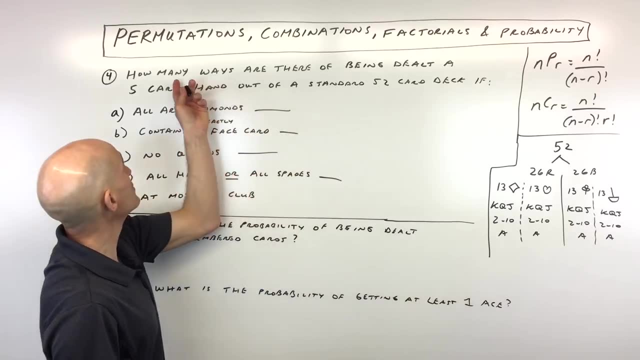 face on them, Okay, And each of the different suits. and then there's numbered cards, two through 10 in each of the four suits, And then each suit has one ace. Okay, So let's go into some examples here. It says how many ways are there of being dealt a five card hand out of a standard 52 card. 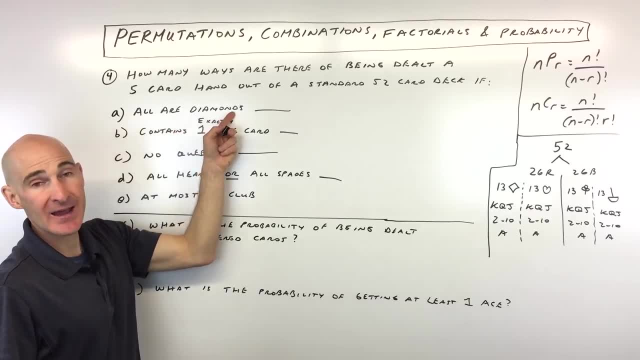 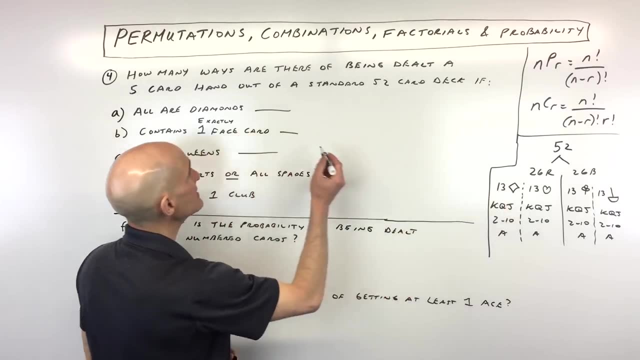 deck if all the cards are diamonds, Okay, So we're trying to figure out how many ways you could be dealt all diamonds. Well, the key is you say: well, how many diamonds are there? There's 13 diamonds and we're choosing five, or you could say 13 combination five. Now it doesn't. 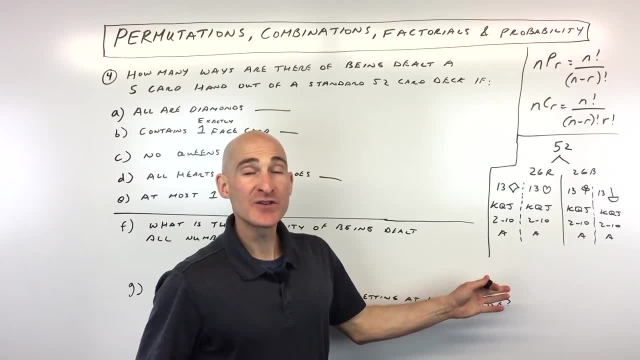 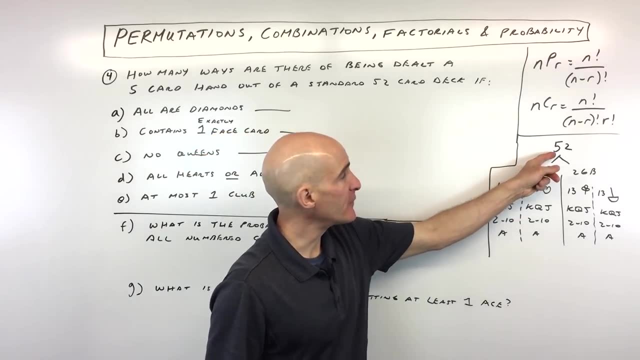 would be all the committees that had at least one or two or three or all four on them. Okay, now some examples for, with cards, playing cards, a standard 52 card deck. if you're not familiar, it's pretty easy to understand. there's 52 cards in the deck. half are red and half are black, So 26. 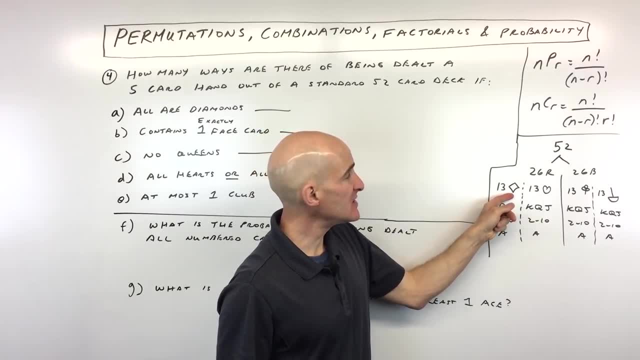 red, 26 black, and then it's broken down into what they call suits. for suits, There's 13 diamonds and 13 hearts. These are red. And then there's 13 clubs and 13 spades. these are red. And then there's 13. 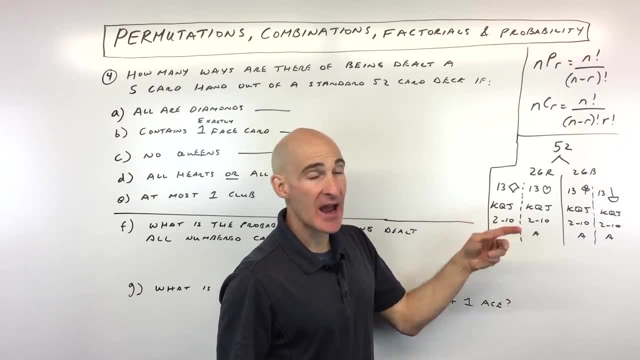 clubs and 13 spades. These are red. And then there's 13 clubs and 13 spades. And then there's 13 clubs and 13 spades- These are black. And then there's a king, a queen and a jack. they call these face cards that because 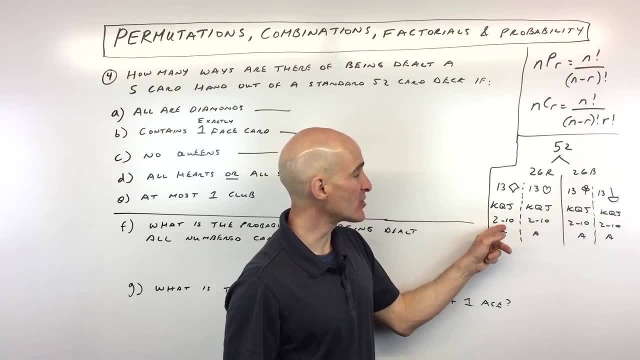 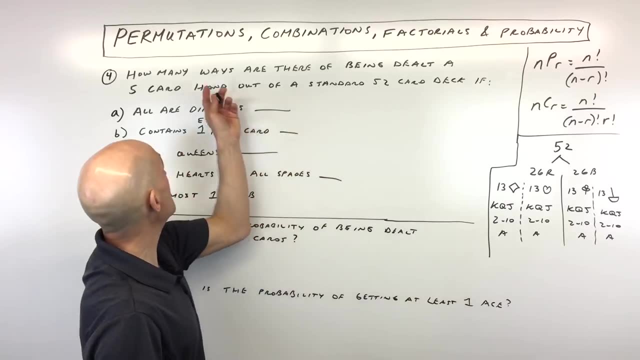 they have a face on them, okay, in each of the different suits. And then there's numbered cards, two through 10 in each of the four suits, And then each suit has one ace. Okay, so let's go into some examples here. It says: how many ways are there of being dealt a five card hand out of a standard 52? 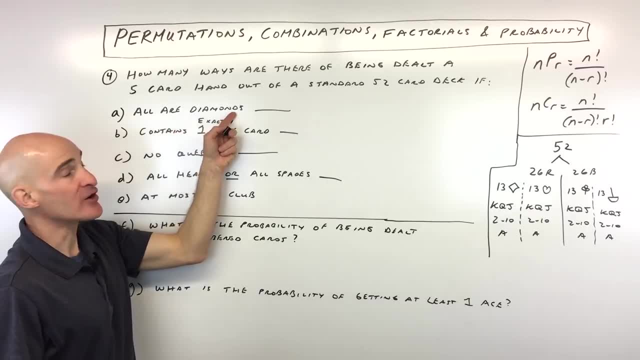 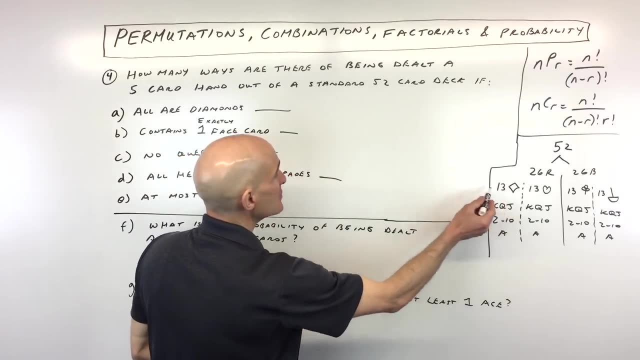 card deck if all the cards are diamonds, Okay, so we're trying to figure out how many ways you could be dealt all diamonds. Well, the key is you say: well, how many diamonds are there? there's 13 diamonds And we're choosing five. 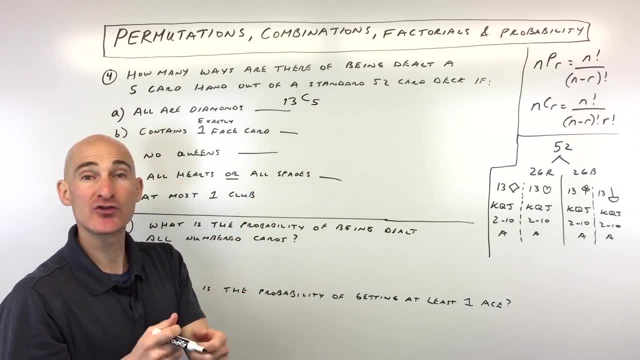 or you could say 3013 combination five. Now it doesn't matter which way you're dealt the cards, because you can shuffle them up in your hand once you get them. So that's why we're using the common combinations and not the permutations. So this one's just 13 C five. how many ways are? 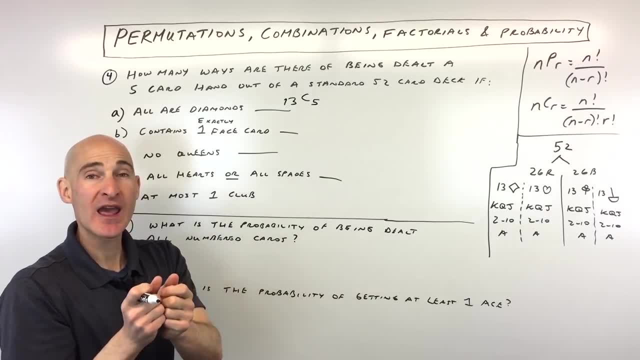 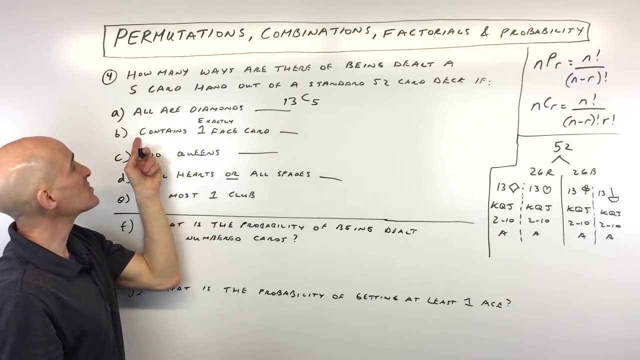 matter which way you're dealt the cards, because you can shuffle them up in your hand once you get them. So that's why we're using the common combinations and not the permutations. So this one's just 13 C5.. How many ways are there of getting a five card hand that contains exactly? 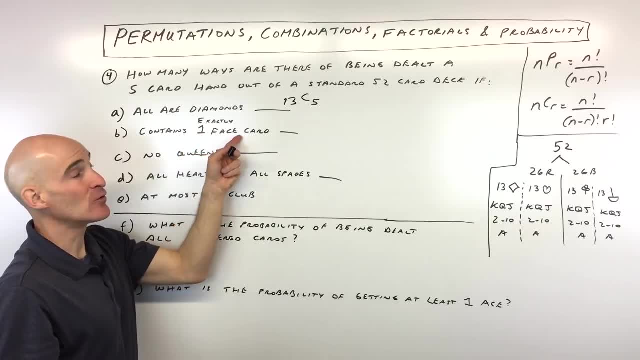 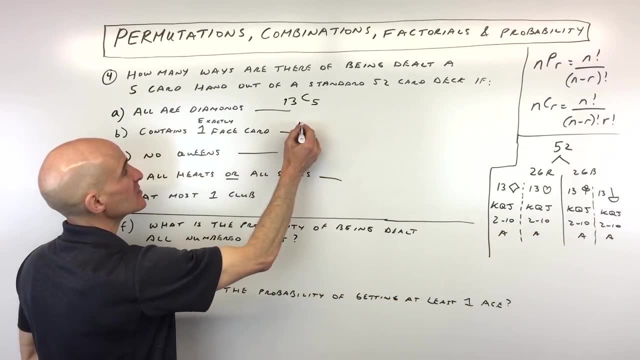 there of getting a five card hand that contains exactly one face card. Okay, so we look at the face cards. you can see that there's three, six, nine, 12 face cards. so that's going to be 12, choose one. see exactly one face card, But then the remaining cards. 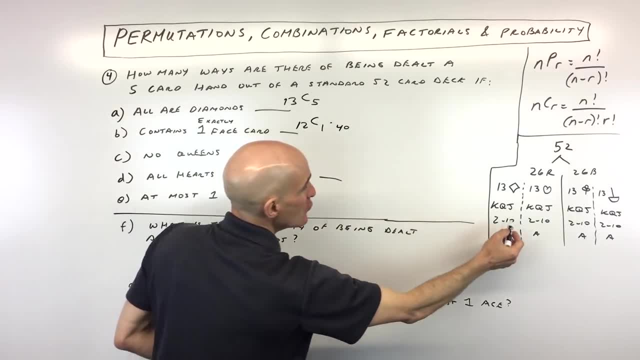 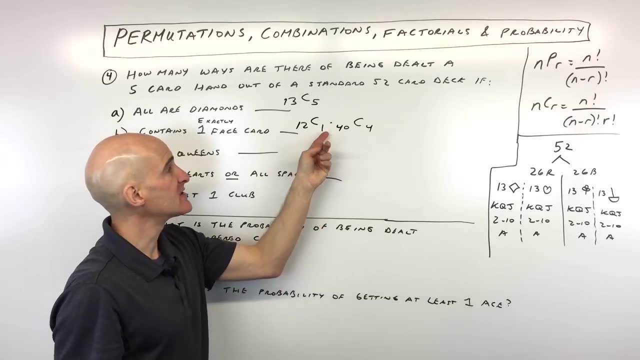 there's 40 cards that are not face cards, because 52 minus 12,, which is 40. And we're choosing four. So one way to think about this is: the first number is: how many is in that group? The second number is: 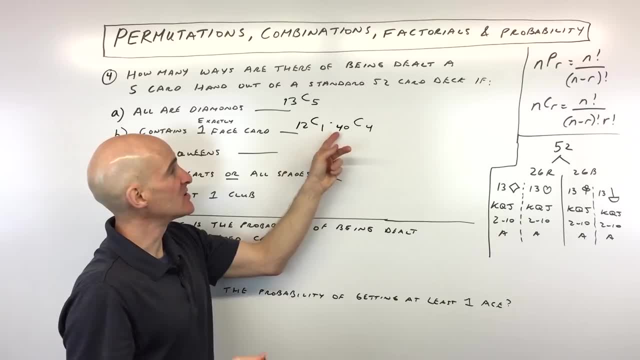 how many that you're. you're choosing out of that group And then you can see here the 12 and the 40. that adds up to 52, the one in the four adds up to our five card hand. The next one, let's say you: 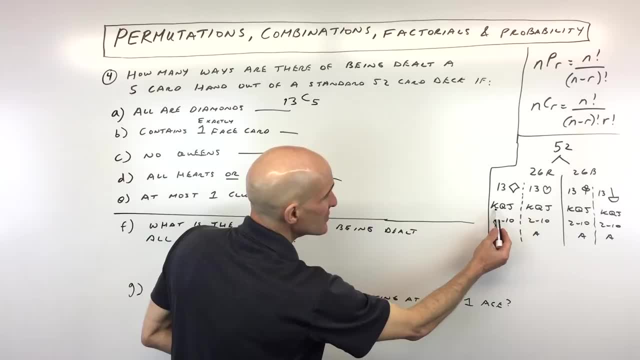 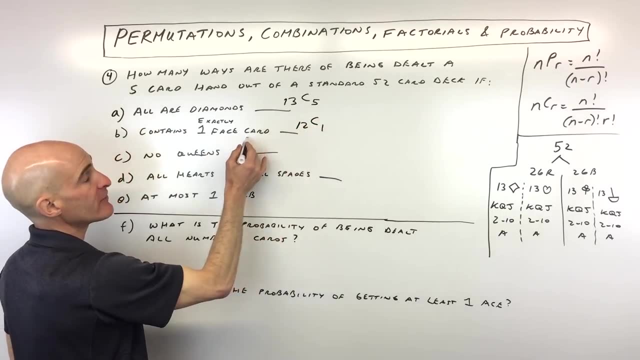 one face card. Okay, So we look at the face cards. You can see that there's three, six, nine, 12 cards. You can choose one. see exactly one face card, But then the remaining cards: there's 40. 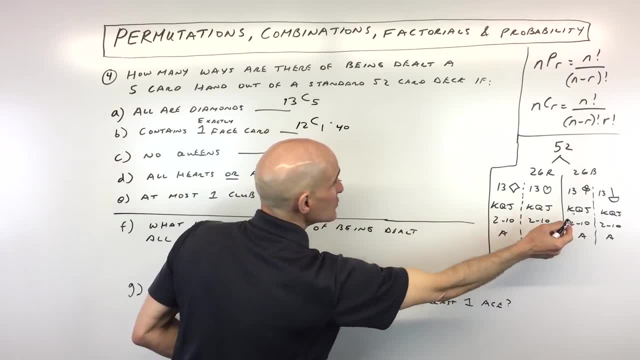 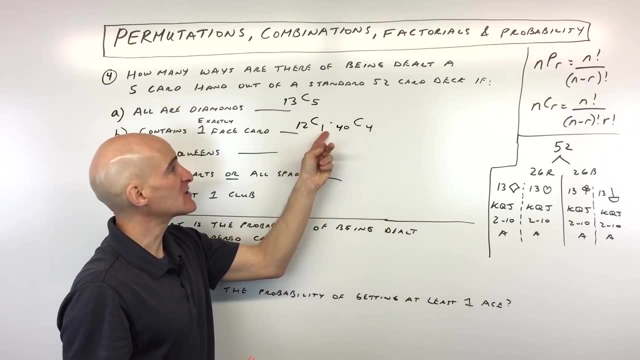 cards that are not face cards, because 52 minus 12, which is 40, and we're choosing four. So one way to think about this is: the first number is how many is in that group. The second number is how many that you're choosing out of that group, And then you can see here the 12 and the 40, that adds. 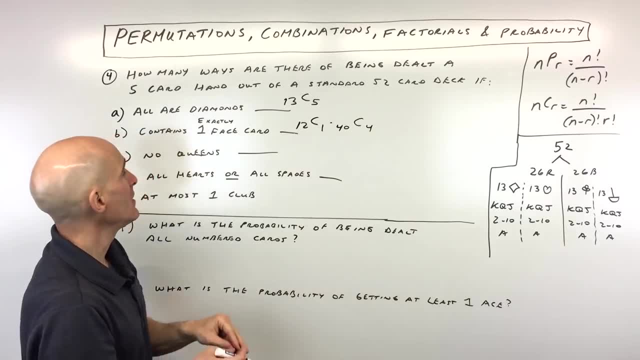 up to 52.. The one in the four adds up to our five card hand. The next one, let's say you want to find out the number of ways of not getting a queen. So you get five cards in your hand. None of them are. 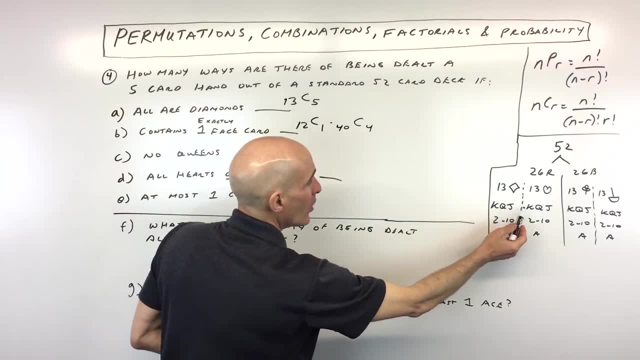 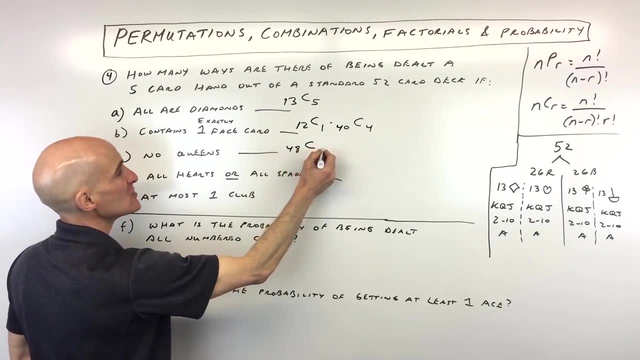 queens. Well, let's see, It looks like there's a queen, one, two, three, four queens. So if we take 52 minus four, that's going to be 48 cards that are not queens, and we're choosing five. 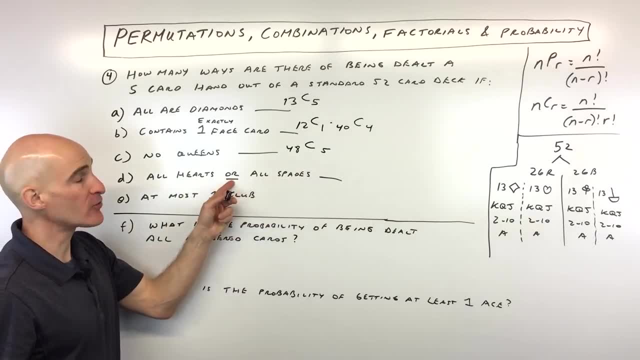 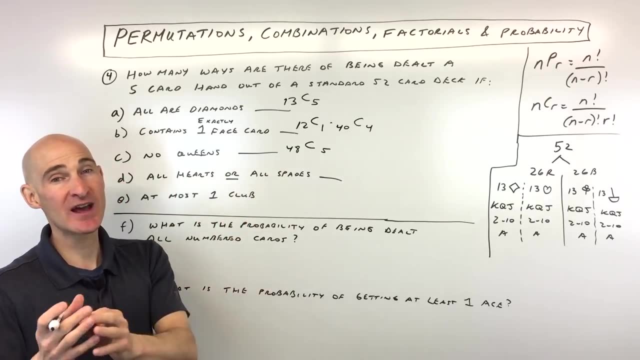 Okay, All our hearts or all our spades. Now, in math, when you see the word or, or means a union, it means both. It means like you're combining all these possibilities with all these possibilities, making sure not to double count any, But in this case you're not going to get a heart and a spade. 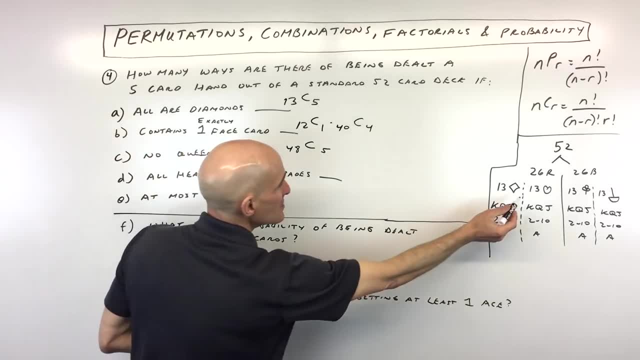 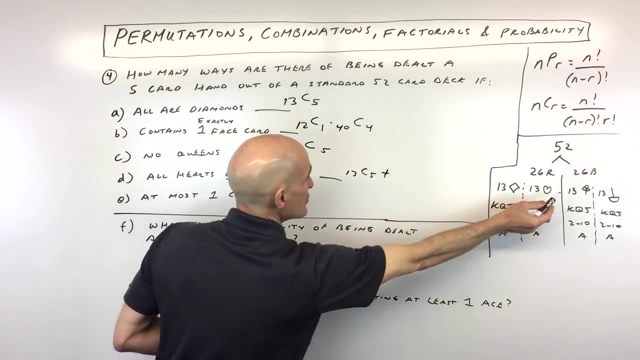 at the same time. So what's the number of ways of getting all hearts? Well, you can see, there's 13 hearts, So that's going to be 13,. choose five plus how many ways of they're getting all spades. Well, there's 13 spades over here, So that's going to be 13,. choose five. do those? 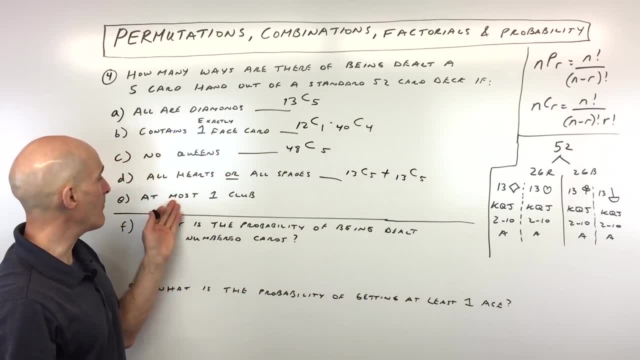 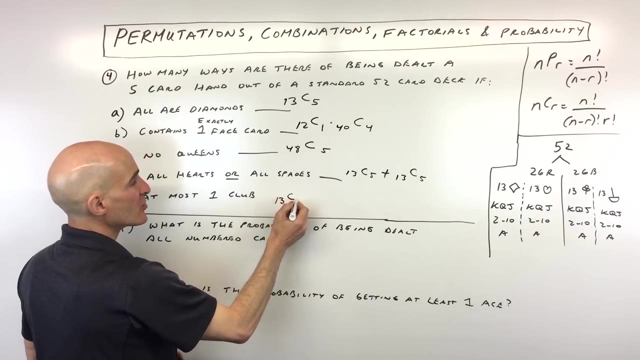 separately and then add them together. Okay, How about this last one? At most one club. So at most means that you could have zero clubs or one club. So let's figure out how many ways to get zero clubs. So you can see there's 13 clubs. So let's just say, out of the 13 clubs you're going to get, 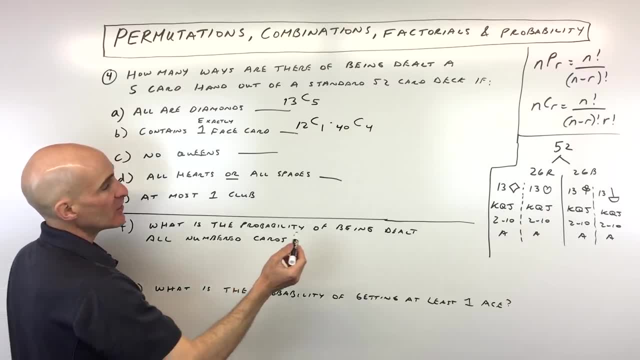 get five cards in your hand. none of them are queens. Well, let's see. it looks like there's a queen, one, two, three, four queens. So if we take 52 minus four, that's going to be 48 cards. 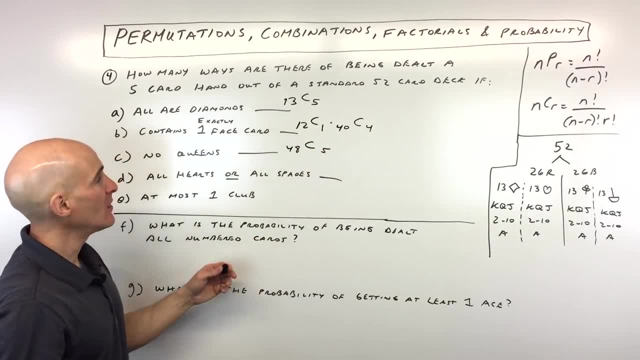 that are not queens and we're choosing five: Okay, all our hearts or all our spades. Now, in math, when you see the word or, or means a union, it means both. it means like you're combining all these possibilities with all these possibilities, making sure not to double count any, But in this 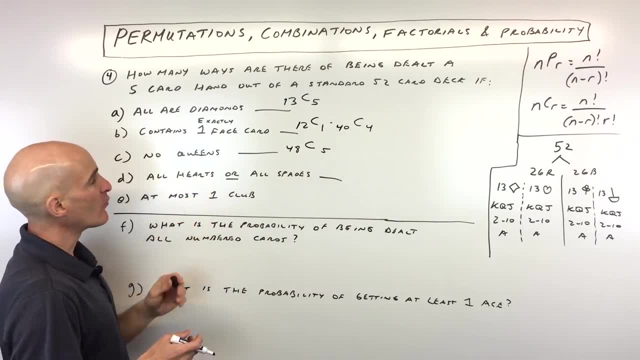 case, you're not going to get a heart and a spade at the same time. So what's the number of ways of getting all hearts? Well, you can see there's 13 hearts, So that's going to be 13,. 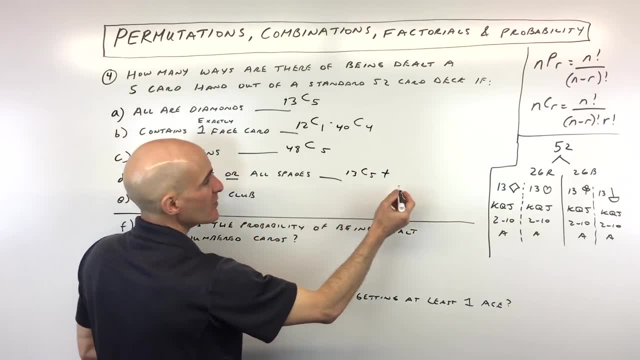 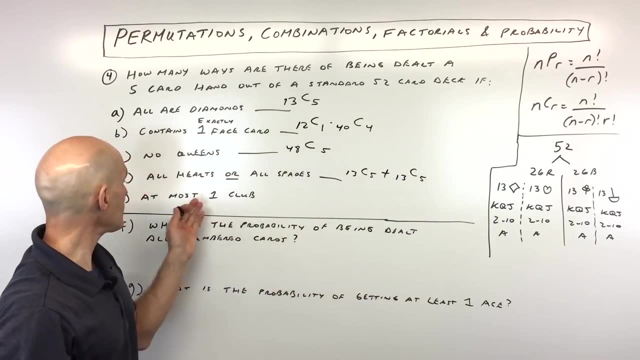 choose five plus how many ways are they're getting all spades? Well, there's 13 spades over here, So that's going to be 13,. choose five, do those separately and then add them together. Okay, how about this last one? at most, one club, So at most, means that you could have. 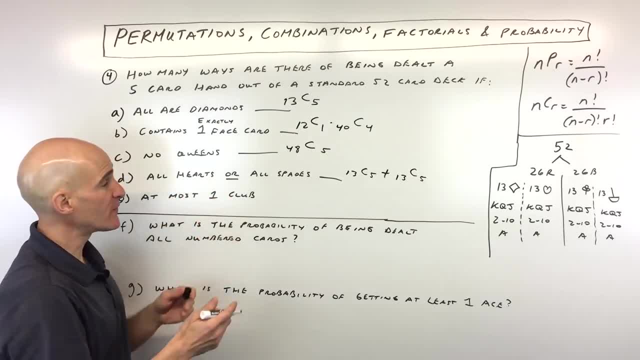 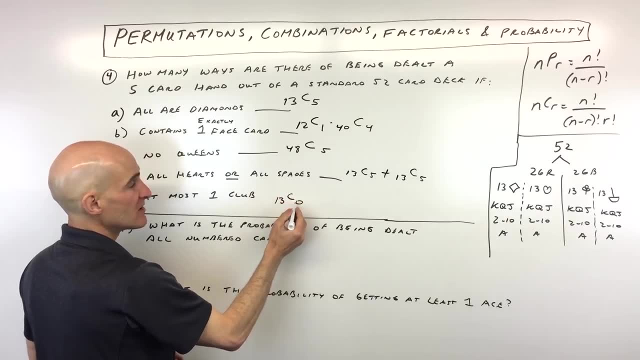 zero clubs or one club. So let's figure out how many ways to get zero clubs. So you can see there's 13 clubs. So let's just say, out of the 13 clubs you're going to get zero, but out of the 39 remaining cards that are not clubs, you're going. 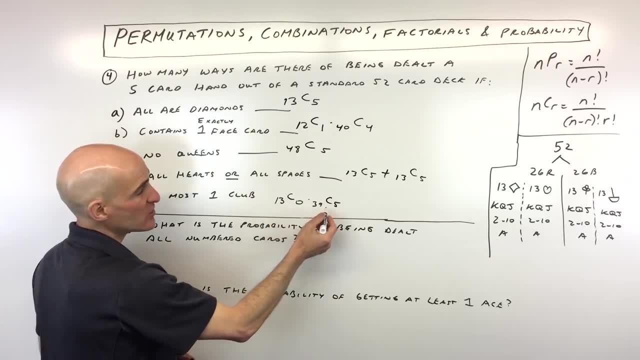 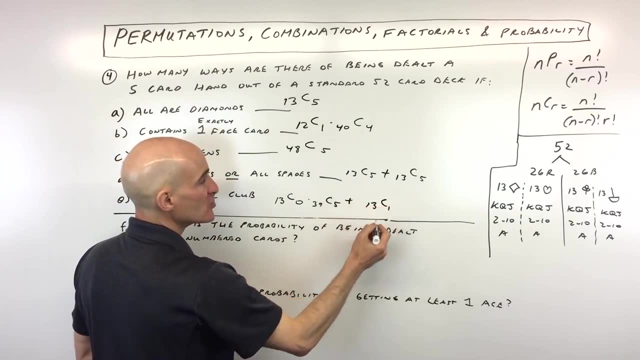 to get five right. 13, choose zero is just one, So I could have just written 39, choose five Plus what's the number of ways of getting one club? Well, out of the 13 clubs we're choosing, 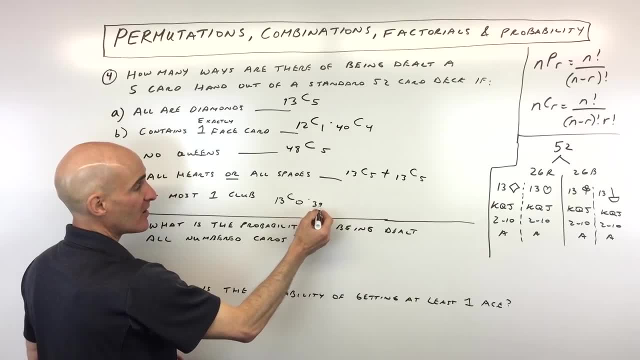 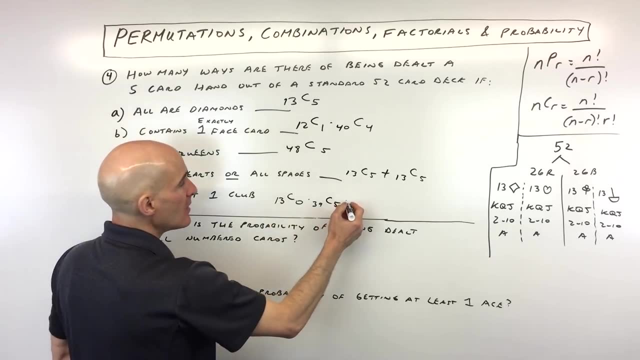 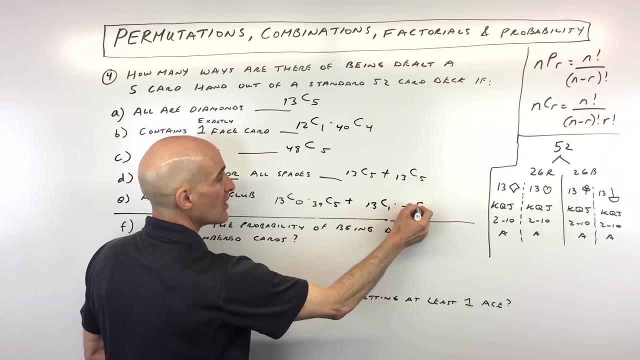 zero. but out of the 39 remaining cards that are not clubs, you're going to get five, right 13,. choose zero is just one, So I could have just written 39, choose five Plus what's the number of ways of getting one club? Well, out of the 13 clubs, we're choosing one and the 39 non-clubs. 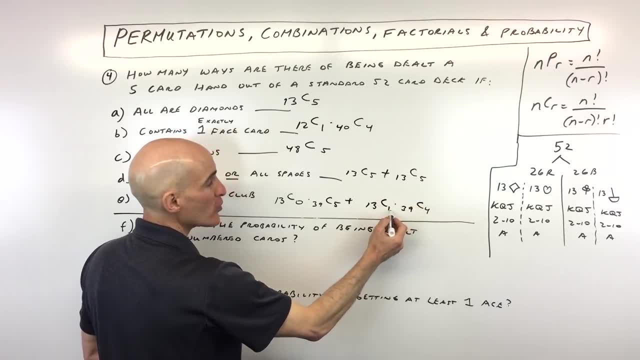 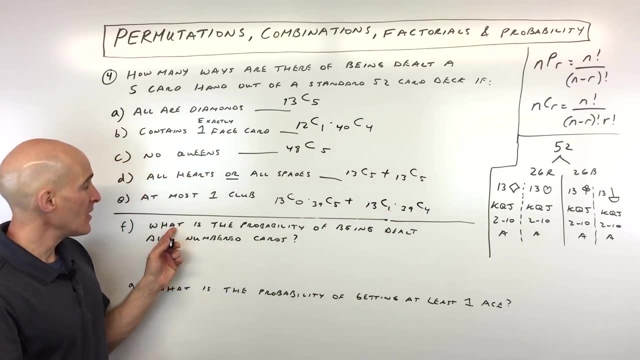 one and the 39 non-clubs. we're choosing four, Notice. the one and the four add up to our five card hand. The 13 and 39 add up to 52.. Let's transition into probability now. Same standard deck of cards, but we're going to get five. So we're going to get five. So we're going to get five. 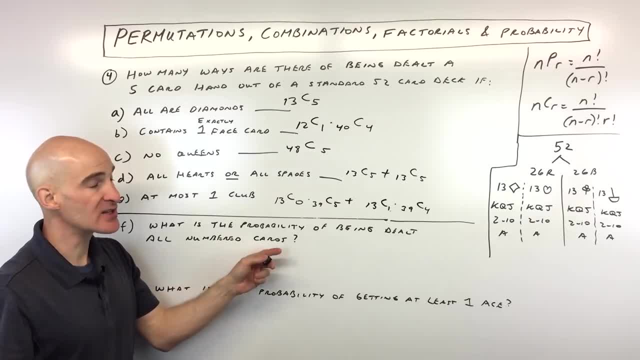 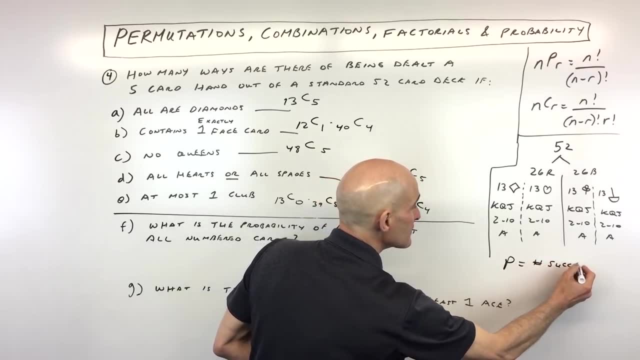 What is the probability of being dealt all numbered cards? Now a quick review of probability. Probability is defined as what? The number of successful outcomes. So I'm just going to write the number of successes divided by the total possible outcomes. Okay, so another way to think. 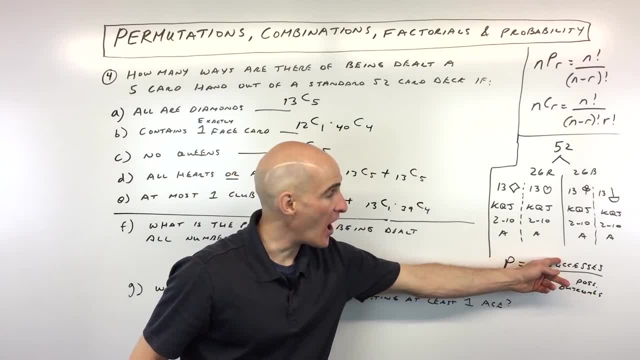 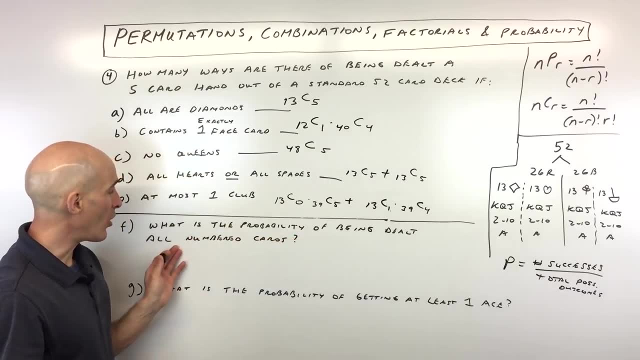 about it very simplistically is: how many ways can you get what you want out of the total things that could occur? So it's the number of successes over the total possible right? So what is the probability of being dealt all numbered cards? Well, you can see, the numbered cards are two. 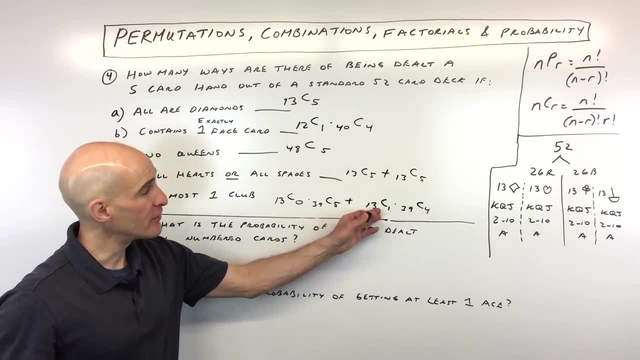 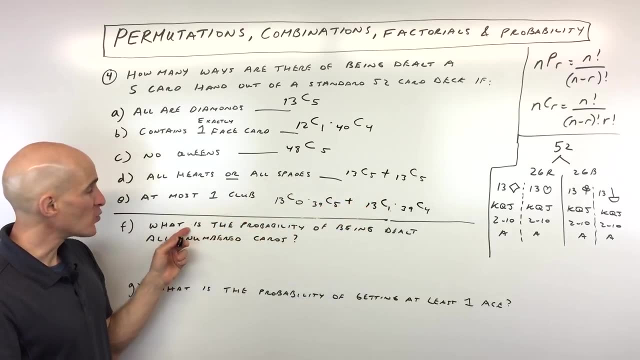 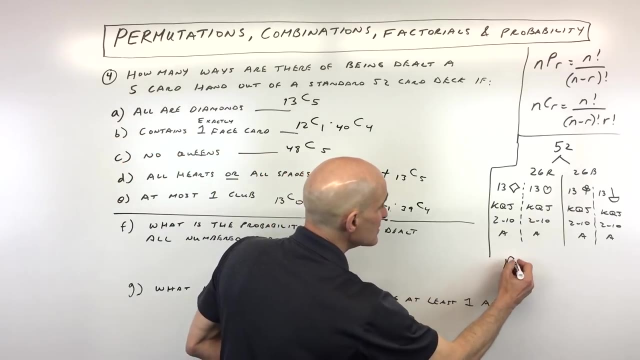 we're choosing four. Notice the one and the four add up to our five card hand. The 13 and 39 add up to 52.. Let's transition into probability now. Same standard deck of cards. What is the probability dealt all numbered cards. Now a quick review of probability. Probability is, you know, defined as: 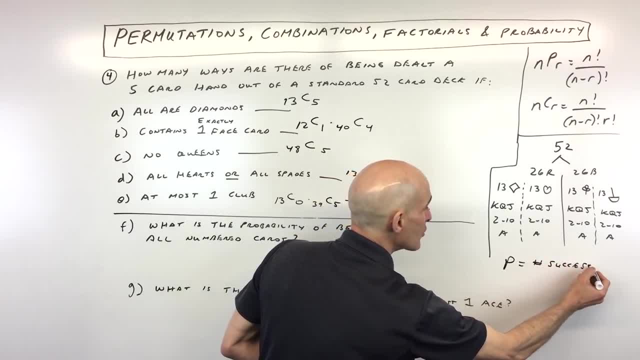 what? The number of successful outcomes. So I'm just going to write the number of successes divided by the total possible outcomes. Okay, So another way to think about it very simplistically is: it's: you know, how many ways can you get what you want out of the total things that could occur? 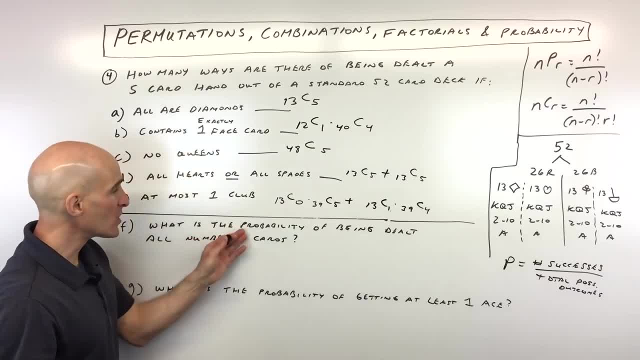 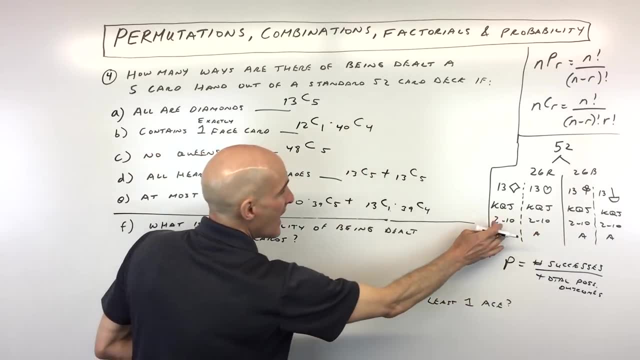 So it's the number of successes over the total possible right. So what is the probability of being dealt all numbered cards? Well, you can see, the numbered cards are two through 10, two through 10, two through 10.. There's nine numbered cards in each suit. Nine times four is 36. And we're going to choose. 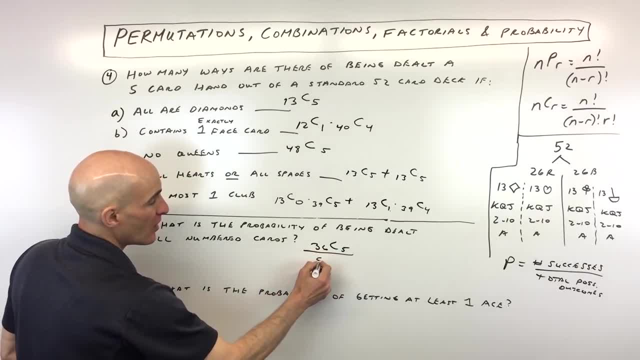 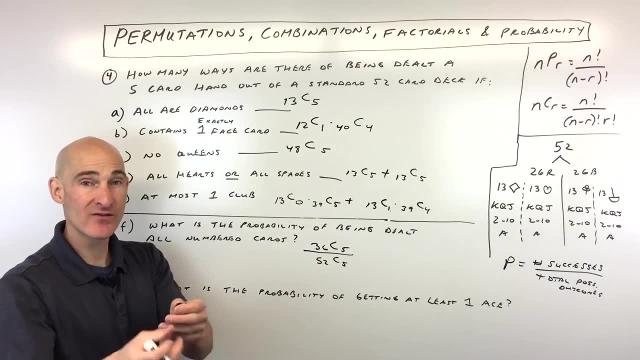 five of those. But in a 52 card deck, how many ways could you be dealt? a five card hand, That's going to be 52, choose five. So out of 52 cards, how many ways of their of you know being dealt? 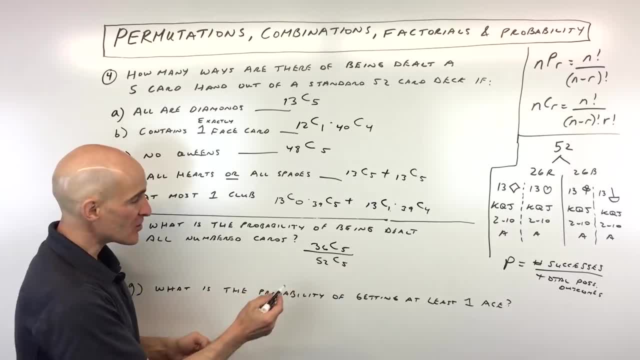 five cards. the order is not important, So we're using combinations again, But our successes are the 36 numbered cards. We want to choose five out of them. So number of successes divided by the total that's going to give you your probability, And this one. 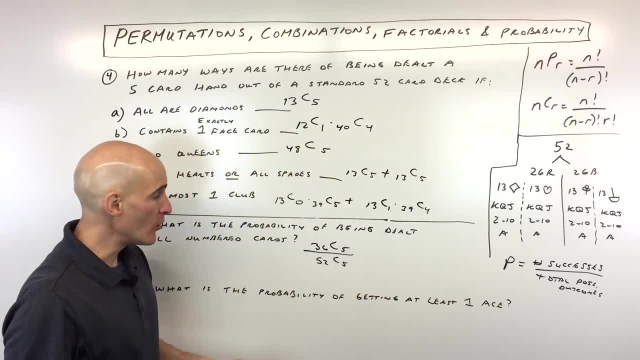 what is the probability of getting at least one ace? Okay, so probably getting at least one ace means that you could have, excuse me, one ace, two ace, three ace, four aces or five aces. right, That's a lot of. you know calculation, So let's go about it a slightly different way. Let's figure: 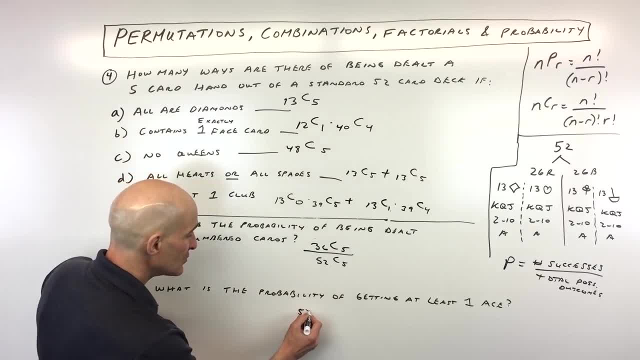 out all of the five card hands, That's 52, choose five minus the ones that have no aces. So when we do this one, do the total minus none. So in this case, the ones that have no aces. that would be 48. 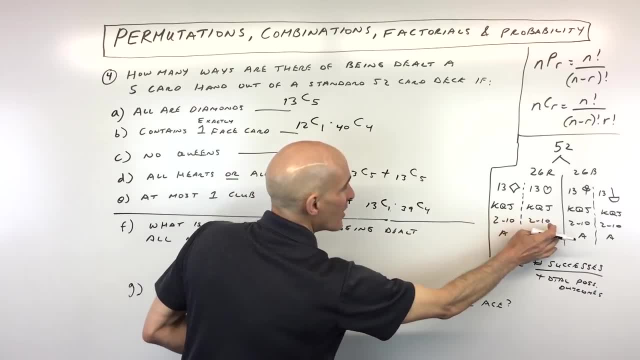 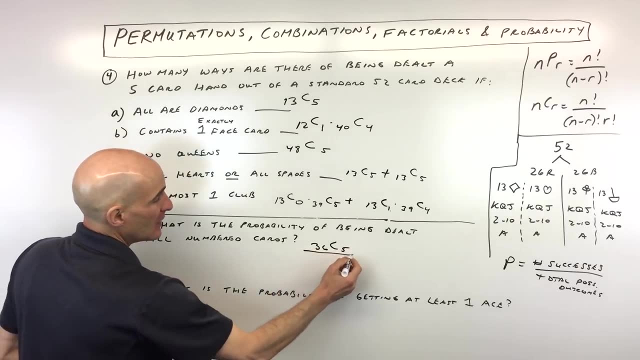 through 10, two through 10, two through 10.. There's nine numbered cards in each suit. Nine times four is 36, and we're going to choose five of those. But in a 52 card deck, how many ways could you be? 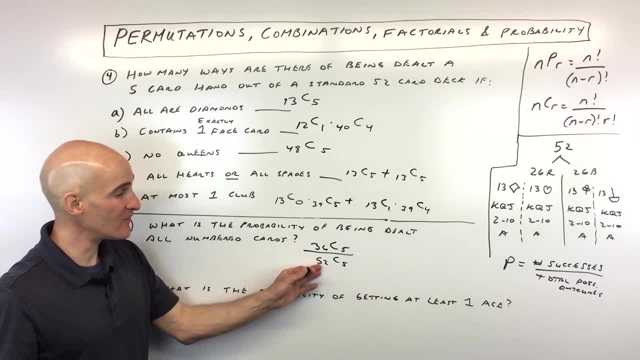 dealt a five card hand. That's going to be 52, choose five. So out of 52 cards, how many ways of being dealt five cards? The order is not important, so we're using combinations again, But our successes are the 36 numbered cards. 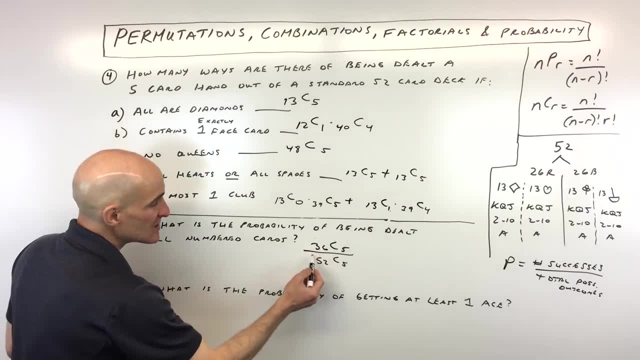 we want to choose five out of those. So number of successes divided by the total that's going to give you your probability, And this one: what is the probability of getting at least one ace? Okay, so probability of getting at least one ace means that you could have, excuse me, one ace. 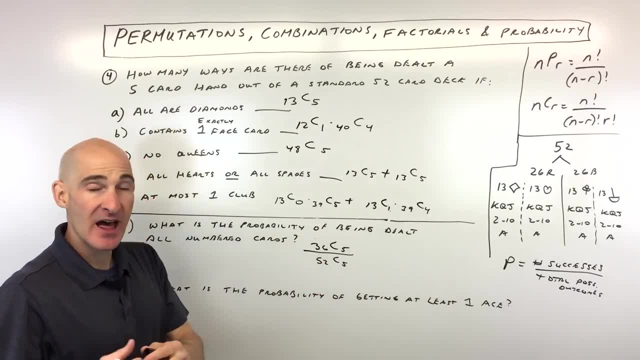 two ace, three ace, four aces or five aces. right, That's a lot of. you know calculations, So let's go about it a slightly different way. Let's figure out all of the five card hands, that's 52, choose. 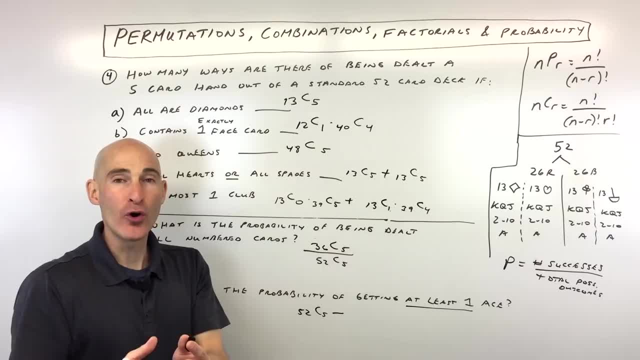 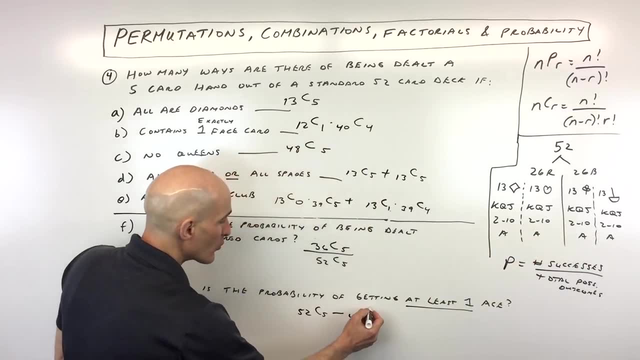 no aces. So when you see at least one, do the total minus none. So in this case, the ones that have no aces, that would be 48 cards that are not aces, because there's just four aces and we're. 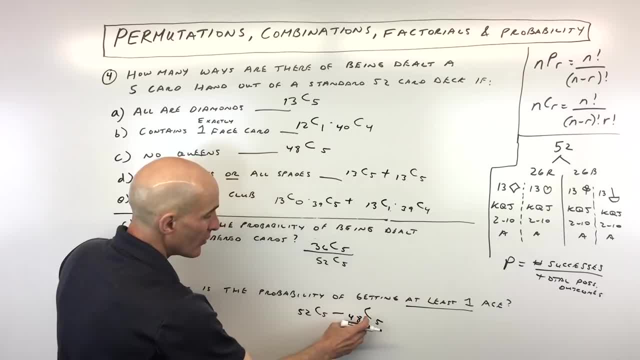 choosing five. okay, So this would be all the cards that the five card hands that have at least one or more ace in it, because this is the ones that have none. So total minus none divided by how many ways can you be dealt a five card hand out of 52 cards? That's 52, choose five, If you simplify. 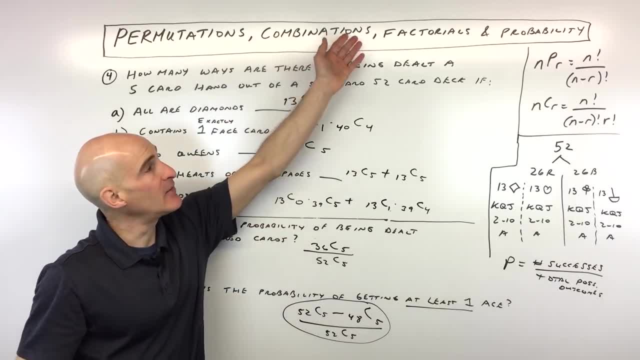 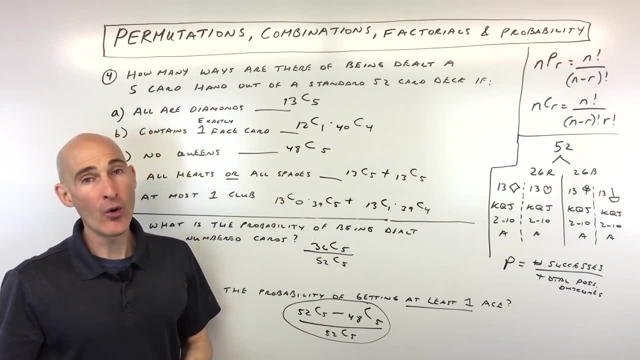 that you get a five card hand out of 52.. If you have some additional questions about permutations, combinations, factorials, probability, I'll put links to some other videos I did in the description of this video. Or another option is go ahead and put your question in the comments below and see. 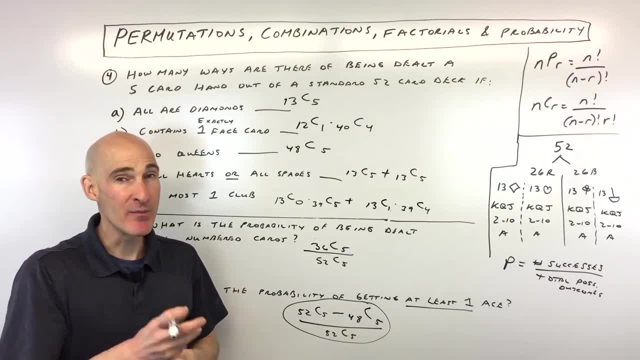 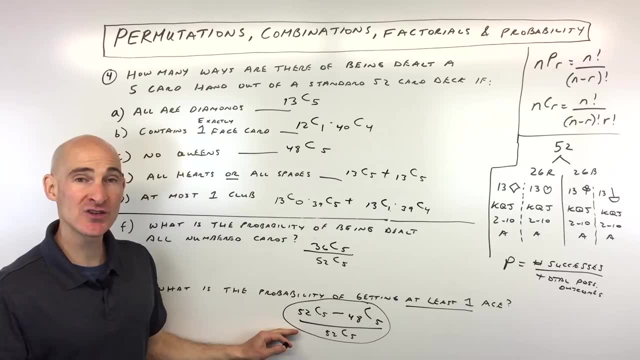 if you can help one another answering some of those questions. So test yourself, you know, by maybe posing a question and also by trying to answer some other students questions as well. You'll learn a lot from that. Also, check out my other videos, like I said, about permutations, combinations. 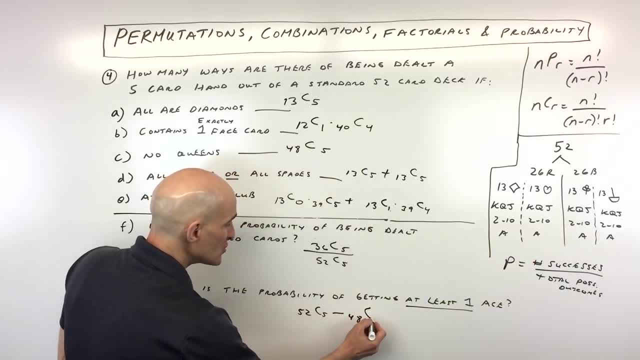 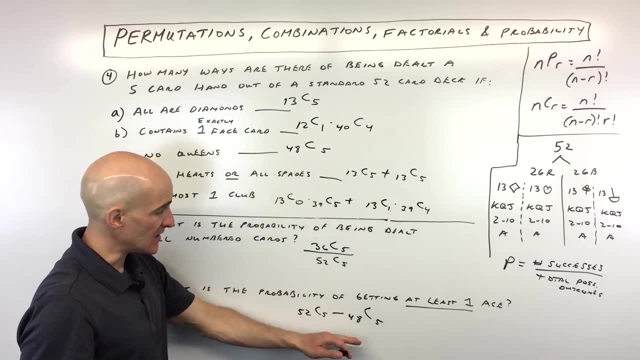 cards that are not aces, because there's just four aces and we're choosing five. Okay, so this would be all the cards that the five card hands that have at least one or more ace in it, because this is the ones that have none. So, total minus none divided by how many ways can you be dealt a five? 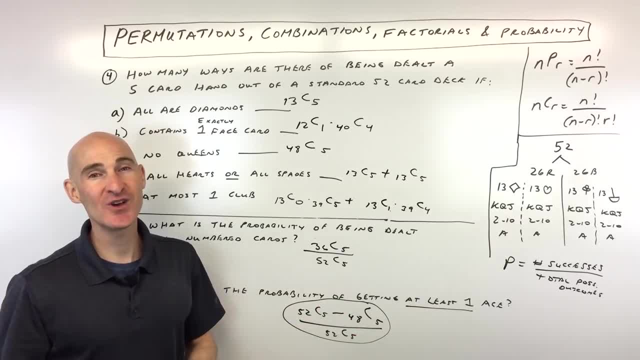 and probability. Otherwise, subscribe to the channel and I look forward to seeing you in the future videos. I'll talk to you soon. 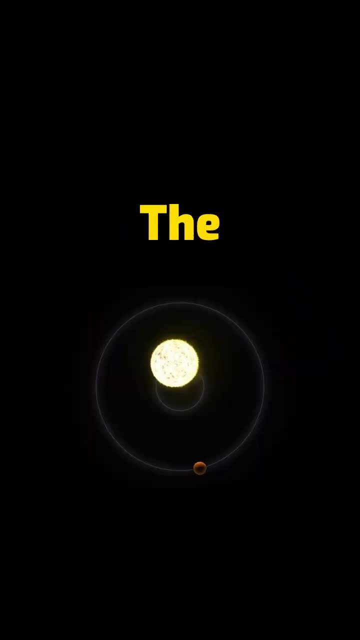 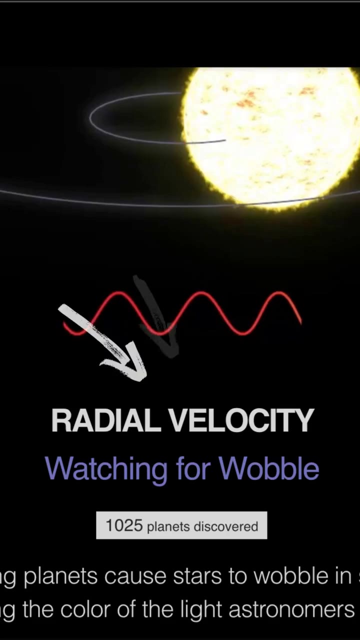 Gravitational interaction between a planet and a star causes the star to wobble in space. This phenomenon changes the color of light, called redshift. By using this data, astronomers use radial velocity method to confirm exoplanets. So far, we found 1,025 planets with